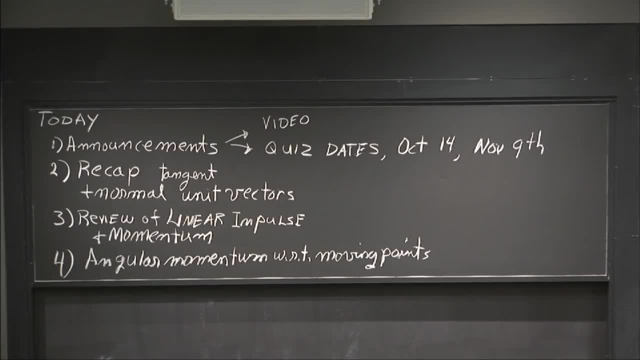 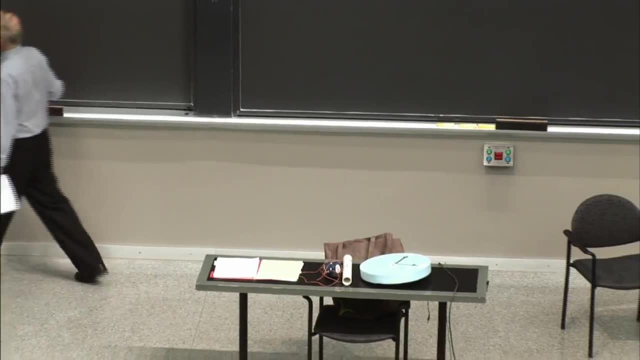 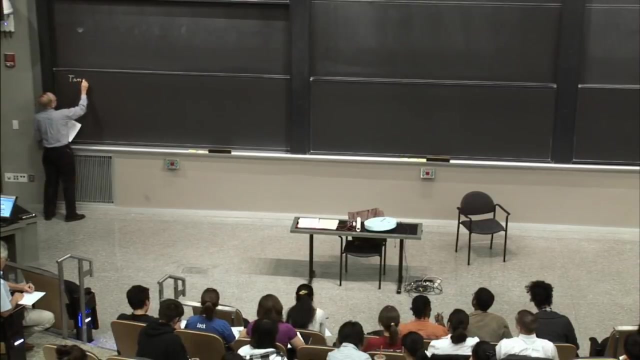 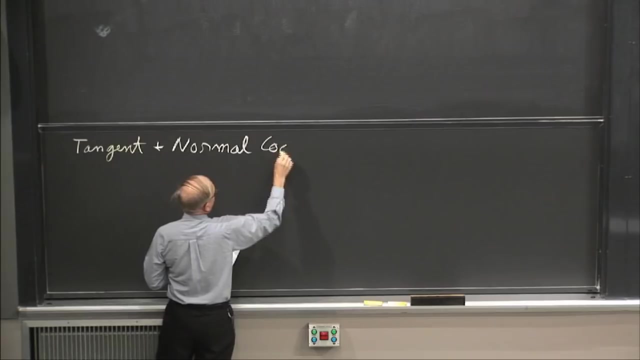 with respect to moving points, which you probably haven't encountered before. So those are the three topics for today. Let's get started. So last time, the piece that I rushed a bit is this notion of tangent and normal coordinates, So I had this example. 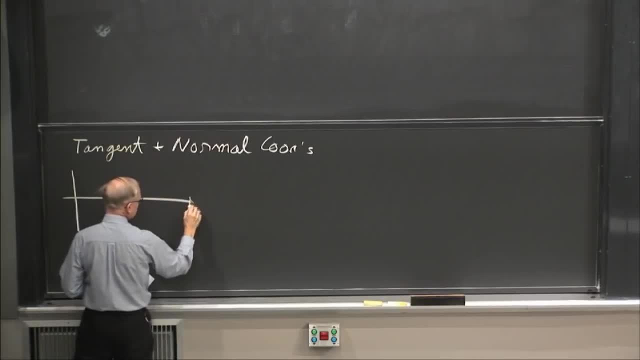 You're driving down the road, You're drunk or whatever, And when you're at this point, this point and this point, I'd like to know what the accelerations are. So I'll call these 1,, 2,, 3.. 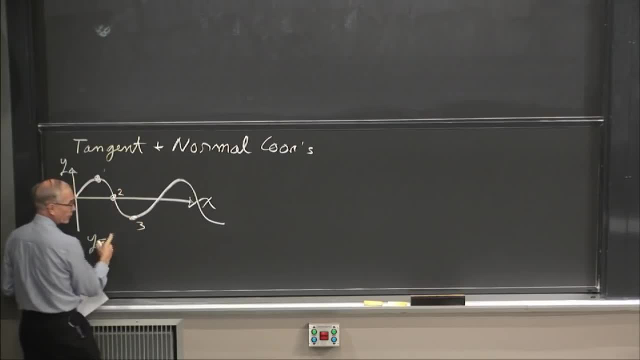 And this curve, y is of the form, some y of some f of x, And in this case it's a sine k. x And k is what's known as wave number is 2 pi over the wavelength, 2 pi over lambda. 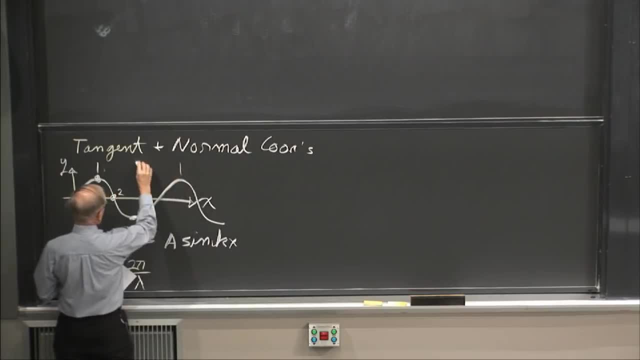 And the wavelength then is, for example, from here to here. Now the velocity- I'm going to pick a point here- The velocity at any point, we know, is just the tangent to the path. So this is the path and this is horizontal. 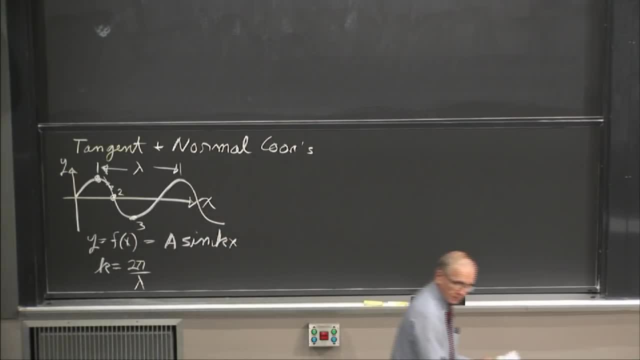 So you're driving down the road like this. That's what we're trying to do here. The gravity is down into the board. It doesn't really come into the problem. So the velocity, at any time the vector we could describe as a magnitude. 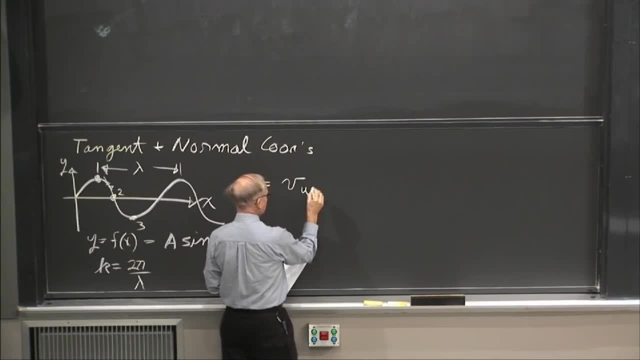 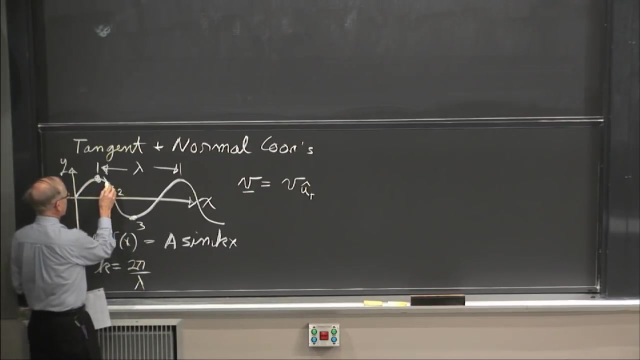 And a unit vector we'll call ut, which is the tangent unit vector And at any instant in time it's just aligned with the tangent to the curve And its perpendicular partner is a normal unit vector which it points inward on the curve. 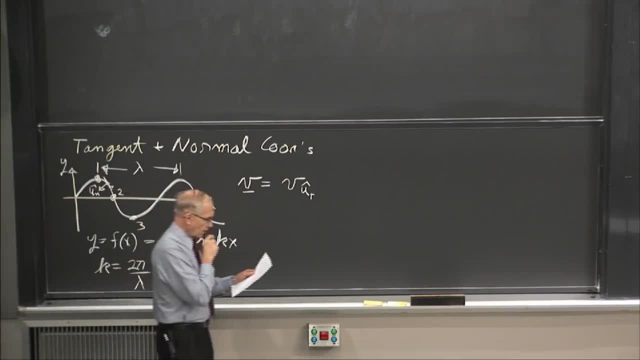 And this would be un. Now we're interested in accelerations, so we'll need to take a derivative of this. So let's back up. OK, All right, I was going to say take it aside, but I won't. So the acceleration vector we have. 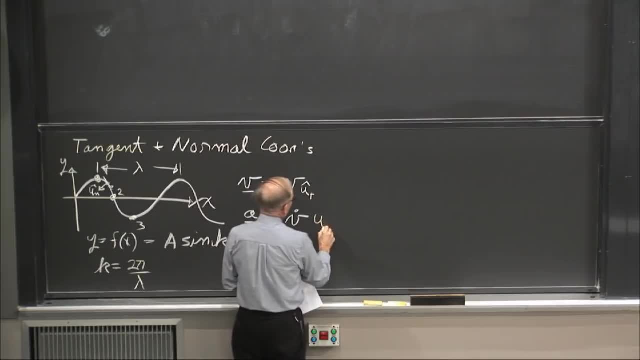 to take the derivative of this, Well, it's a v dot ut plus a v ut dot. It's a unit vector And we've encountered this problem before because if this rotates, the unit vector has a non-zero derivative because of its rotation. 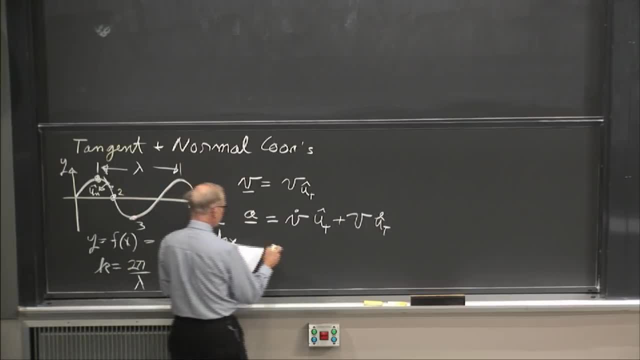 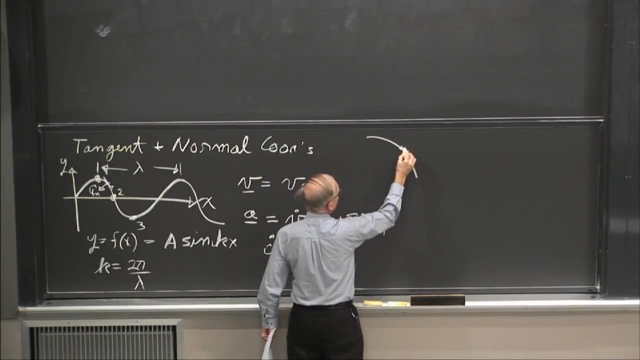 And this derivative of the unit vector is given by theta dot un hat. Now, what's theta dot? Well, on this curve, at any instant in time, here's? u Can't draw arrows today. Here's your ut. At any instant when you're traveling along on a curve. 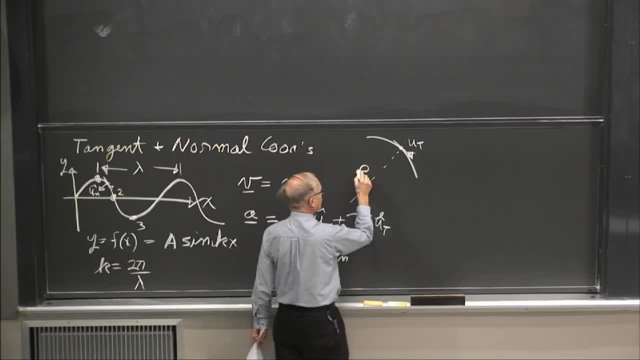 you are going around a circle of some radius, we'll call rho. So there's some radius of curvature at any instant in time And that radius as you drive along. in a little time, delta t, you go forward an amount, rho, theta dot. 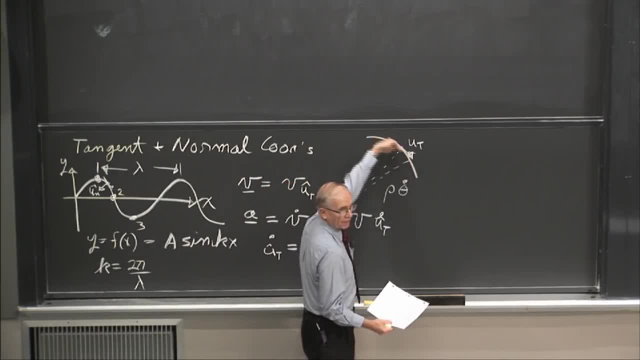 is the Velocity at which you're traveling tangent to the curve. There's an angle in here. So in here there's some delta. You advance some delta theta. So r omega is a velocity. right So rho, theta dot is a velocity. 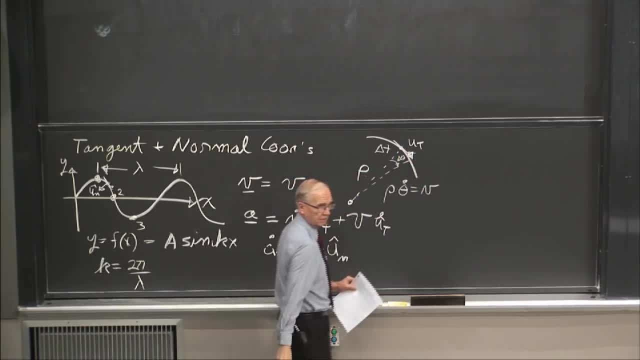 And that gives you this velocity, magnitude v, And we've gone through. I'm not going to go through that little derivative. I've done that little argument before. But the change in direction of this unit, vector ut, when you go forward a little bit, is actually inward un. 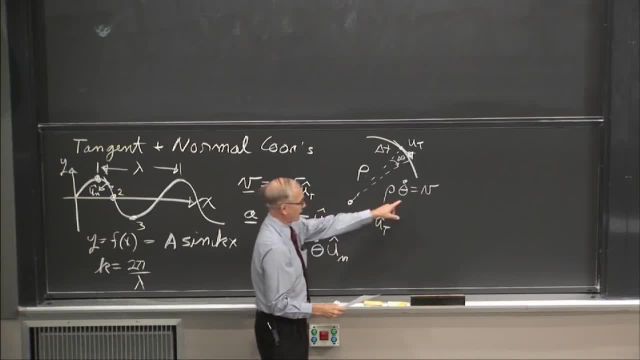 by an amount: theta dot 1 times theta dot. So I'm not going to do that piece of the derivative before. But here is this derivative of the unit vector. It's theta dot- un. So if we substitute those back in here, 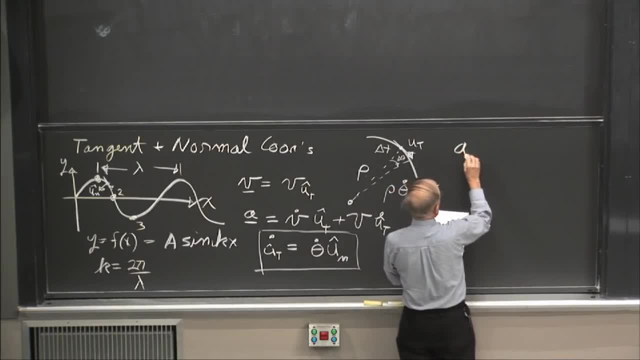 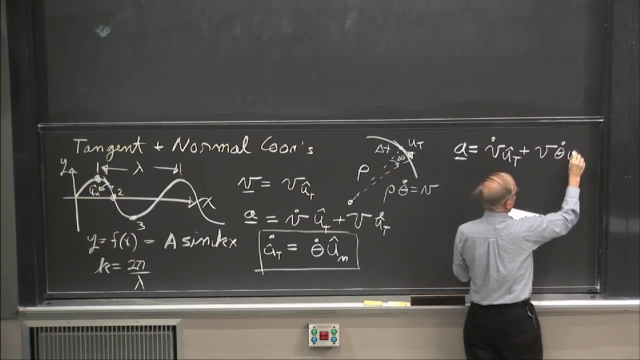 we can get an expression for our acceleration. This is just the acceleration along the path, plus v, theta, dot, un. And then we need to take into account the fact that we know that v Yeah The magnitude of the line, The velocity. 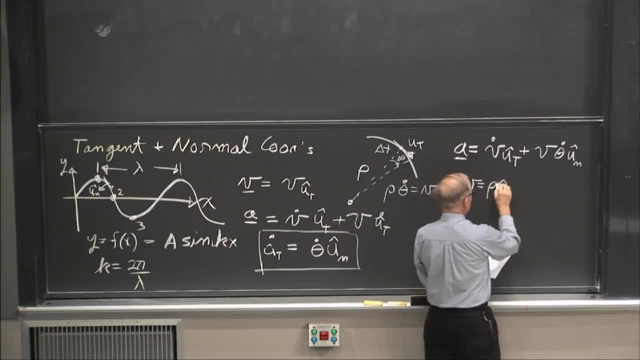 The speed. in other words is rho, theta dot, And that means theta dot is v over rho. So if we plug that in up here, then we get a final expression for our acceleration: v dot ut plus v squared over rho un. 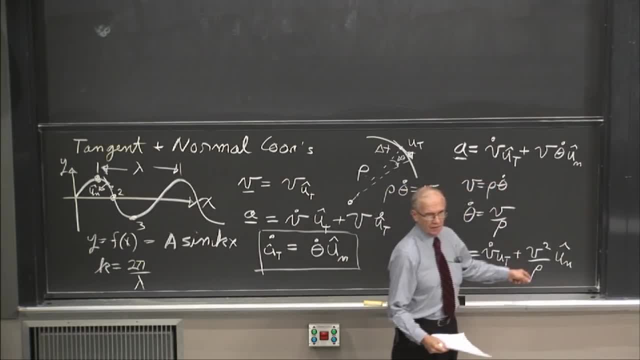 And that v squared over rho. this is a centripetal acceleration term. You're going around a curve, There's an acceleration inward. It's just like as we did from polar coordinates. It comes from rotating things. Well, as soon as you go around a curve, 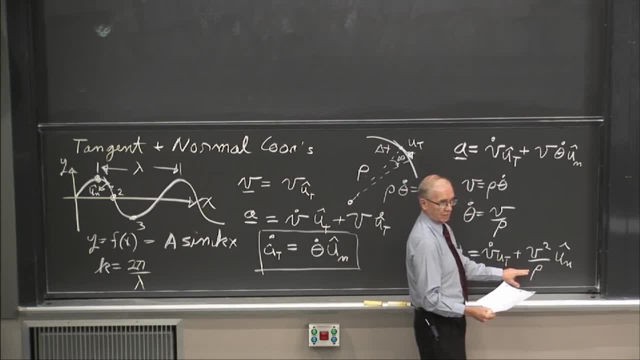 you're going to generate an acceleration that is of the same kind, But now, because you tend to know speed, it's easier to express it this way when you're doing these tangent normal problems. And this is just the acceleration along the path. 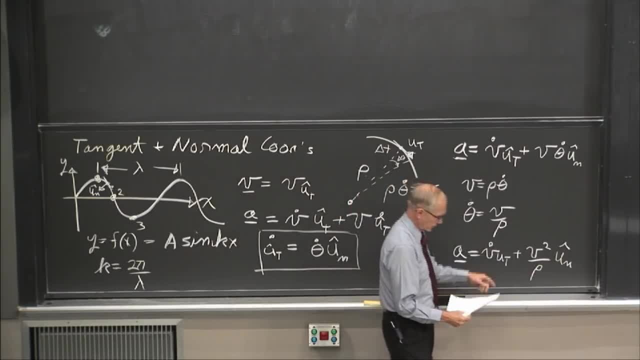 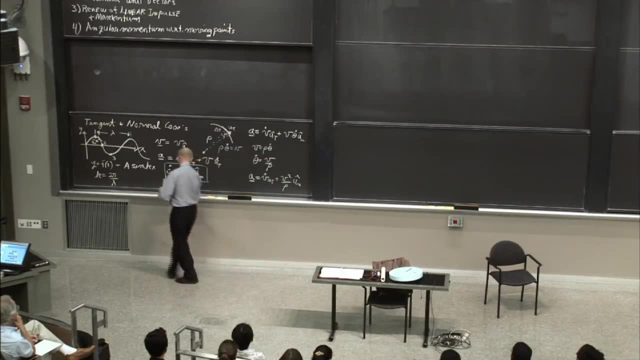 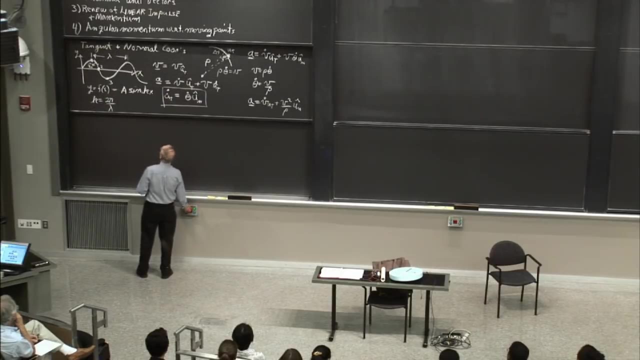 The usual: hit the gas pedal and speed up. That's this term, OK, So the piece that I didn't have time to put up last time, which is in the book, as is this little derivative, the derivation of that. It's one page in one of the books. 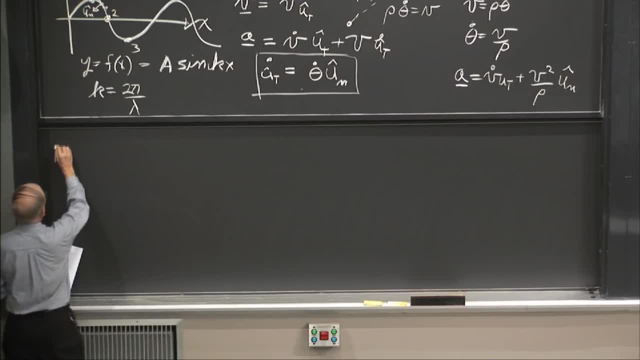 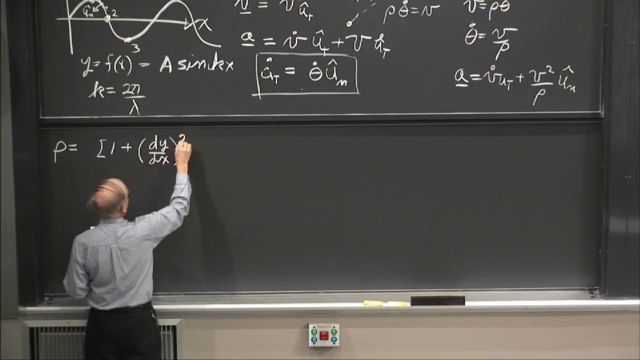 OK, One of the early chapters of the book. How do you get rho And rho when you have y as a function of x? there's just this formula from mathematics, from calculus, that says rho is dy dx, 1 plus dy dx. 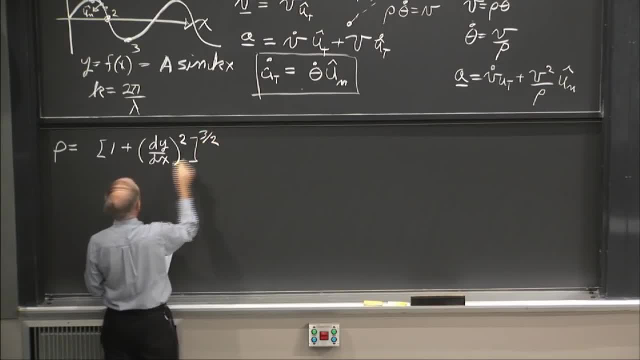 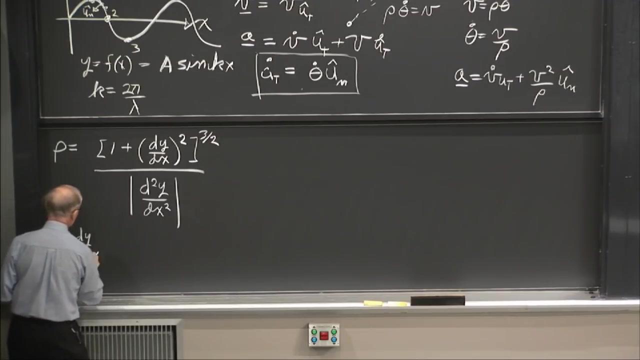 quantity squared to the 3 halves power, all over the magnitude of d2y dx squared, And you just calculate these quantities and plug them in. So for y equals a sine kx, then dy dx is ak cosine kx And d2y dx squared is minus ak cosine kx. 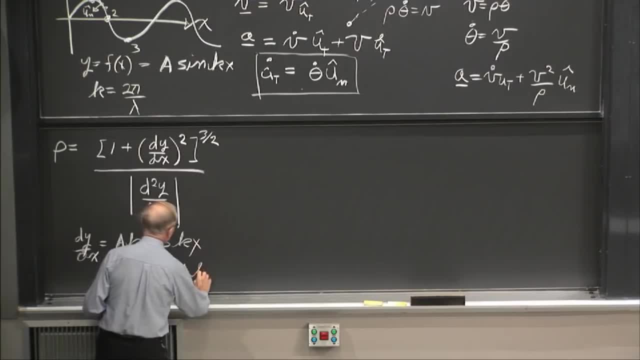 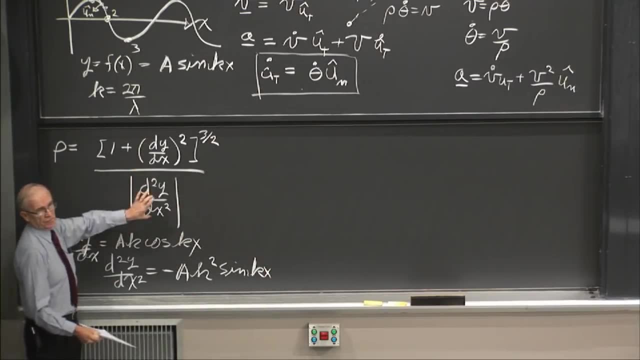 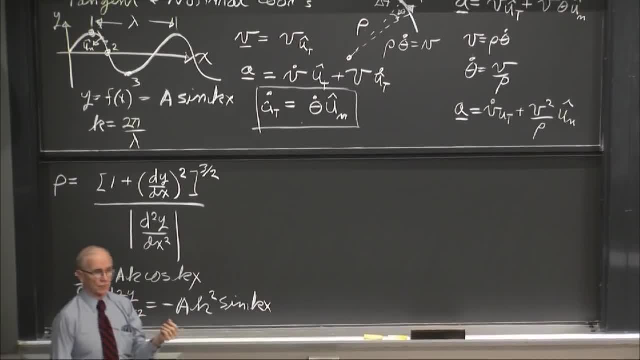 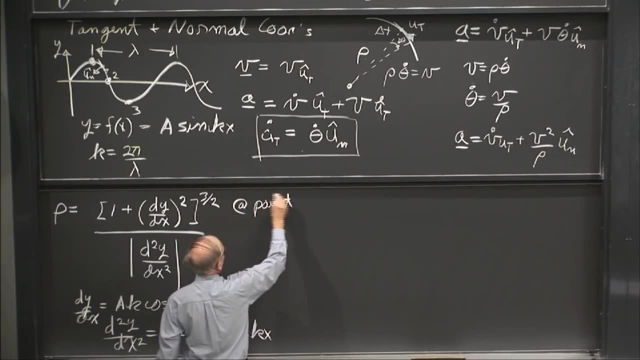 So at 0.1 kx is pi over 2.. Right, Because sine is a maximum, x is lambda over 4. kx x is pi over 2, sine kx is 1, cosine kx is 0.. 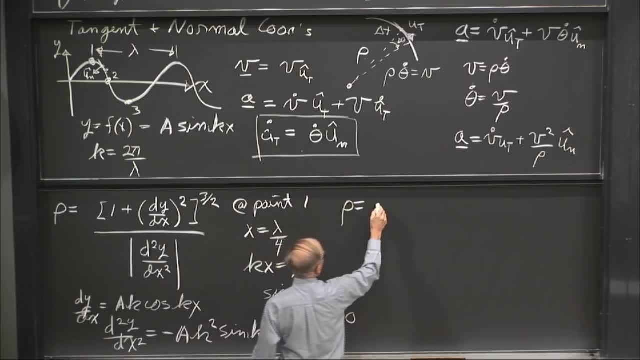 And so we can calculate rho 1 plus and dy dx. The derivative is cosine, That's 0. So this term in here is 0. This is to the 3 halves. That's pretty easy to calculate This term down here. dy dy dx squared. 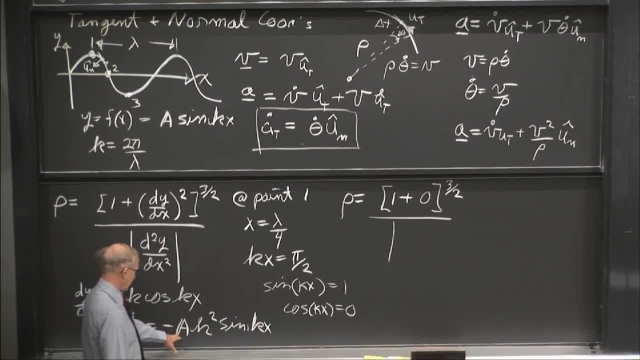 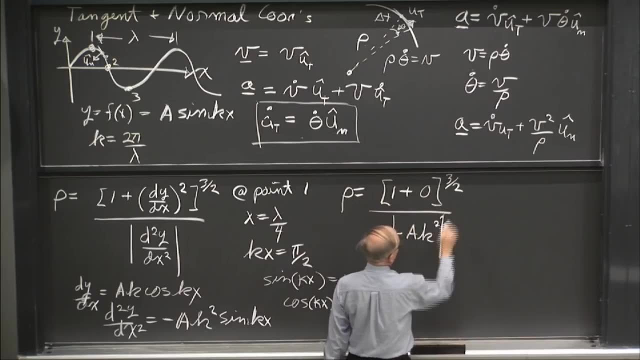 Well, sine of kx is 1.. So that's minus ak squared, But this is an absolute value sign. This just turns out to be 1 over ak squared And we plug in some numbers. I'm going to let my lambda be 150 meters. 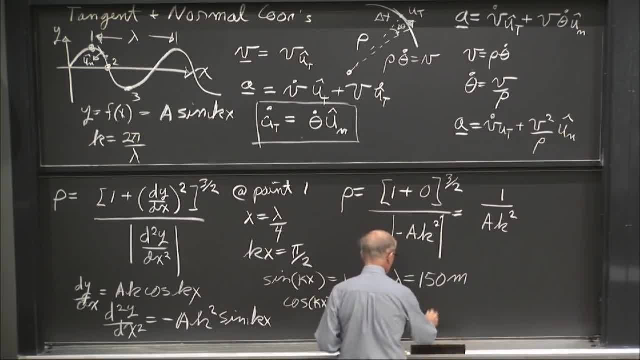 My amplitude here, that I'm swerving back and forth. let's make that 5 meters. That's all we need to get rho. So rho in this case works out to be 100.. And 14 meters, So the radius of curvature of this road. 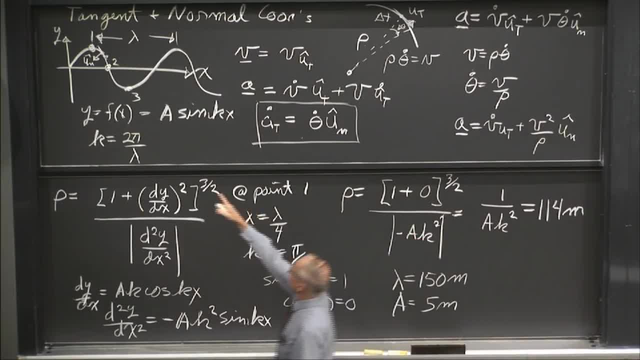 that I'm driving down at that point, right at the peak in the curve, is 114 meters. So the acceleration that I'm looking for a well, it's v dot ut, And if I'm not accelerating I'm not hitting the gas pedal. 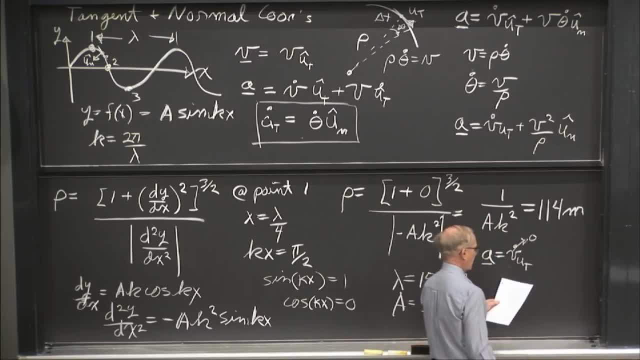 constant speed. I'll let that one be 0. 0. 0.. And the other one then is v squared over rho in the un direction, And let's let v equal. I have here in my example 20 meters per second, which is about 40 knots. 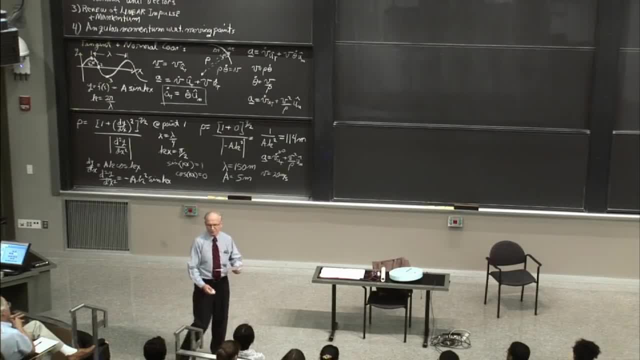 And a knot is 15% more than a mile per hour. So it's somewhere about 45 miles an hour. So a typical road speed driving down the road, 20 meters per second. Now you can plug in here. You can plug in here. 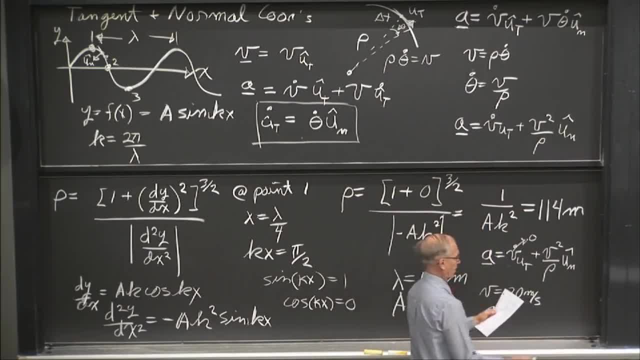 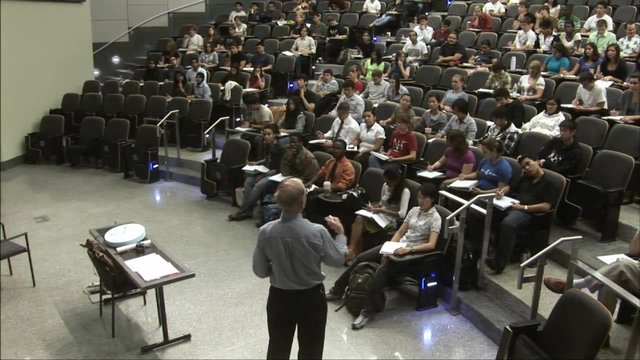 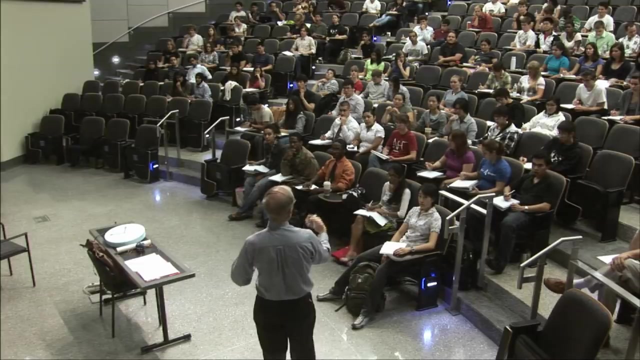 And you can find that the acceleration that I work out here is 3.51 meters per second squared. And in what direction is it? What direction is that acceleration? It's in the normal direction. It's in the normal direction. Is it to the inside of the curve or the outside of the curve? 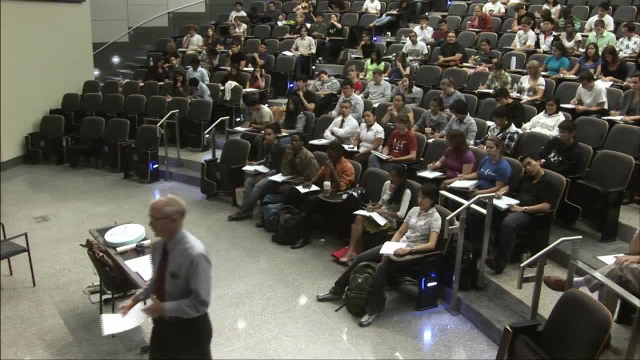 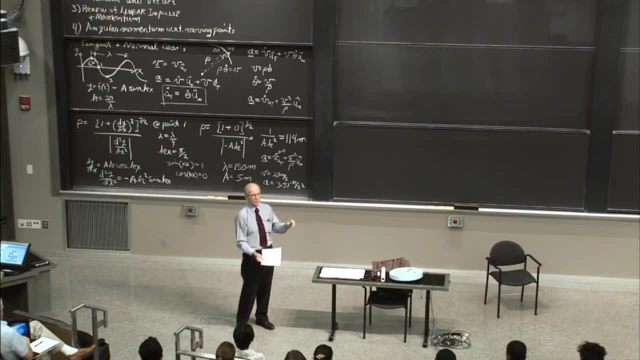 Inside, always to the inside of the curve. So these tangent normal coordinates are really simple coordinates. They're meant for a particular kind of simple problem when you know the path And it's just defined. The normal un is positive, always inward to the center of the curve, pointing. 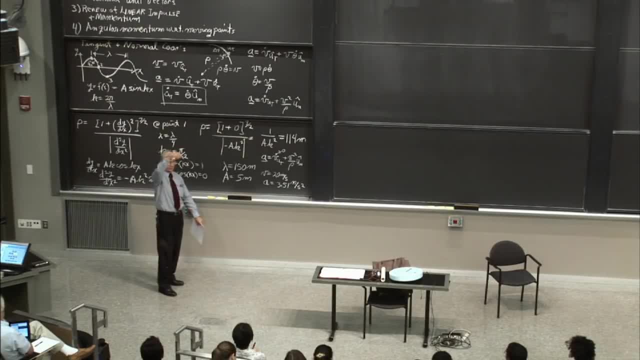 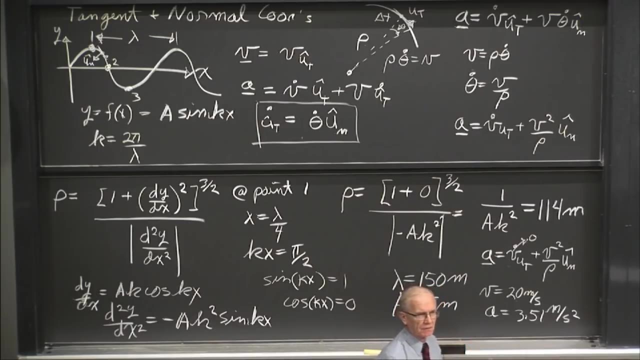 toward the center of rotation, where your radius of curve is always pointing at the origin of that radius of your curve. So g is the order of 10 meters per second squared, So that's about a third of a g. Would you do a third of a g enough to notice? 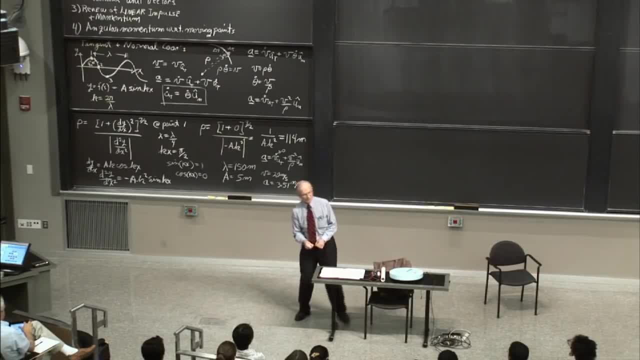 Yeah, absolutely, You'd get pushed to the side of the car. if you do that, Any questions about that? I'm going to move on next. If not, I'm going to move on to linear impulse and momentum. And this will be a quick review, because this 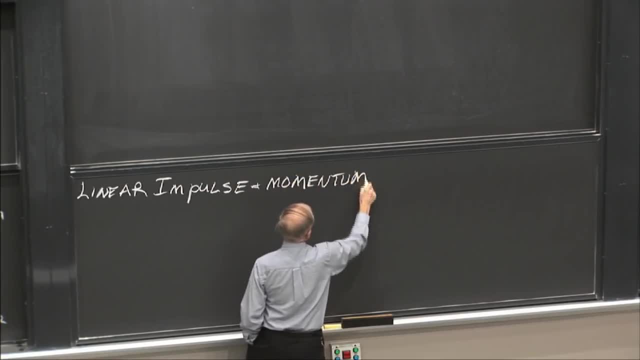 consists of the physics, the kind of physics that you've done lots of times. So we're going to hit it quickly and then move on to angular momentum. So we know for a particle. this is what Newton told us. You've got a particle here. 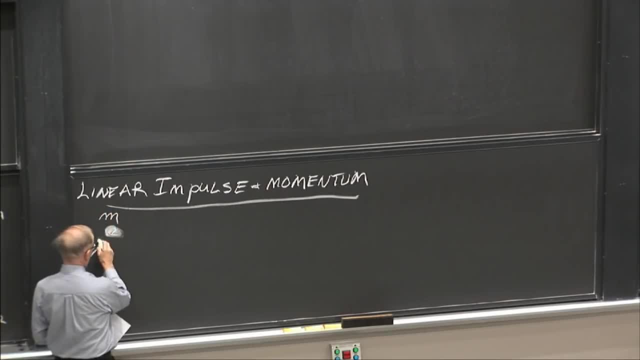 That's some mass m, We know for a part, and it has some external forces on it. we know for a particle that the sum of these external forces- it's a vector sum- is equal to the mass times, the acceleration for the particle, Newton's second law. 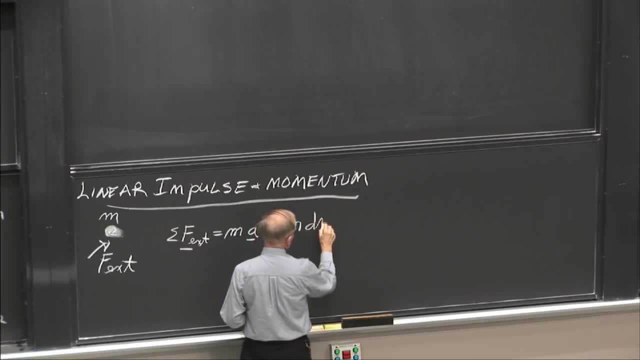 And that's the mass times, the derivative of the volume, That's the velocity with respect to time. That's where we get acceleration. So this formula, we can just rearrange the dt's a little bit. So the summation of the forces dt is mdv. 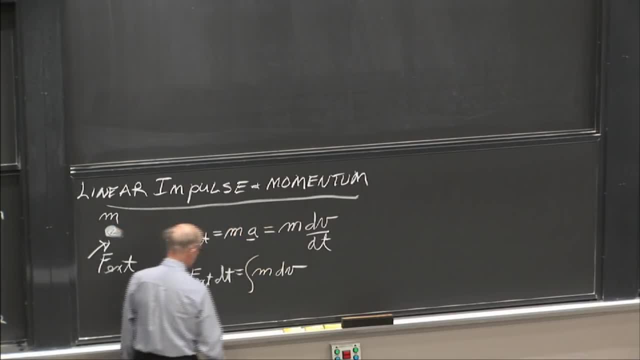 And I want to integrate these. So if I integrate this over time from some t1 to t2, this equality says we're going to find some change in velocity from v1 to v2.. And this is kind of the beginning of our impulse-momentum relationship. 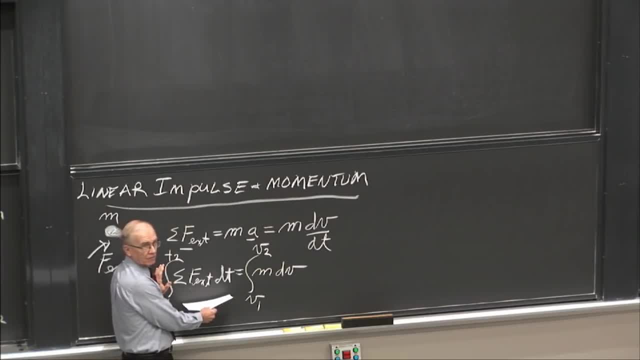 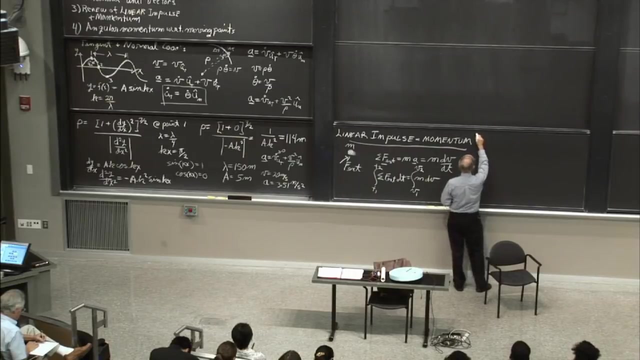 We tend to call the integration of forces over time impulse, And if you have a non-zero impulse, that leads to a change in the linear momentum. So when you carry out- So they're writing this a little bit different way- You can do summation because these are vectors. 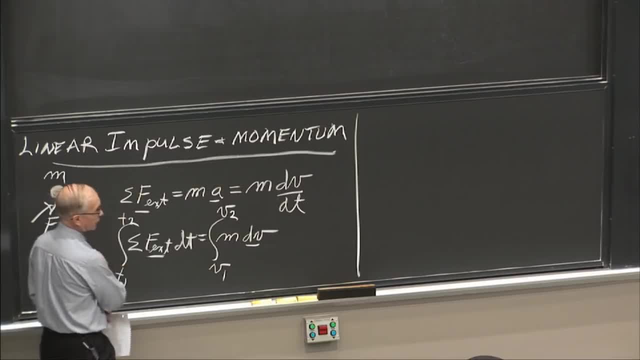 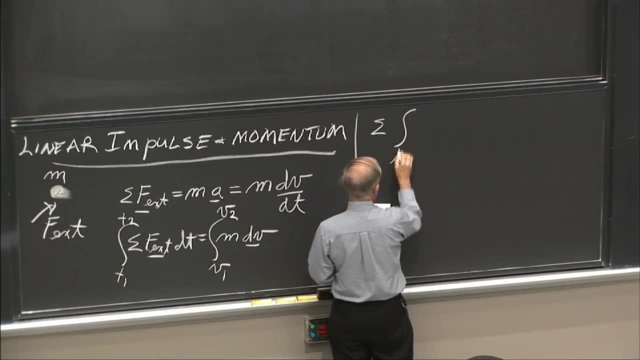 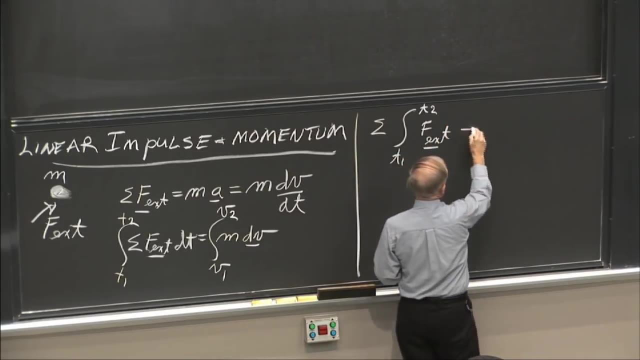 And we have rules about vectors. You can bring the summation outside of the integral. So this says that the summation of the integral from t1 to t2 of these external forces is just mv2 minus mv1.. Because the integral is going to be mv2 minus mv1. 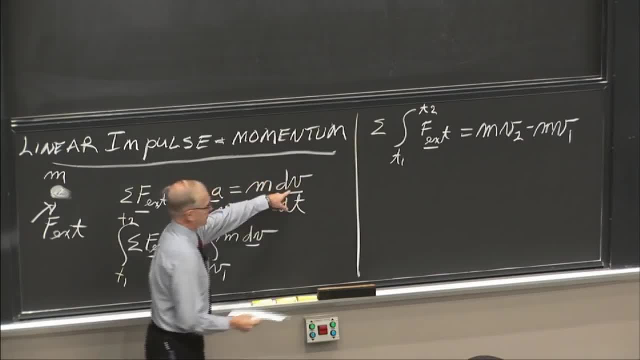 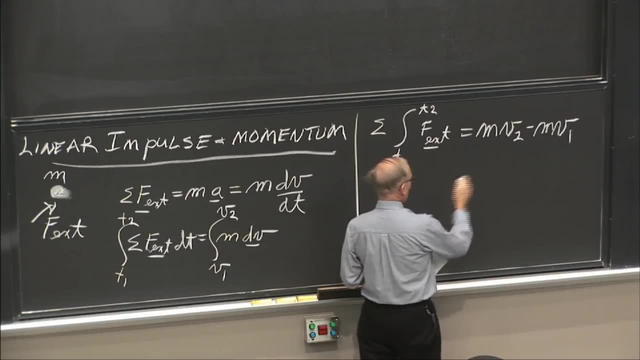 So the integral is going to be mv2 minus mv1.. Because the integral on the right-hand side is really simple And we'll finally state this in a way that we most commonly use it, moving this term to the left. So you start off with an initial momentum, mv1. 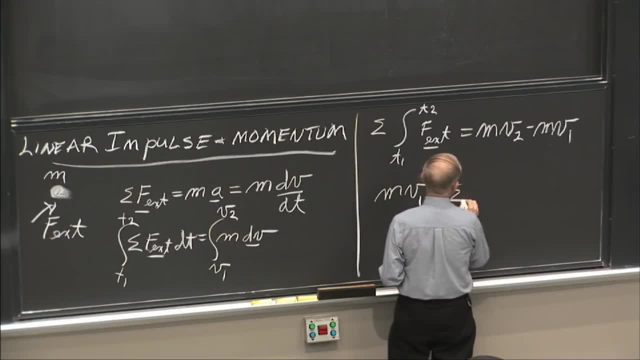 You add to it the summation of the impulses that occur over time: t1 to t2 of the integral. So you start off with an initial momentum: mv1.. You add to it the summation of the impulses that occur over time: t1 to t2 of the integral. 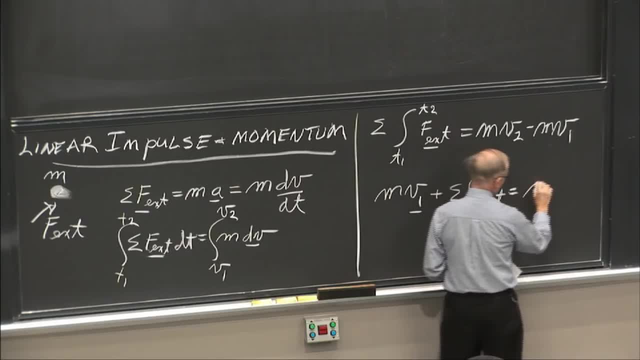 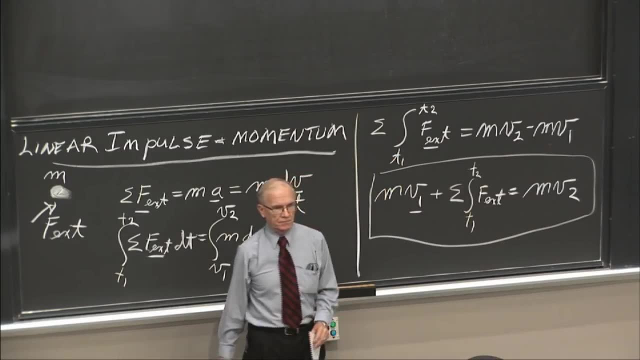 You add to it the summation of the external forces And you get the final momentum, mv2.. And this is the way you usually use the formula. So what happens if there's no external forces? That's where we get the law of conservation of momentum. 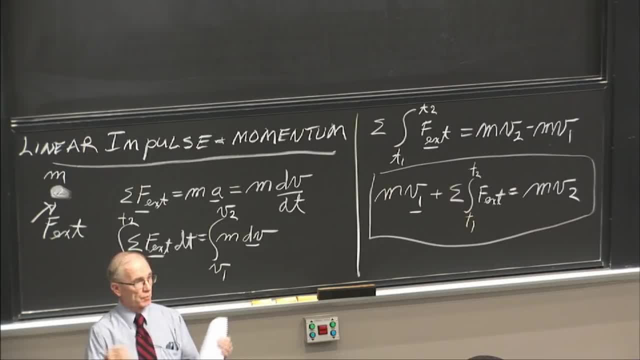 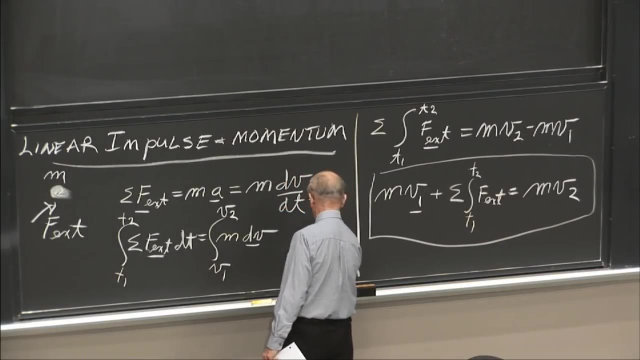 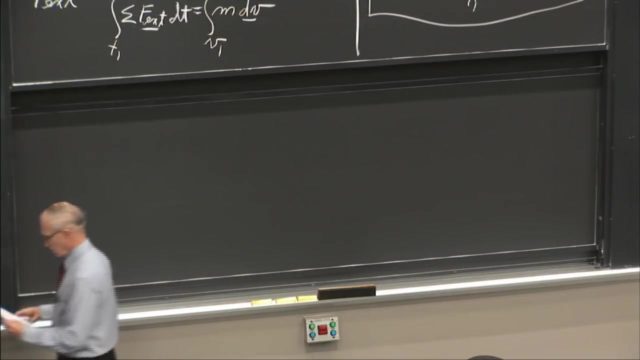 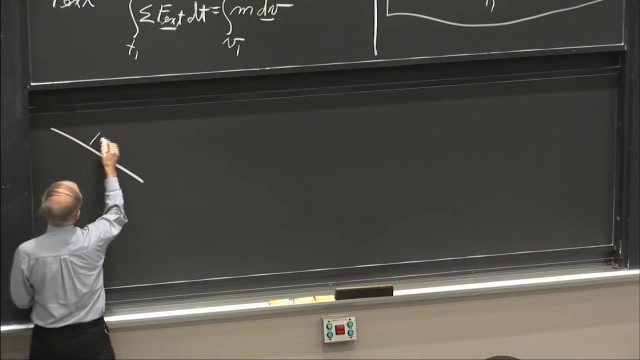 If there are no external forces on the particle, the momentum doesn't change And mv1's got to be equal to mv2.. Oops, So just a really trivial example, drawing for something that we've done before. You have the block sliding down the hill. 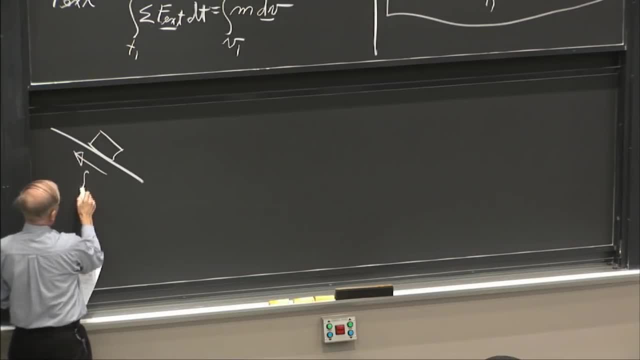 Draw your free body diagram. Friction: We've got gravity, we've got a normal force and we'll set ourselves up with a coordinate system aligned with the motion we're interested in. So this is an inertial system xy, And we've done this problem before. 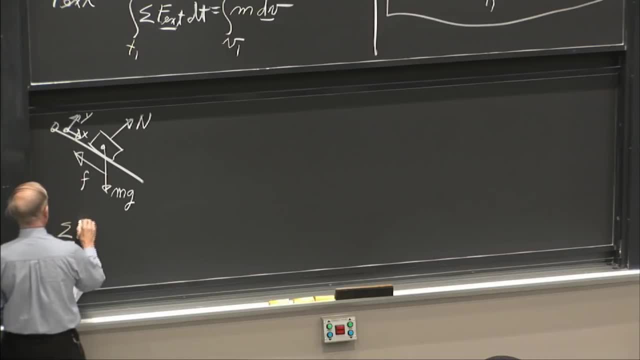 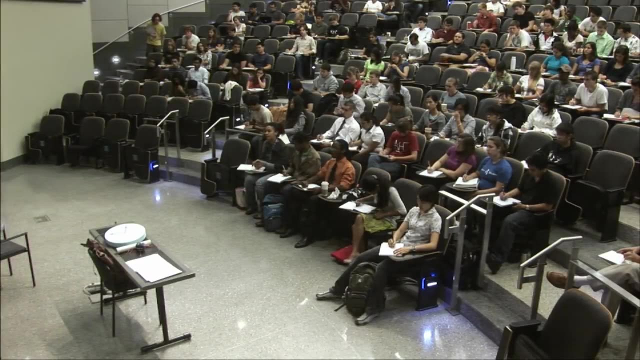 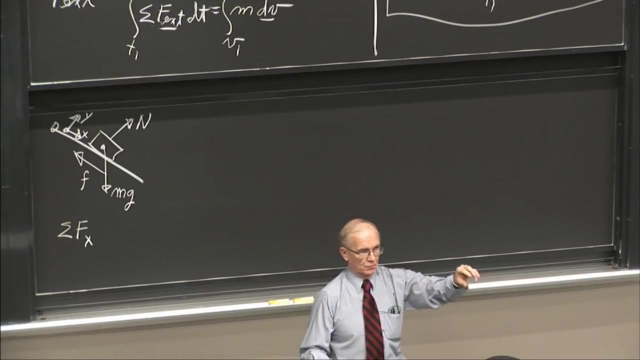 So we said the summation and we found out that the summation of the forces in the x direction- and- ah, this is a good moment to take an aside for a second- This was a vector expression, but you can implement it. You can break it down into its individual vector components. 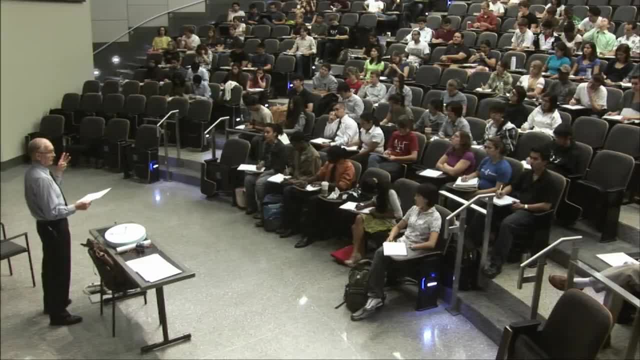 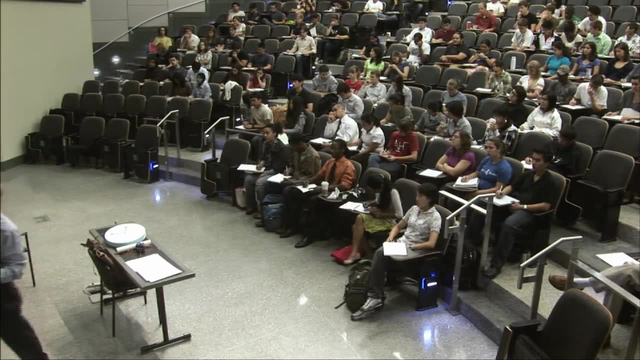 So that equation gives you for particles, gives you three sub-equations, one on the x, one on the y, one on the z, and you can use them each independently. So in this case we're going to only need the x component. 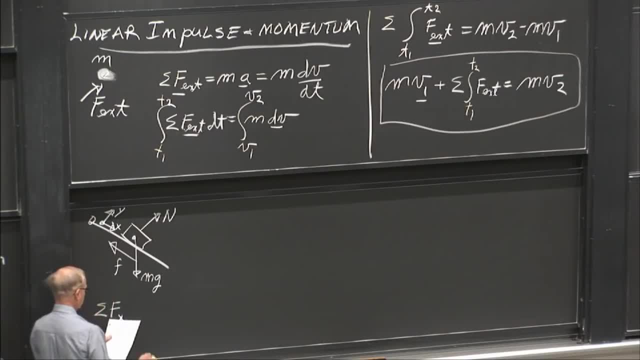 in order to do the problem. So the sum of the forces in the x direction now in this problem, which we have done before, is mg sine theta, that component of gravity pulling it down the hill, minus mu mg cosine theta, And that's the friction. 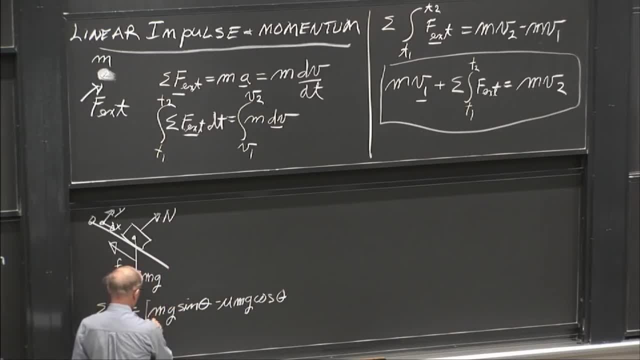 And none of these are functions of time. So that whole thing is just some constant. I'll just call it k. So the total forces on this system in the x direction is just some constant, And that makes this integral up here pretty trivial to implement. 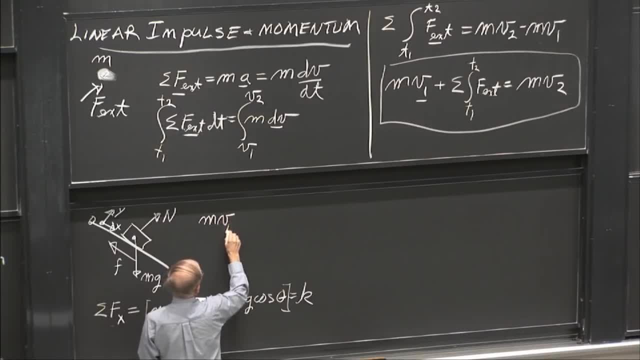 So now we can say that mv1, I'll just make it v1x to emphasize that integral from 0, or t1 to t2, but I'm going to let t1 be 0. Usually makes the problems easier. 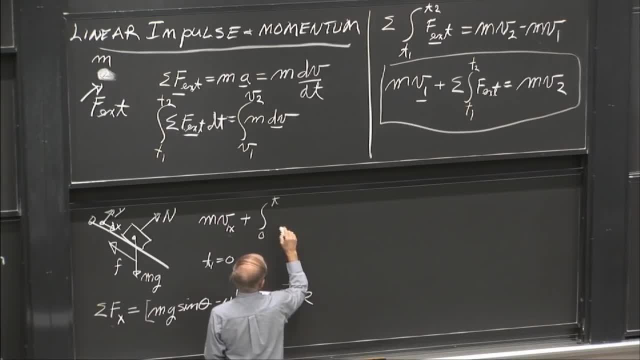 So from 0 to t, 0 to t Of kdt equals mv2.. I can't write this morning In the x direction And if v1x is 0, starts off at 0 time and 0 velocity. 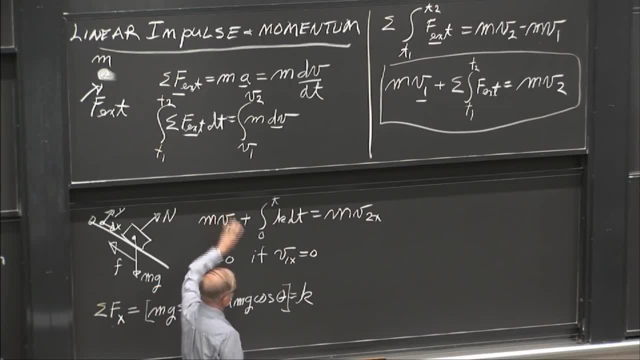 when you let it go to start with, then this term will go away And we can just implement this integral, and the integral of kdt is 0. kt, right? So this says then that kt evaluated from 0 to some time. 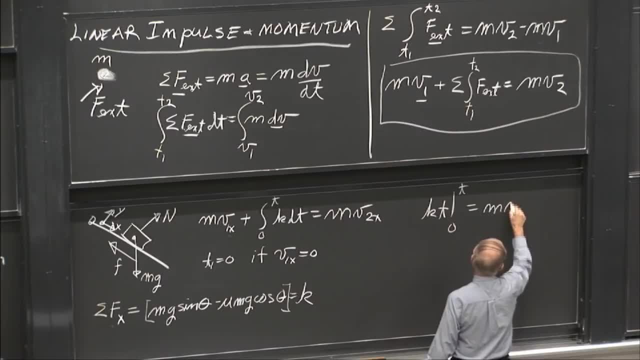 that we want to know. the answer is mv2 in the x direction, And so let's let t equal 3 seconds. You find out that v2x is 3 seconds, And that's it. That's it, That's it. 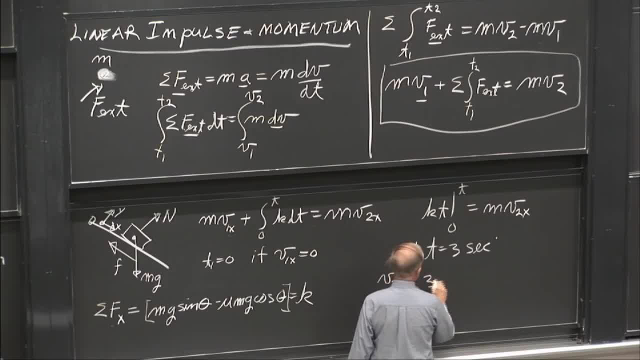 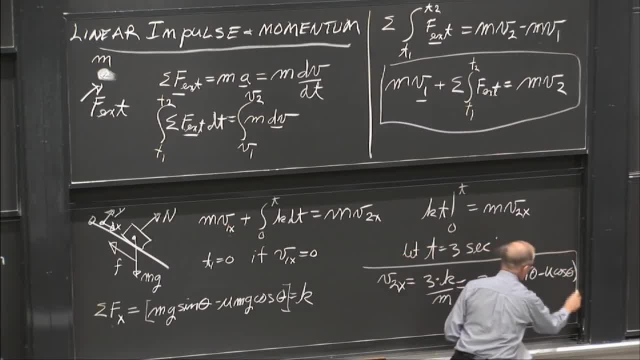 So really the trivial, almost trivial example. it's not a hard example but it emphasizes all of the key points in the problem. Start off with a vector equation. You can apply it in any one of the three vector component directions. You integrate the forces, the sum. 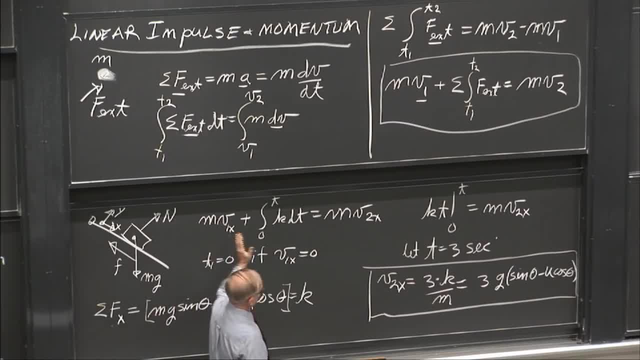 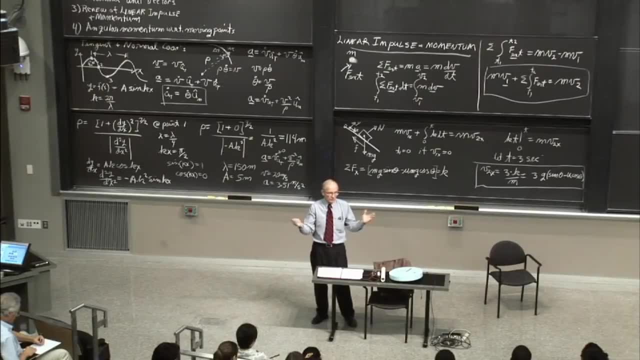 of the forces on the object in that direction over time And you apply the impulse momentum formula and you get the answer. You can do that So that basic step-by-step process is how basically most impulse momentum problems are done. And if there's no forces, then you. 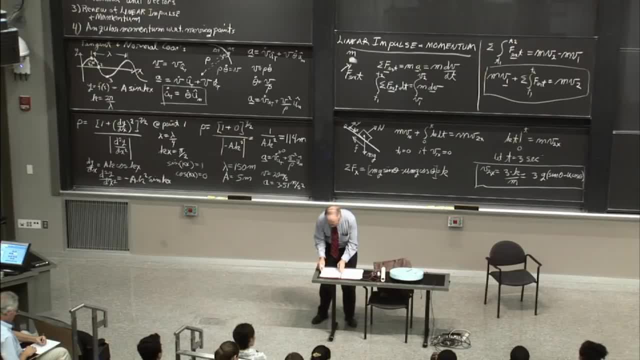 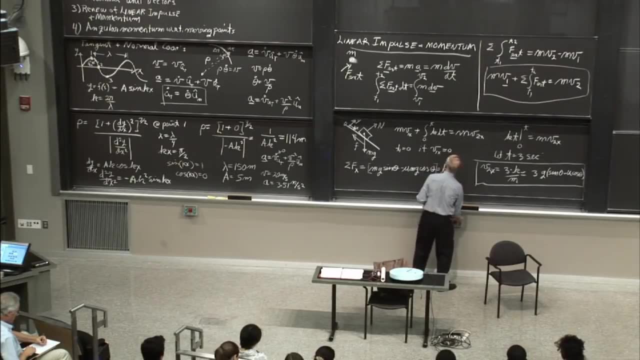 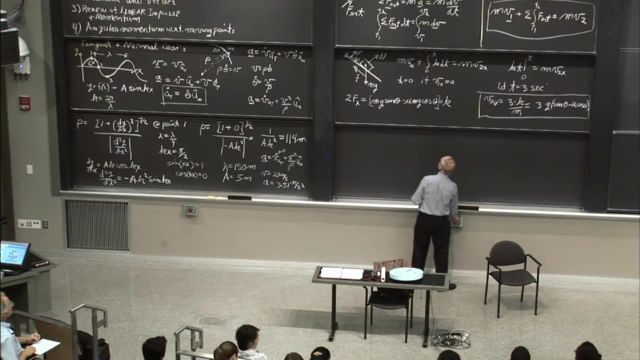 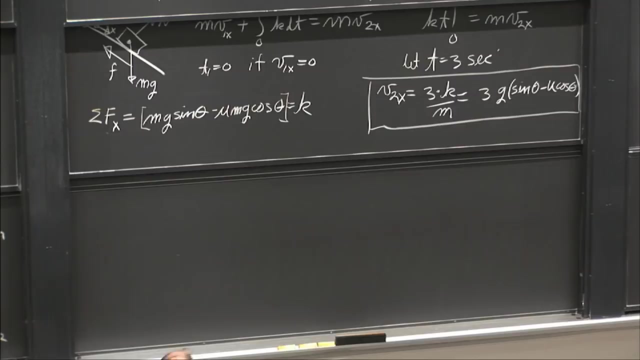 have conservation of momentum. OK, so let's do. this was for particles, Just a quick reminder. We need to ask ourselves: does this apply to groups of particles, Systems of particles? Well, remember that we said: if you've got a bunch of particles, a system, all of these. 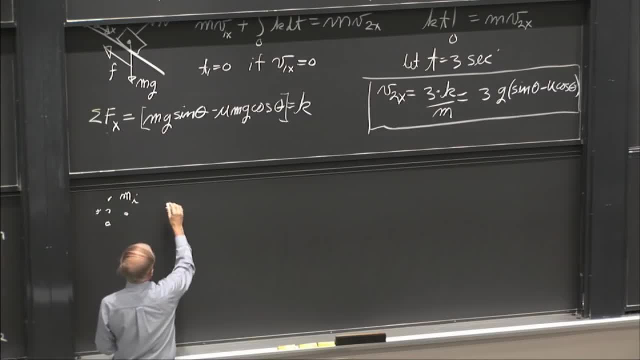 are the mi's. we've already figured out that the total mass of the system times the velocity of the center of mass. this is, g is my center of mass with respect to my inertial frame. So this is the momentum of the system. 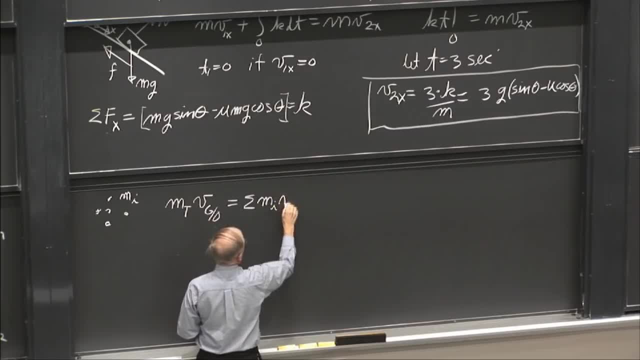 That was just a summation of the individual mi vi's with respect to o And, furthermore, we took the derivative of this. So this is the momentum of the system. The time derivative of the momentum should be the external forces, So that we were able to, by taking that derivative, 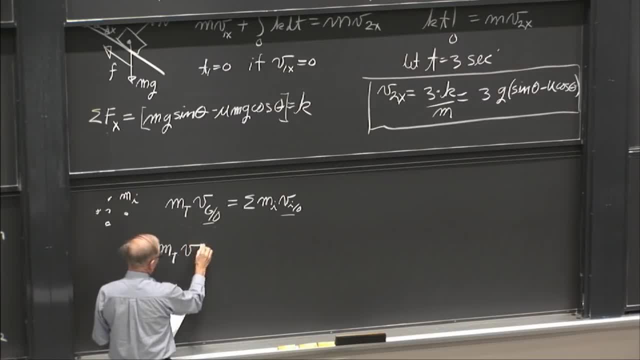 you get mt, the total mass times, v, OK, OK, v g with respect to o dot, And that had better give you be equal to the summation of the external forces on all the particles, Because you can do it one particle at a time. 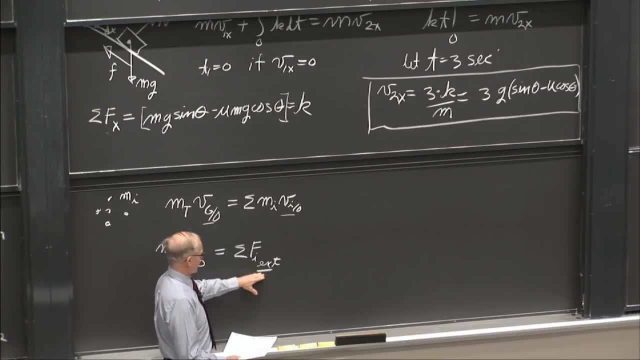 And each of these particles has forces. You sum them all up, you get these forces, And this allows you to say: You say that the sum of all of the external forces on the system is equal to the total mass of the system times the acceleration of the center of mass. 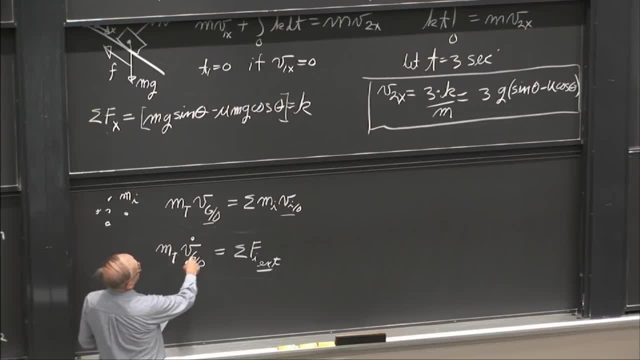 So this formula now can? it looks very similar to where we started with this little derivation for a particle. You can now say that the summation this all leads to, the summation of the integral from t1 to t2.. OK, Of all of these forces over time gives you. 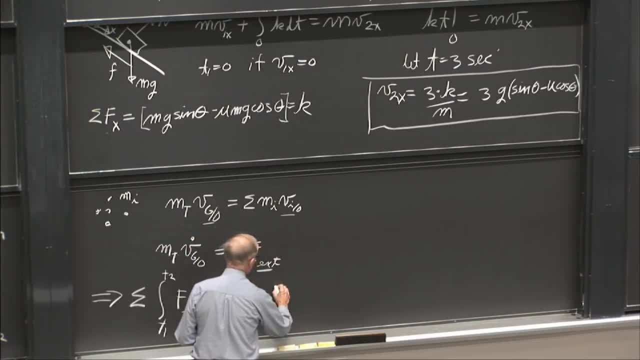 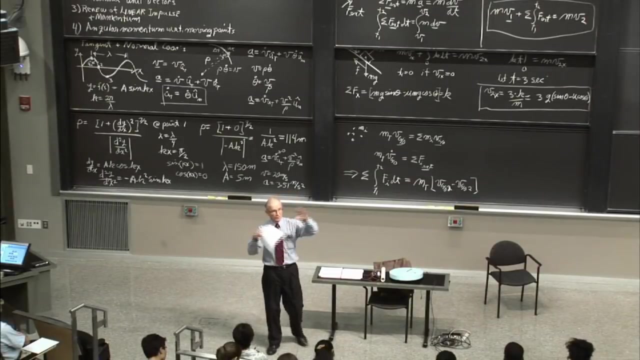 the change in the total linear momentum of the system: v g with respect to o1, 2, rather Minus v g with respect to o2, the second one. So this is exactly the same kind of form: The change in the linear momentum of the system. 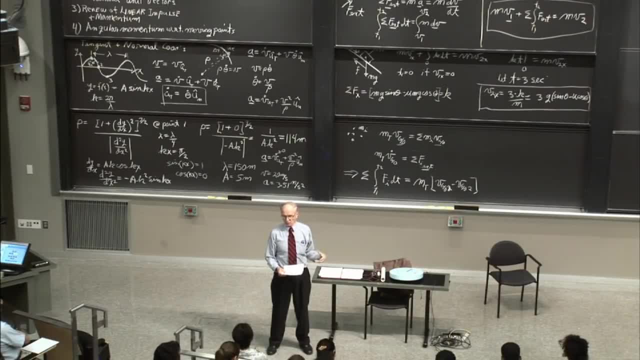 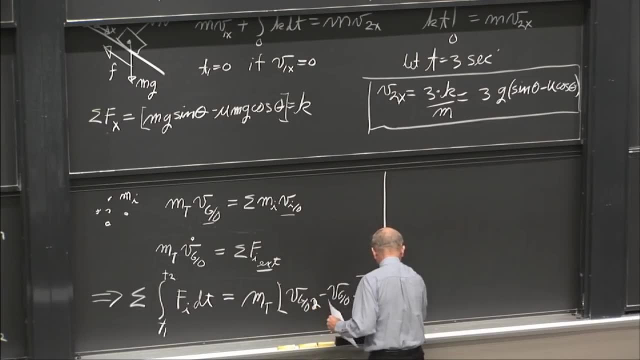 is equal to the integral of the forces on the system over time. So the impulse to the system, So this allows you to do problems that you might not have thought about before. So think about something like this: I've got an old revolutionary war. 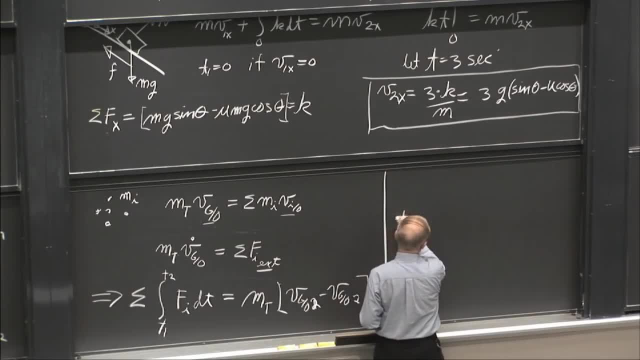 OK, I'm trying to draw a, so here's my cannon barrel, And back in those days I'll draw a little better job here. So we've got this cannon sitting here, And in the barrel you've got a bunch of what's known, as in the old days, known as grape shot. 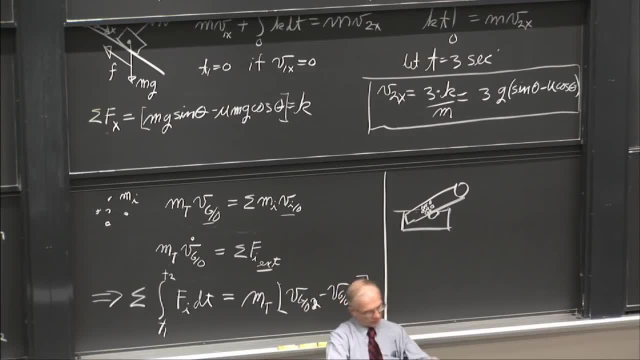 So sometimes for anti-personnel kind of stuff they would just throw a whole bunch of metal and junk into it. But just imagine a bunch of iron balls or lead balls or rocks or whatever you want to put in there, And you put a whole mess of them in here and you have a charge. 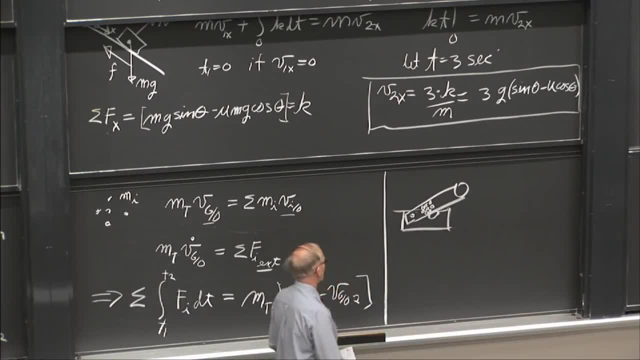 You set it off and it shoots them out. the end of the gun. I want to know what's the reaction, What's the reaction force on the gun When that gun, when that charge, goes off, if you go down to the Constitution, which? 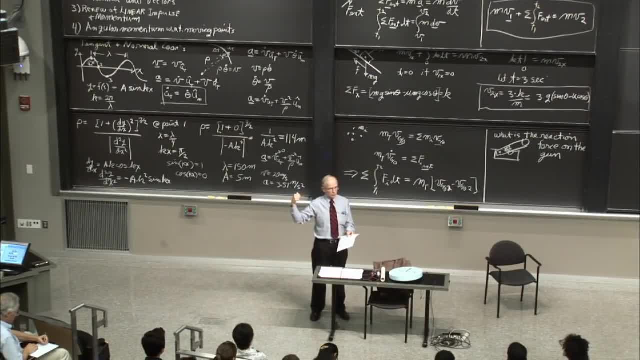 is the oldest commissioned warship in the US Navy still afloat. I don't know if any of you have seen it down here in the dock in Chelsea. It was built around 1799.. But when they shot one of those guns the gun would roll back. 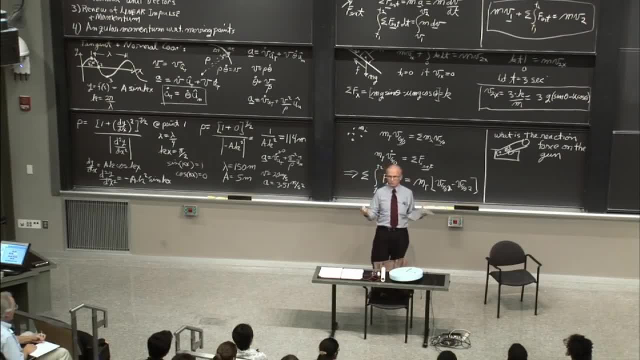 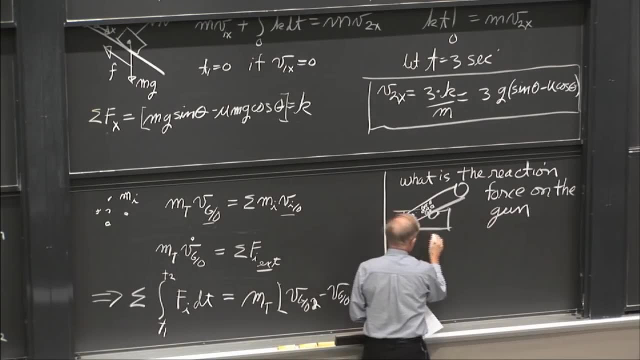 several feet and get dragged to a stop by a bunch of restraining lines And then dragged back up for another load. So the reaction force, the force pushing back- these things are usually sitting on wheels- could be pretty large. Let's take an estimate of it. 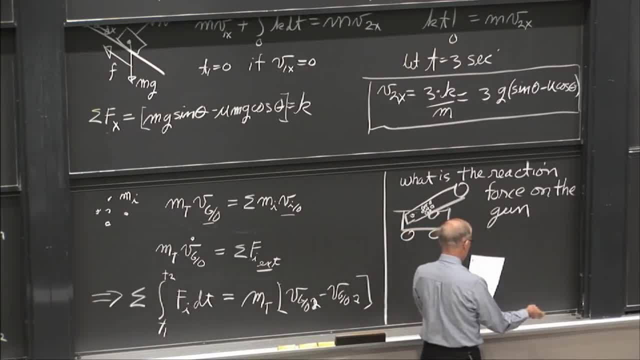 So this is going to be a relatively small gun. The total mass of the shot here, times g, is 10 pounds, So 10 pounds a shot. A gallon of milk weighs 8 pounds. This isn't a very big load, And let's say that this barrel here from here to here. 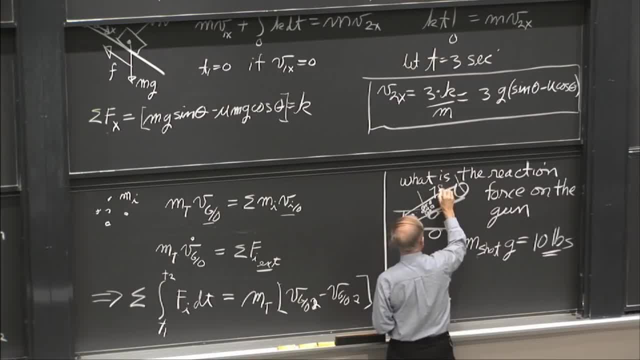 the acceleration length is 7 feet, So that shot's accelerated out the barrel over a distance of 7 feet And it has a muzzle velocity, an exit velocity of 700 feet per second. Are most guns subsonic, supersonic projectiles? 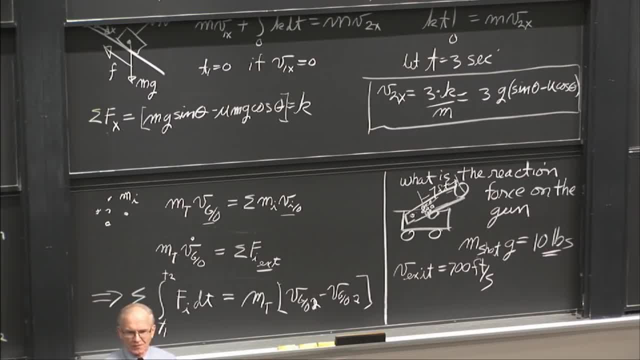 when they come out of guns. Have you thought about that? I'm just asking to see if you have a feeling for speed. How close to the speed of sound is that? So the speed of sound is about 1,100 feet per second. 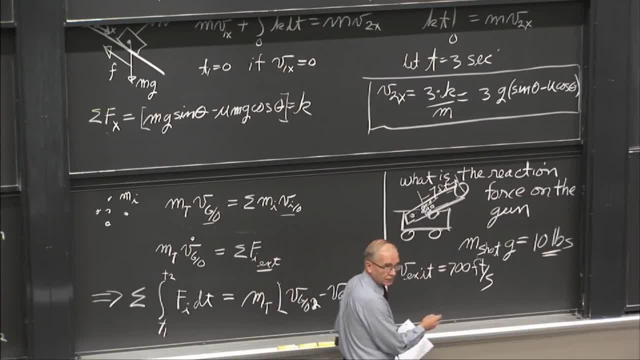 340 meters per second. So this is the order of Mach 0.6, or something like that. Something like 0.6, not 0.06, 0.6.. So about 60% of the speed of sound. 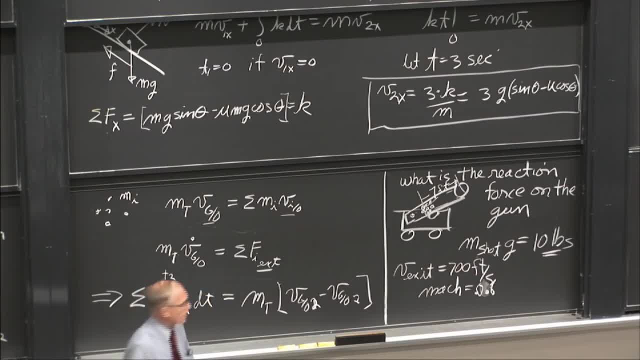 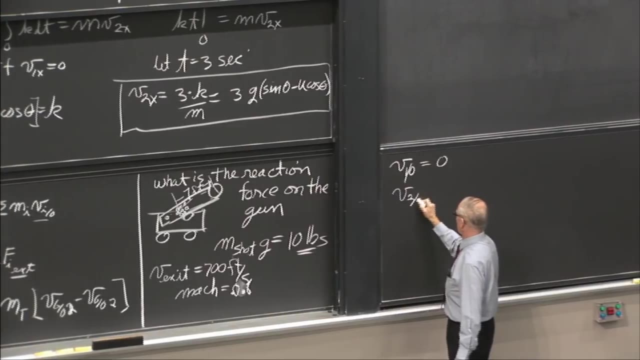 That's kind of slow actually as guns go. So the initial velocity- the shot's just sitting there- is 0.6.. 0.6., 0.6., 0.6. 0.6.. The final velocity is 700 feet per second. 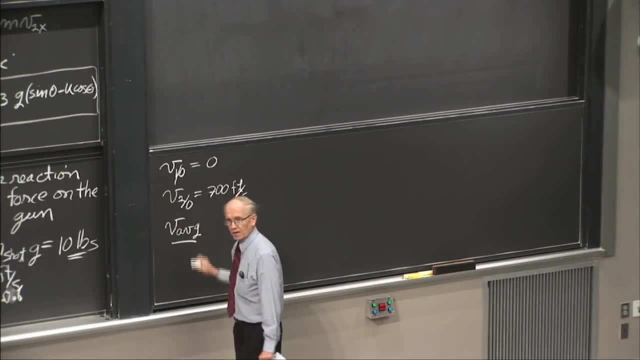 The average velocity, which I'm going to need for a second, because I'm just making some estimates here. The average velocity average of 0 plus 700, is 350 feet per second. The reason I need this is I need to estimate the delta t. 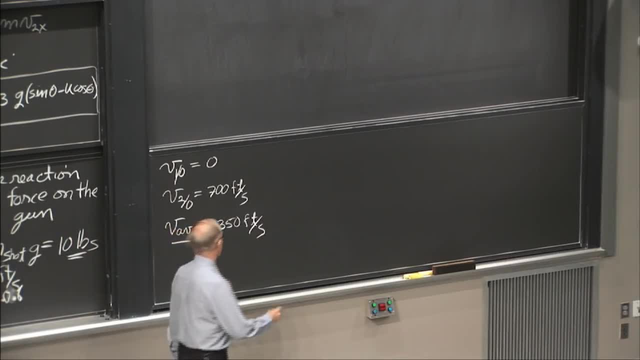 How long does it take to get the shot out of the barrel? So distance equals rate, times, time, right, So the V average times delta t equals 7 feet At 350 feet per second. you find out. delta t is about 0.02. 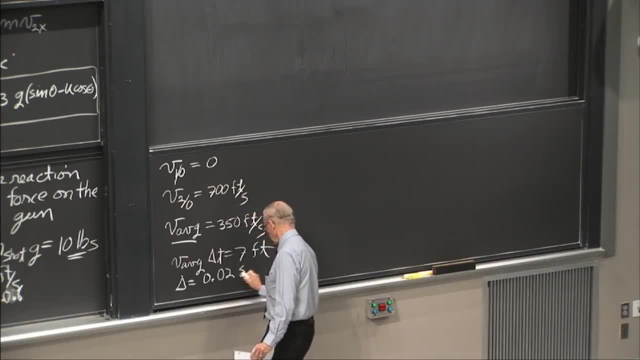 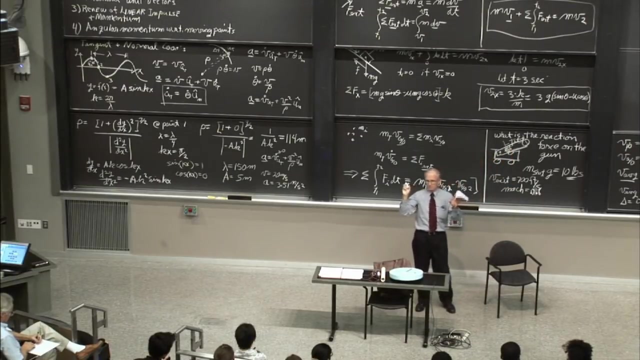 seconds. So it gets out the barrel pretty quickly. 0.02 seconds, 20 milliseconds. Now that powder, when it goes off it's putting a lot of forces on the shot. So the total force on the shot's 5,000 pounds. 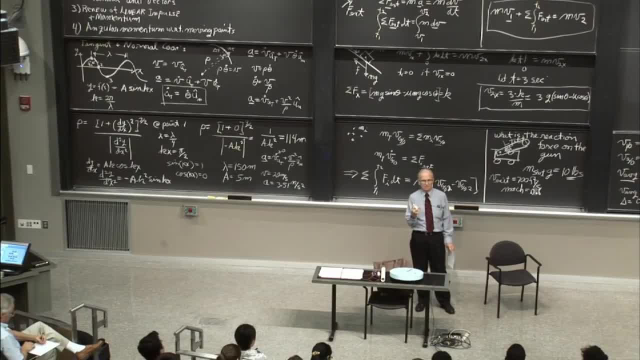 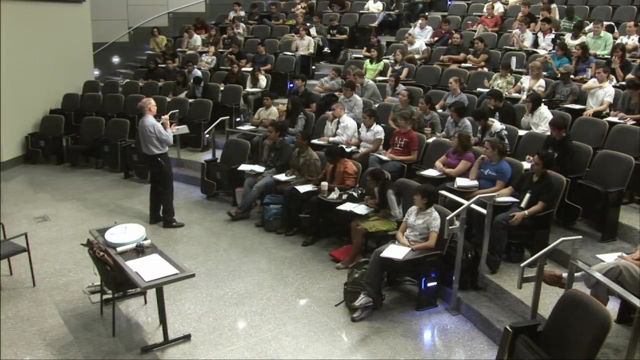 What's the reaction force on the cannon? So we're going to apply a principle here that we talked about earlier. Newton had three laws And this is a group. This is just massive balls in there. The hot exploding gases are pushing them out the barrel. 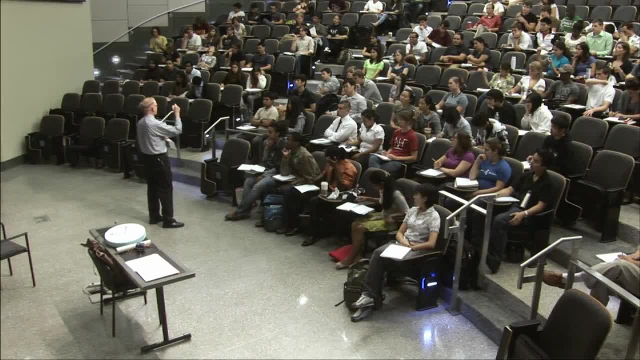 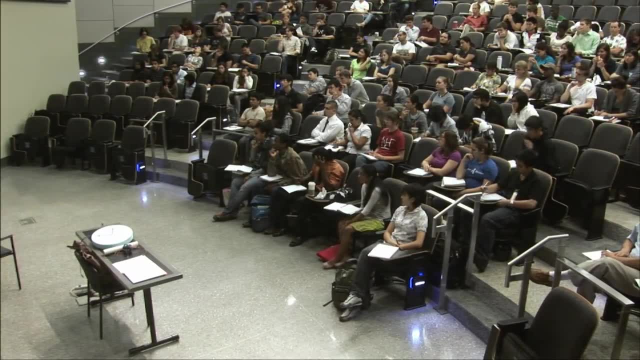 What must be the push of the same gas on the cannon that's containing it. Equal and opposite, Equal and opposite. Newton's third law, Right? So the reaction, Yeah, Yeah, The reaction, The reaction force that we're looking for. 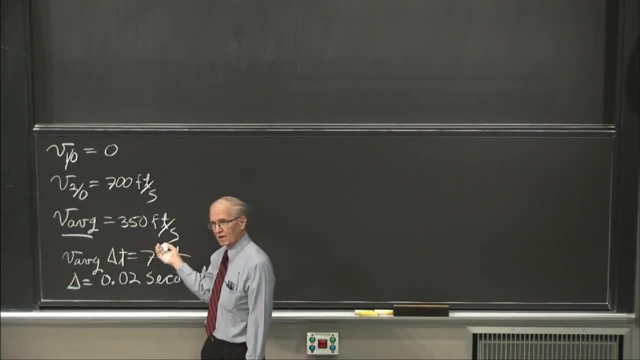 is minus the force that it takes to get the shot out the barrel, So the force on the balls on the shot minus the reaction force, And that's Newton's third law. So we're almost there. We're just applying now this concept of impulse and momentum. 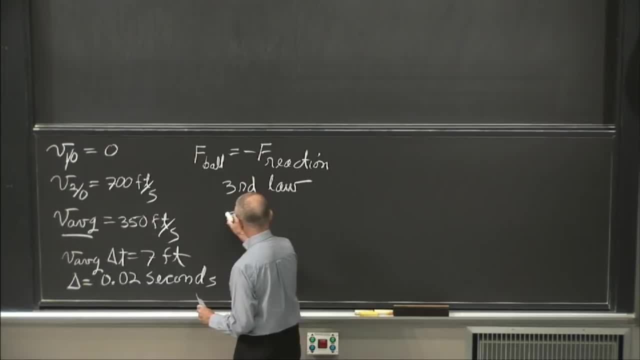 So now we can say the integral And this is the summation. You've got a whole bunch of balls in there. They've all got forces on them, But we're treating the group of balls as a system. So we can use this notion of the total mass times. 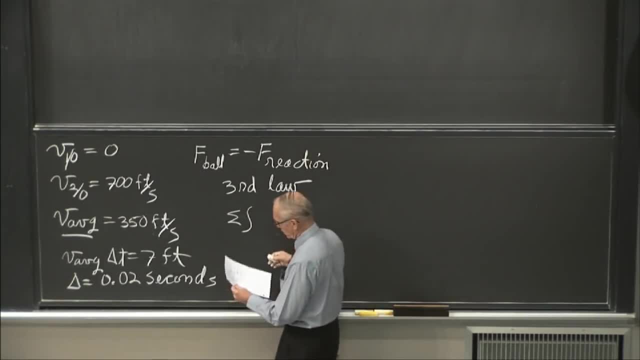 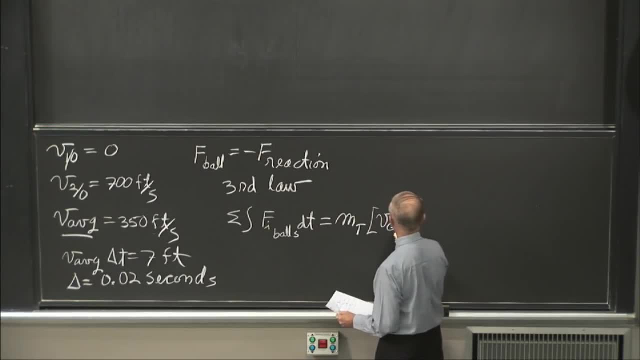 the change in the velocity of the center of gravity, the final velocity minus the initial velocity, This is 0.. OK, OK, We know this. We know this. So this mt is the 10 pounds over g. We know this is 700 feet per second. 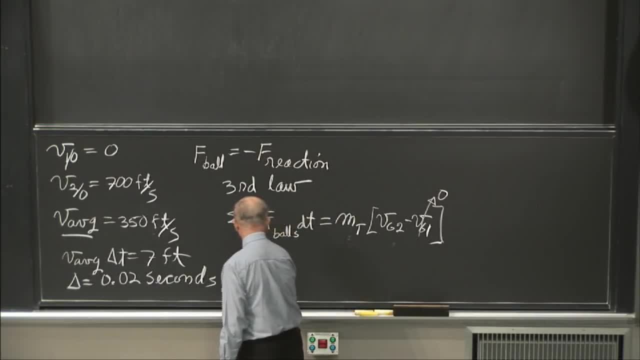 We know that all of this mounts up to the force external on the group delta t, And this is the weight of the ball w, And this is the weight of the ball w over g, And this is 700 feet per second. 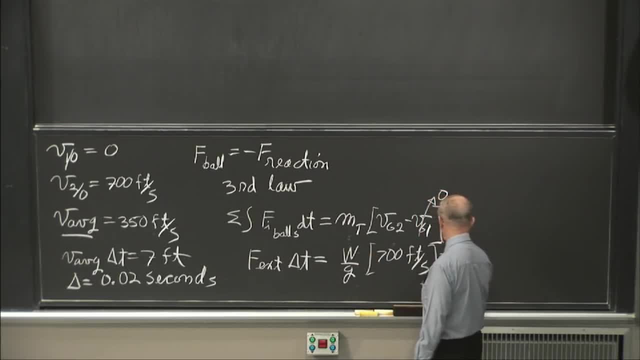 That's 10 pounds divided by gravity, 32.12.. And we need to divide by delta t, So the external force on the balls is w over g delta t times 700 feet per second. OK, OK, OK OK. 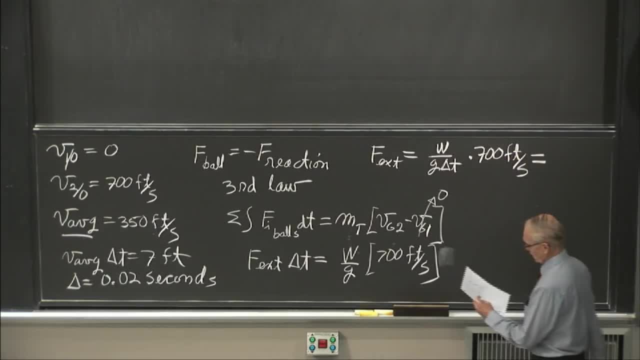 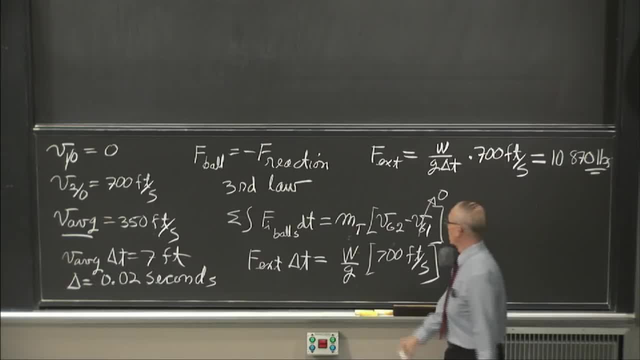 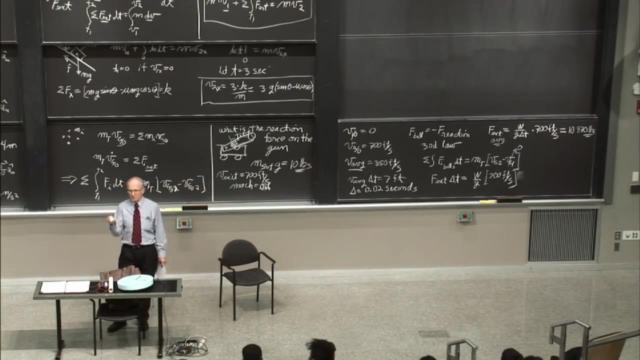 OK, OK, OK, Now this is an average force, right, Because delta t is the length of time it took, assuming we had some momentum. OK, OK, OK, We assumed an average velocity going down the barrel, So the peak force is probably higher than this. 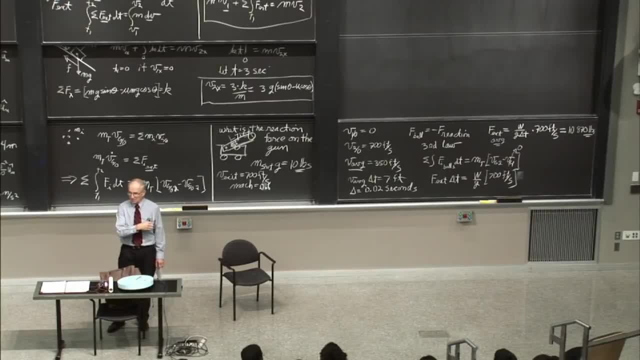 And the pressure in the barrel probably isn't constant. This actually isn't a bad estimate. If you know the muzzle velocity, which you could figure out probably from the distance it goes and things like that, you can make this estimate. So 10,000 pounds of reaction force is quite a lot. 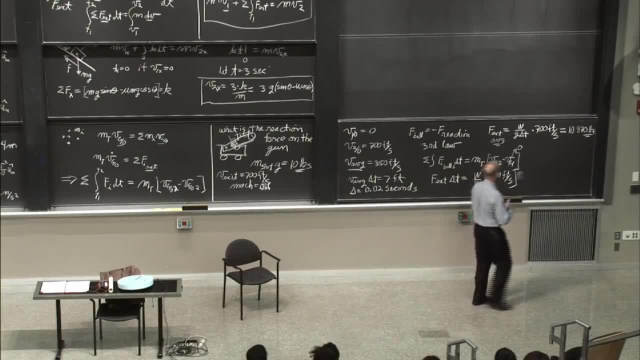 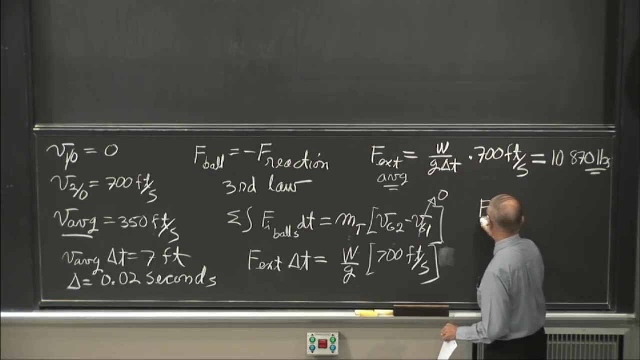 This is a dinky gun. 10 pounds a shot is not much, So this is the force to get the balls out the barrel. If it's positive, what's the reaction force Minus 10,870.. And all through this, I've been doing this in a single 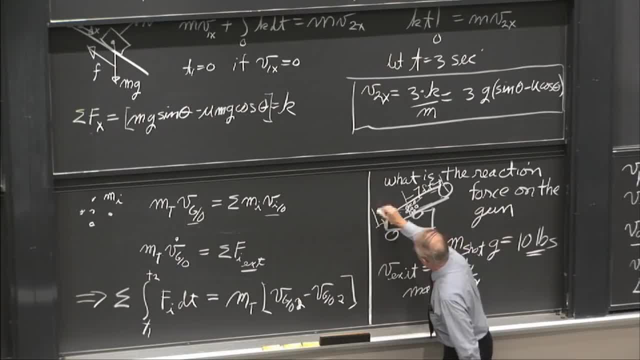 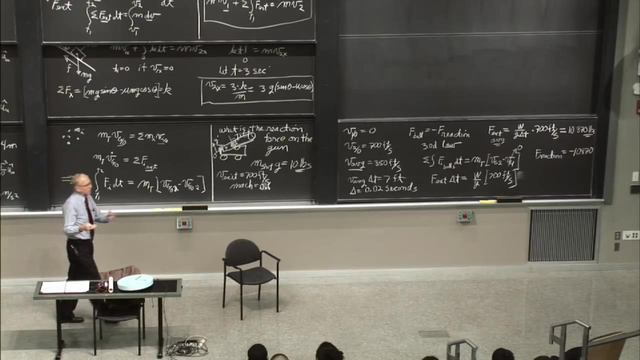 vector direction. So I would have set up my coordinate system like here's: O, this is the x direction, y direction. So this is obviously in the positive x direction is what I've lined up my positive velocities and positive forces to be. So just a really simple way, one of the kind of ways in 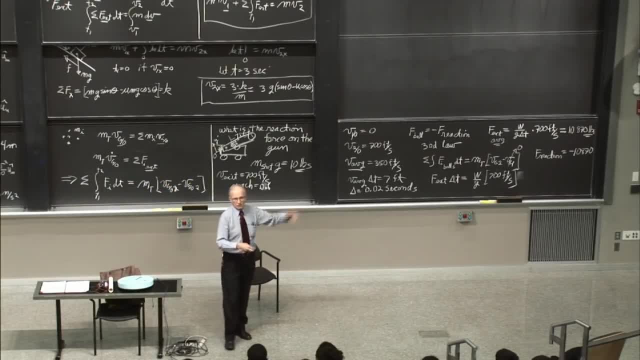 which you use this notion of impulse and momentum, But you can use it to make estimates too. Have you ever fired a shotgun? Yeah, Any kick Right. So what gauge shotgun did you fire? No, no, OK, OK, 12-gauge shotgun. 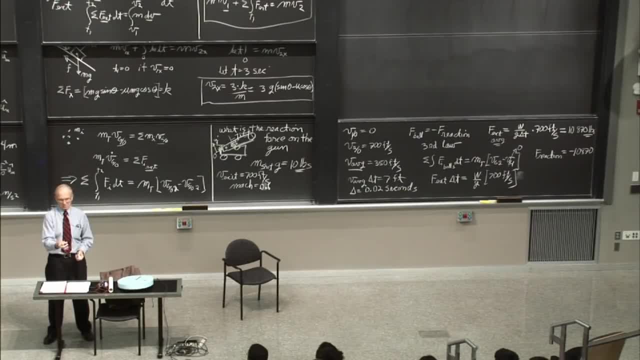 You know, The cartridge is about 3 quarters of an inch diameter And it probably has a little amount of powder in there. It mounts up to about that much stuff, But it can give you a bruise in the shoulder if you don't hold it right. 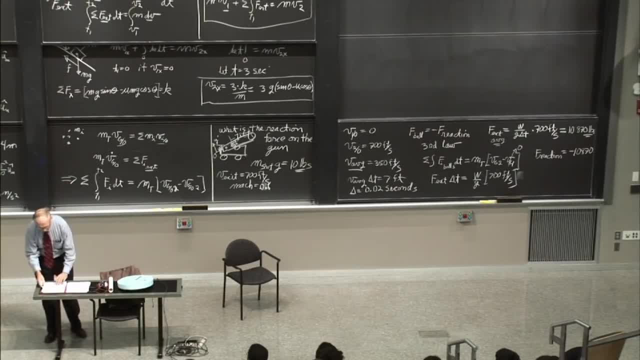 So that's what this is about. All right, So this is kind of a quick review. You've done lots of conservation of momentum problems in your time. The homework set this time has two or three problems on it that are: conservation of momentum, linear momentum. 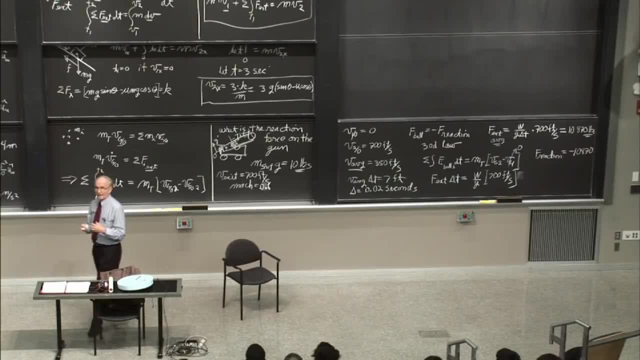 But now I want to move on. I want to move on to talking about angular momentum, And angular momentum in a way in which you probably haven't done angular momentum problems before. So anything about the last thing on this, So mostly this: I want you to read the chapter. 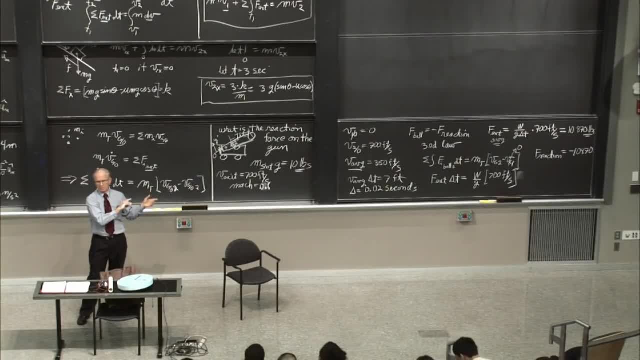 I think it's chapter 15.. First few sections of it are on linear momentum. The last few sections are on angular momentum. Go read them and just work the problems. That's where they are. That's where you'll get most of your refresher is doing. 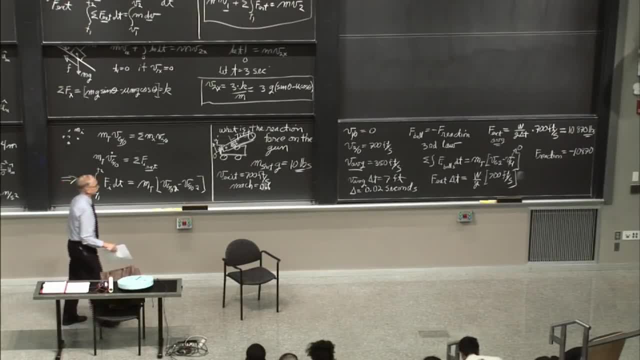 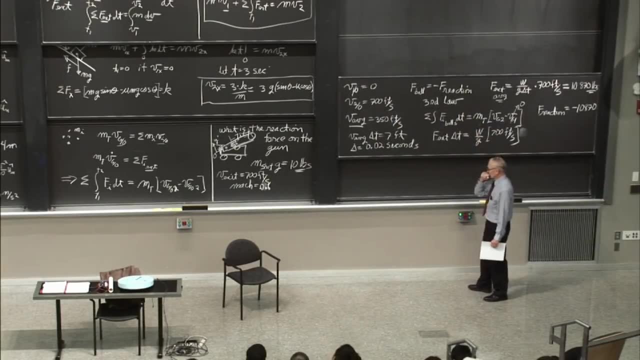 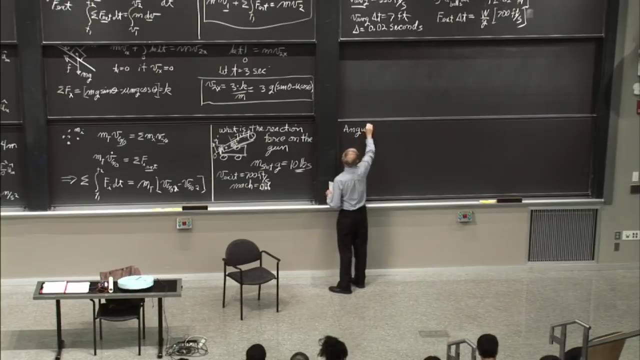 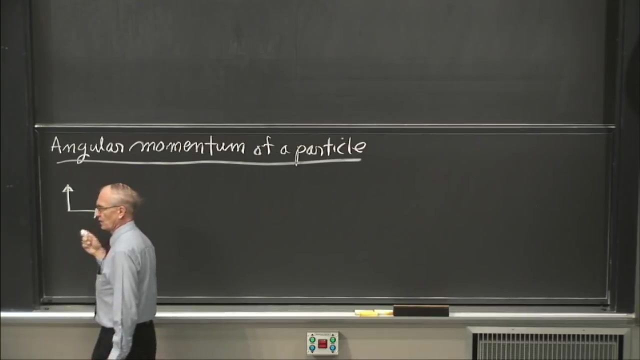 the practice problems. OK, angular momentum. So we'll start with a particle. We're very rapidly going to get to rigid bodies Now. many times you've done angular momentum problems before, mostly rotations about fixed axes. So here's our inertial frame, fixed xy. 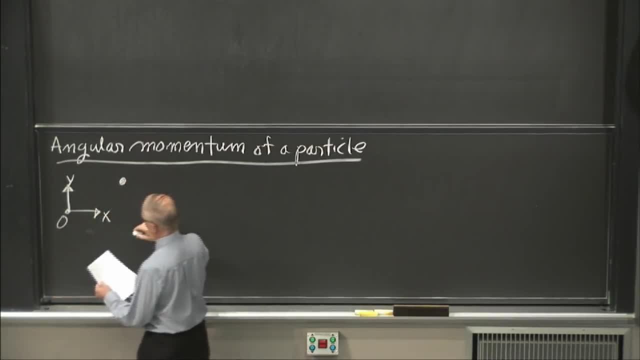 And you have a particle out here And I'll just do this, OK. OK, It just has some mass m And it has some total force on it. The force- and this is the particle- is located at b here. So the force at b, total force at b, just some vector. 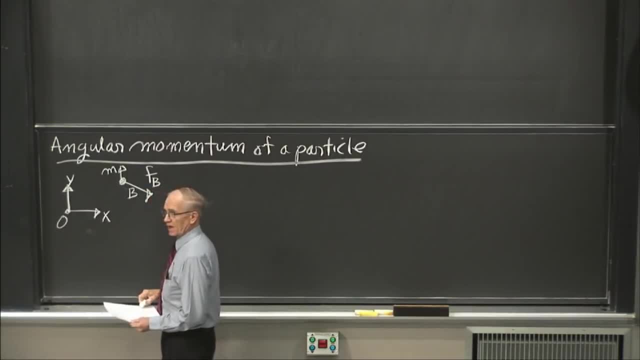 It also is traveling with some velocity at that instant in time, so it has momentum, And the momentum is p of this particle at b with respect to oh, And I'd like to the standard expression then for the angular momentum of this particle at b with respect. 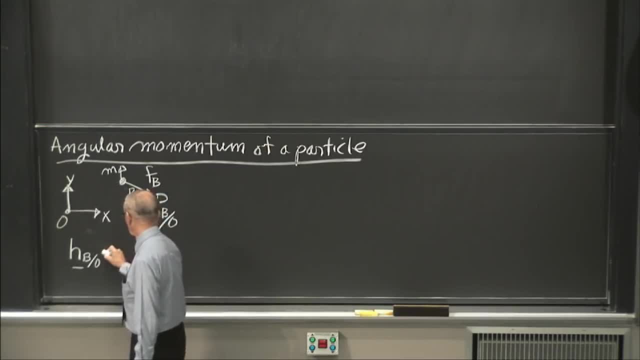 to: oh, we have a position vector here, rbo, which we've used lots of times. By now It's just the cross product of the position vector with the linear momentum, And that's the definition of angular momentum. I'm using a lowercase h here because I'm 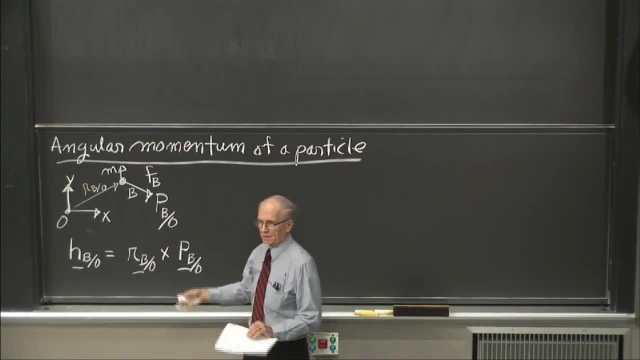 going to do that to indicate single particles, And I use a capital H later on when we're referring to rigid bodies. So the angular momentum of this particle with respect to this point is given by that And where you've used this before then. 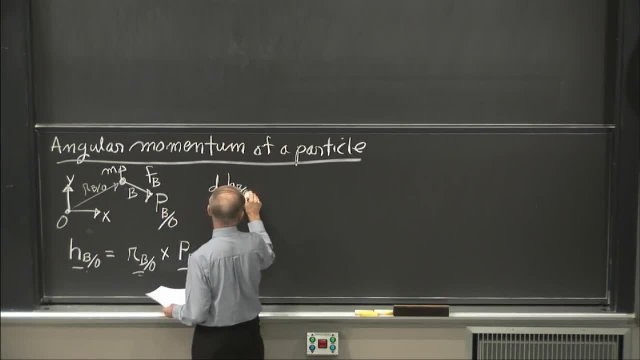 is the derivative of hb with respect to odt. is what is that? Remember? where does this give you The time rate of change of the angular momentum is the torque Right And it's the torque, it's the sum of the torques. 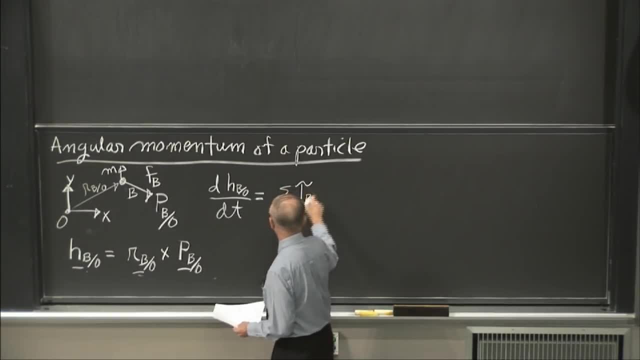 Right And that's applied on that object with respect to the coordinate system in which you're computing the angular momentum. So you've used this formula many times. And in planar motion, where you only have one axis of rotation, usually the z-axis of rotation, 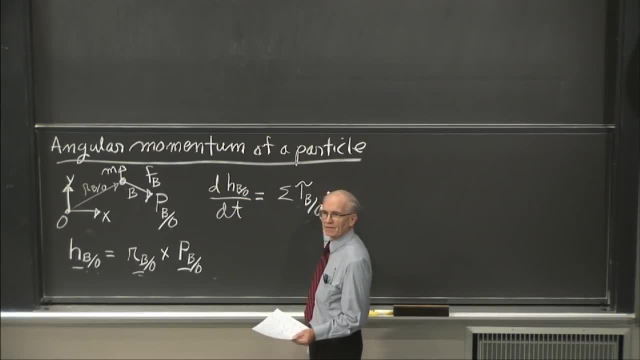 you usually would write this as i: theta double dot In its simplest form. if it's a rigid body, it has some mass moment of inertia times. theta double dot is equal to the sum of the external torques. So that's where you've met this before. 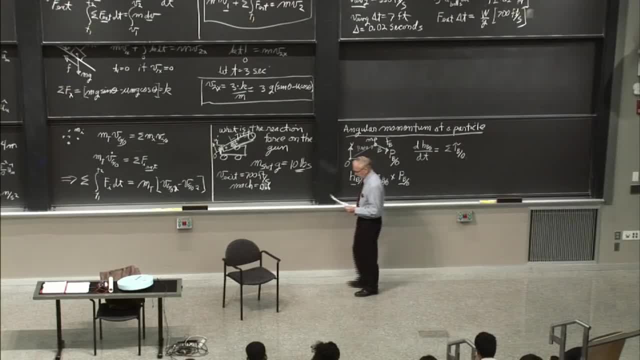 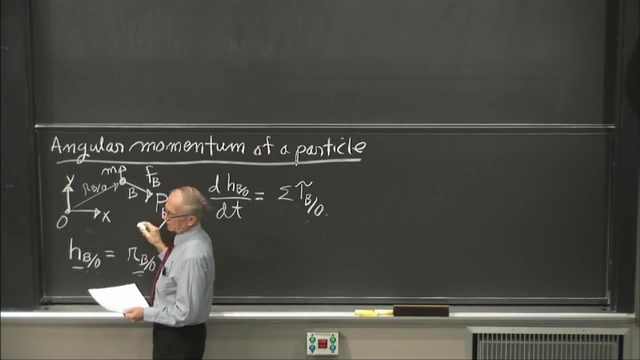 But for the moment this is just a particle. Let's stick with a particle. So the piece that's new here, probably new for you, is that? what if I want to know the angular momentum with respect to another point? So here's a point a. 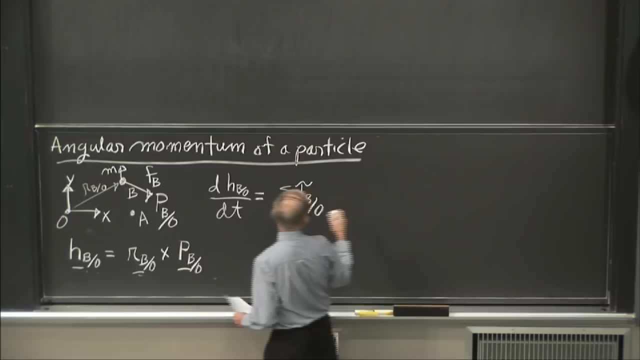 And I'd like to compute h of b with respect to a. Well, that's r. b with respect to a cross p b with respect to o, And this is really easy to forget. The momentum is always calculated with respect to your inertial frame. 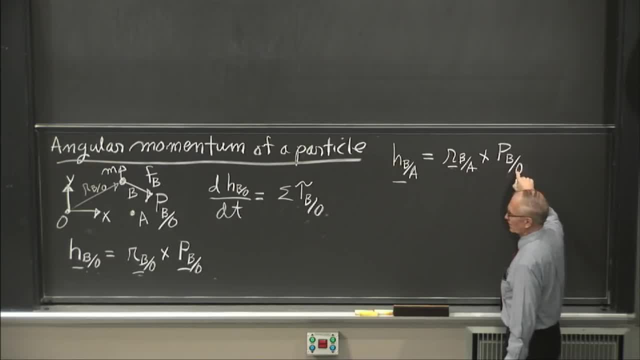 And that's why keeping this with respect to and telling you what the frame is is pretty important. But we're out here at some arbitrary point, computing the cross product of the position vector from this arbitrary point to this moving mass, And we're defining. this is just a definition. 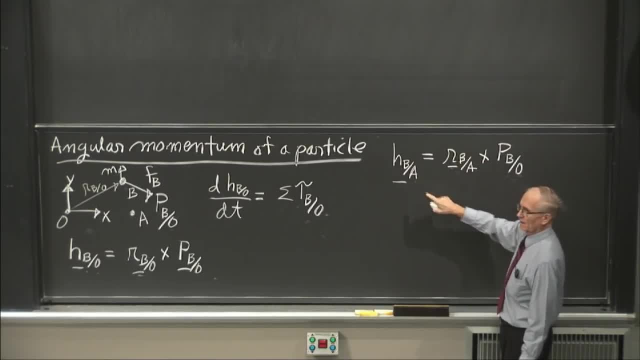 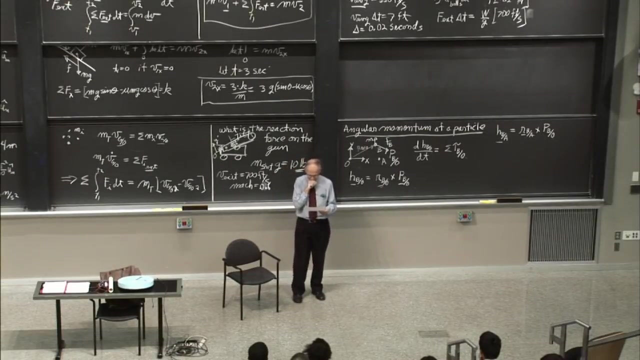 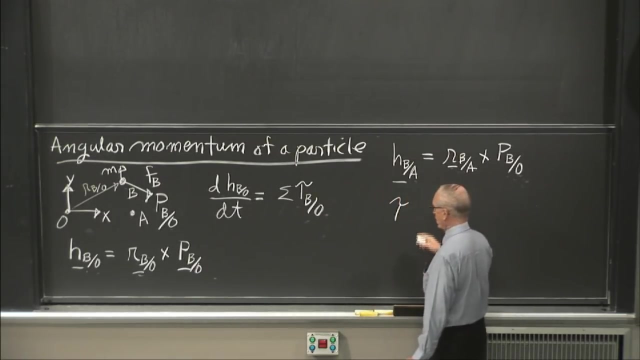 defining the angular momentum, with respect to this point, a as r, b, a cross, p with respect to o. All right, Now. what I want to get to is: now is the torque on this system, on this particle, around this particle. b with respect to a is the time rate. 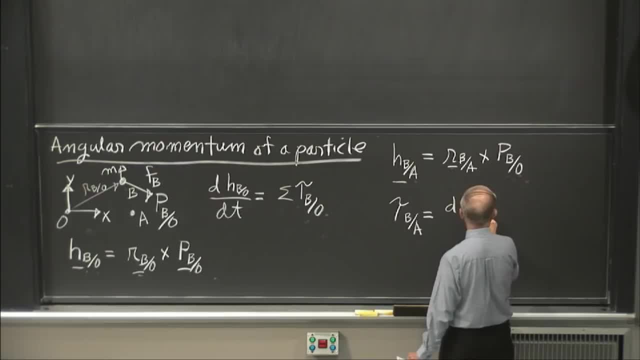 of change of h. All right, All right. So I've got r b, a with respect to t, But now it's a little more complicated, Plus the velocity of a with respect to o, through all vectors cross p b with respect to o. 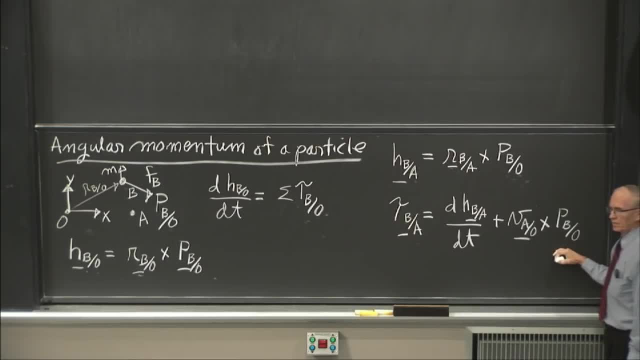 Messy term. I was trying to think of an example where you might want to do this. So imagine that you've got an arm which can rotate- It might be on a robot or something like that- And it has attached to it another arm. 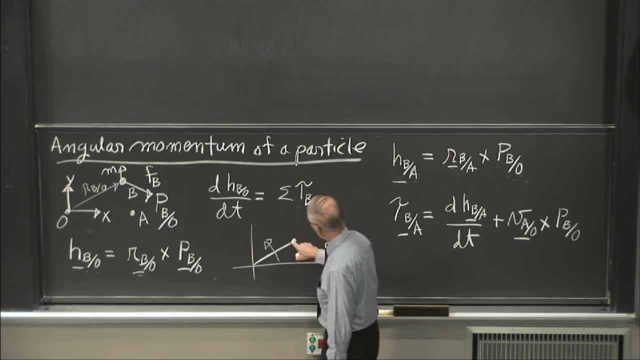 with a mass on it And you've got a motor here which can make this, this rotate, And you're trying to design The motor has to be able to put out a certain amount of torque. So this is o, This is b. 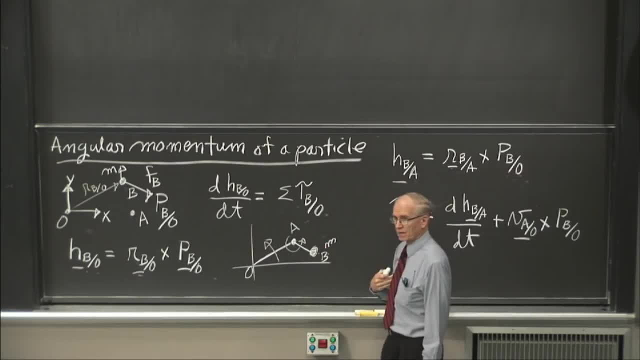 This is a, And you actually, I want to know the torque required in this motor to drive this thing around. But the motor is here And it only cares about what it feels. So the torque at this point to drive this thing, But this whole system. 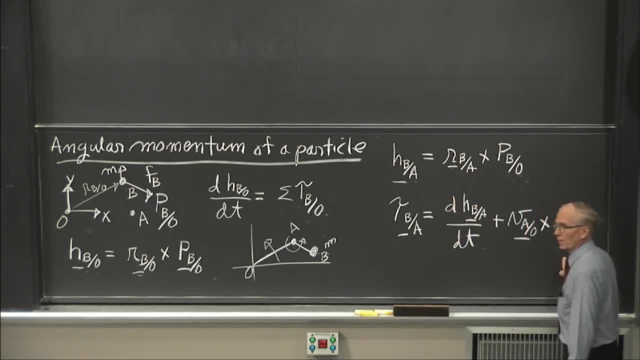 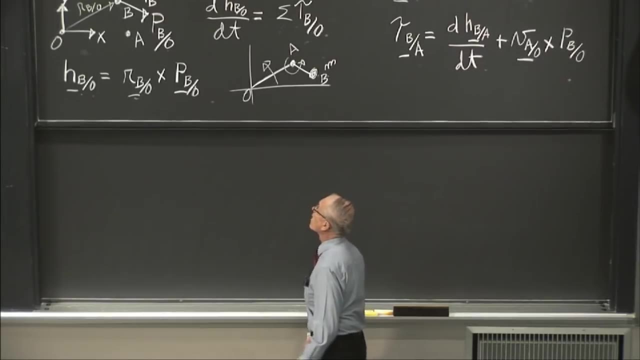 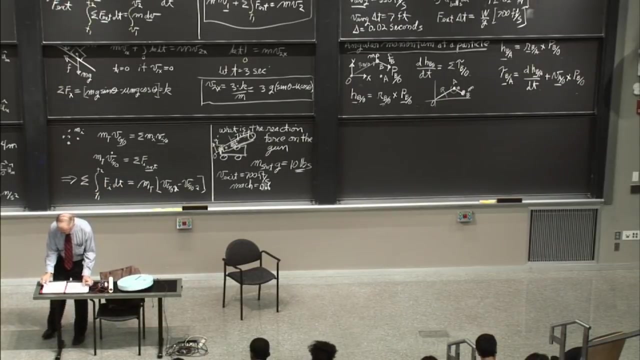 This whole system is now in motion. You'd have to use this formula. So there are practical times when you'd like to be able to calculate something like this. So there is. I'm going to show you a very brief derivation of this. 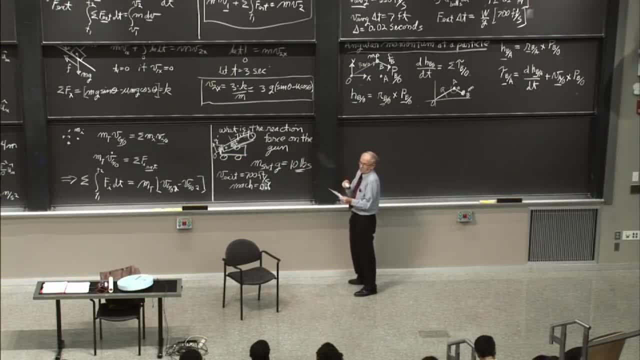 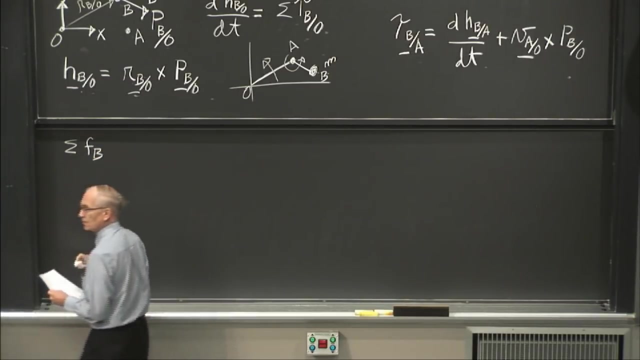 And What. But just so you can get a feeling for where this comes from, because there's a couple of outcomes that are very important to us. So the sum of the forces there at those forces at b give you the time rate of change of the momentum at b. 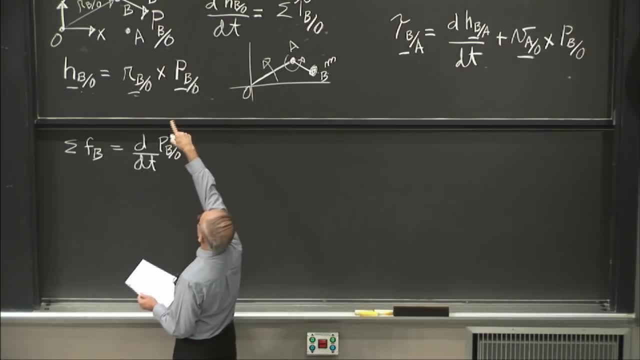 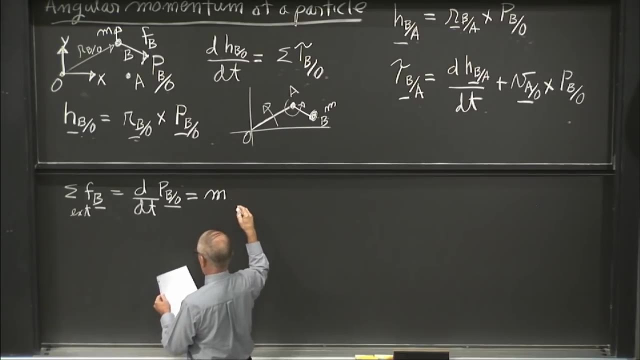 with respect to o, This is that momentum vector of our particle, And this Fb, this is the total external forces acting on the particle. We know that's m single particle times the velocity of the particle. That certainly could be right. 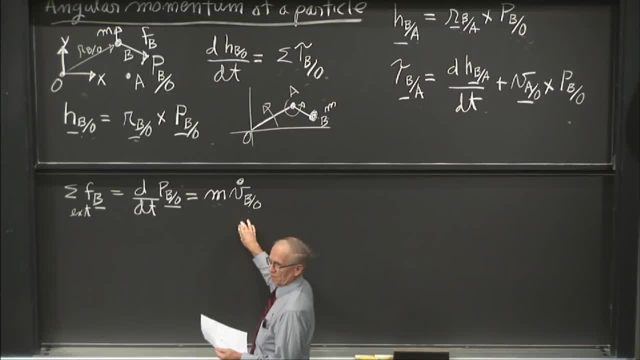 That's our familiar formula for F equals ma right. So the time derivative of the linear momentum gives you this, And the torque of b with respect to a is r. So rba cross this total. let this just be a total vector. 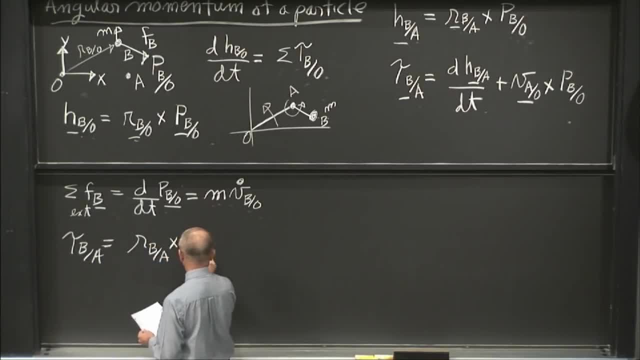 I'll call it Fb. it's a vector. The torque, with respect to a, is just rba, cross this total external force, And that's rba cross the time derivative, And that's rba cross the time derivative of PbO. 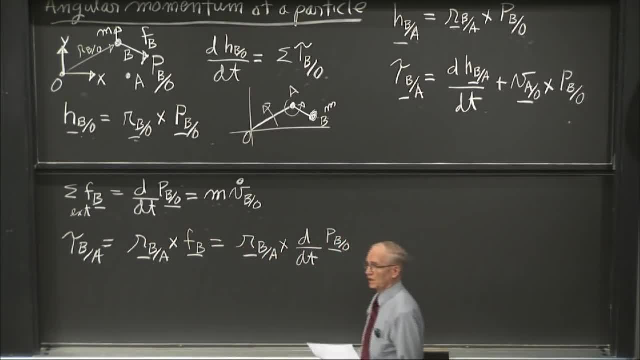 Because the forces give us r, which is from the time rate of change of the linear momentum of that particle. So I can say it like this. But now this: there's just a little vector identity for products of vectors that I'm going to take advantage of. 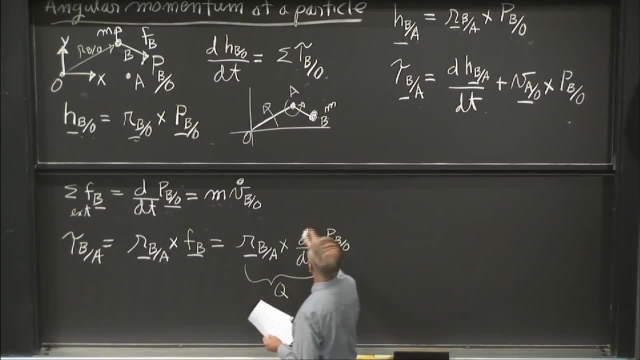 And I'll call this Q. So Q is of the form And I'm going to say: Matt, this is a vector a And this is a quantity, a time derivative of a vector b. It's a cross, db, dt. So there's a little identity that you can use. 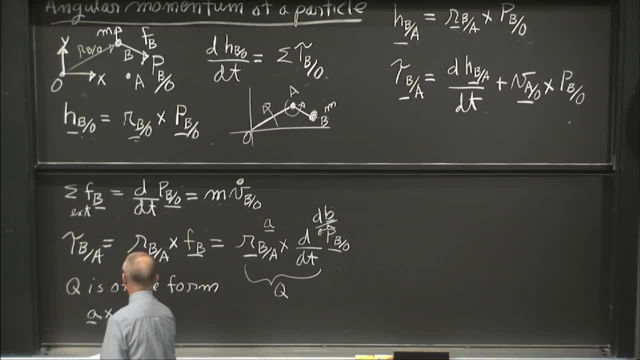 It says a cross db dt. You can alternatively write that as the time derivative of a cross b minus the time derivative of a cross b, And we're going to take advantage of this And just Reconstruct this formula using this expression, So that says torque of b with respect to a. 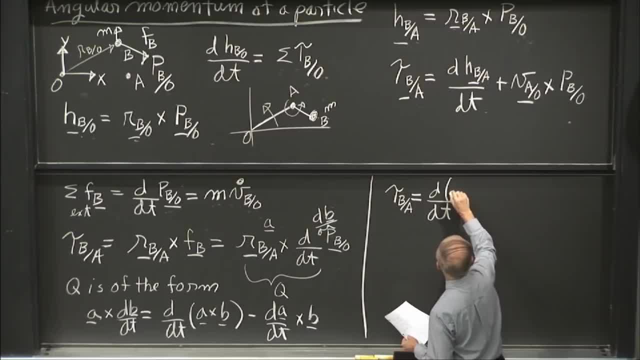 is the time derivative of rba cross pbo minus the derivative of rba cross pbo. So we've just made this substitution down here in terms of rba and pbo all vectors. But we know that rba And pb. 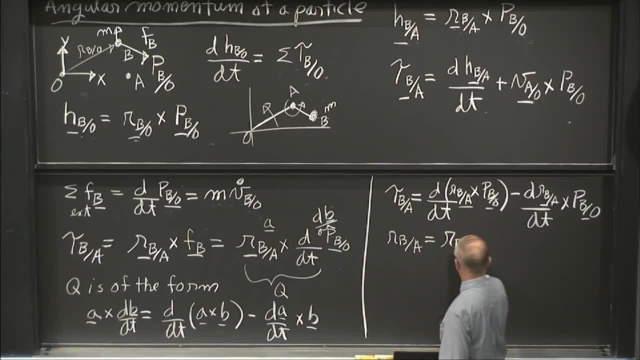 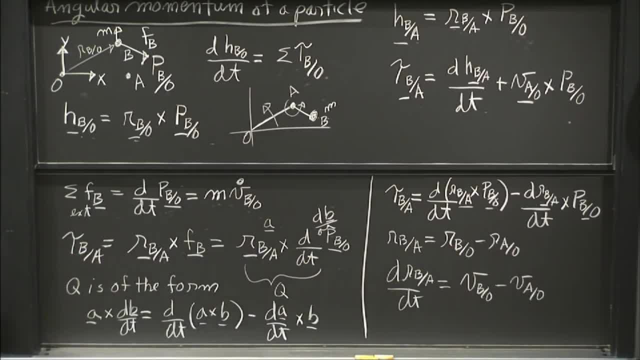 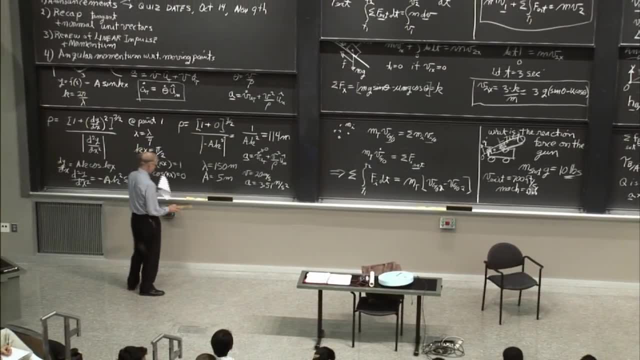 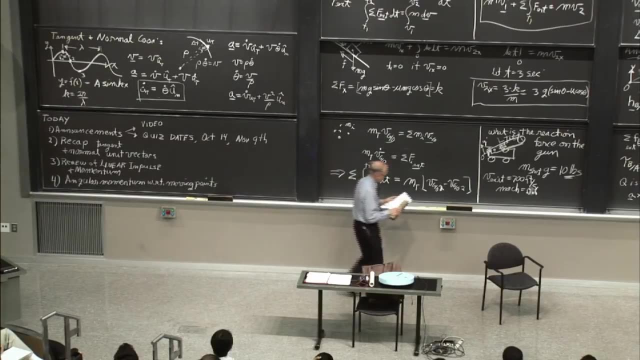 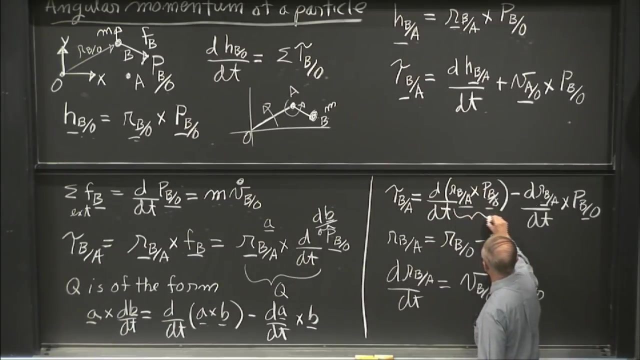 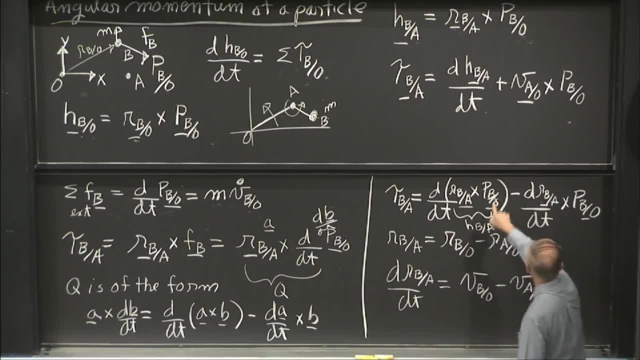 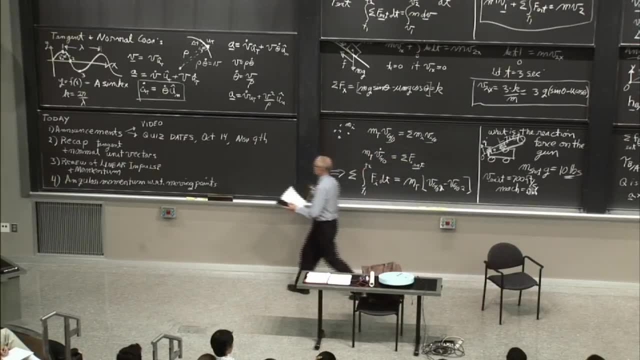 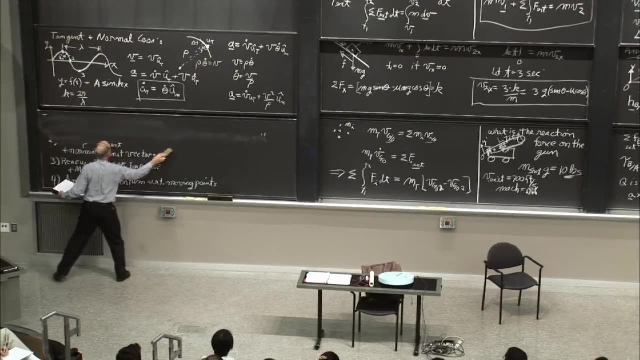 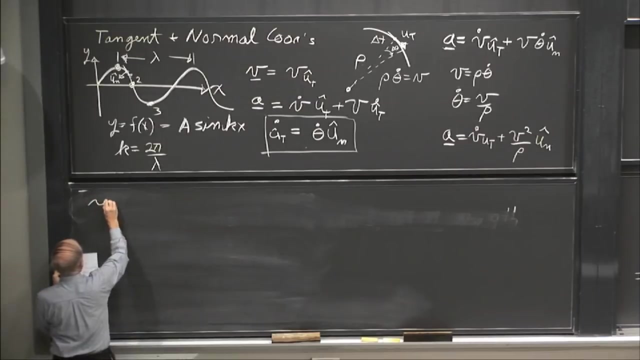 It's just r cross b, if you recall. So then we can rewrite this expression for the torque as the time derivative of h of b with respect to a. That's because of what I pointed out there. And now this is minus vbo, minus vao. 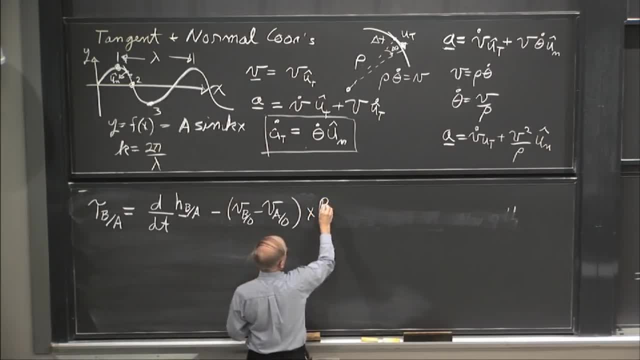 So vbo cross pbo. So p of b with respect to o is just m velocity of b with respect to o right. So vbo cross pbo gives you what Nothing Gives you: 0, because they're in parallel. 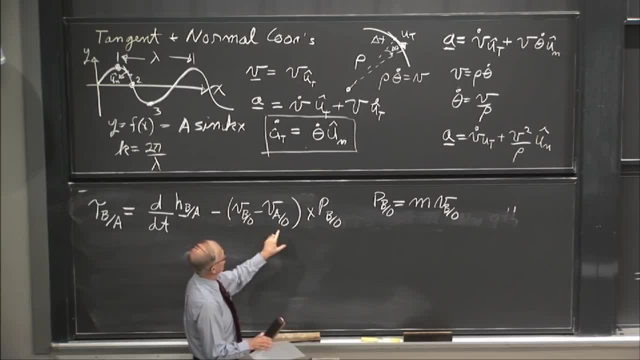 They're going, They're in the same direction. So you only get a non-zero piece out of this. Minus times minus gives you a plus And you end up with- And that's what we said, And that's what we set out to find. 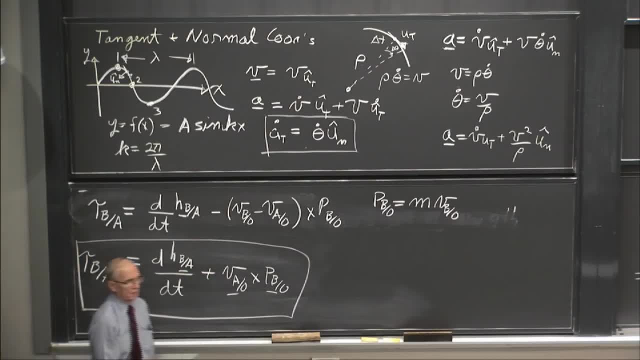 I said, this is where I was trying to get, And now we're there. Now, importantly, there's a couple of special cases of this. This can be kind of a nuisance term to have to deal with Lots of times. you'd like to be able to get rid of it. 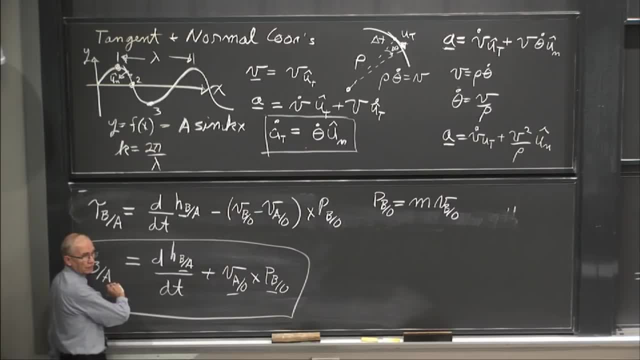 and just be able to go back to that old, reliable formula that torque is time, rate of change of angular momentum. So there are two. There are two obvious- almost maybe obvious- conditions in which this will go away. What's the most obvious one? 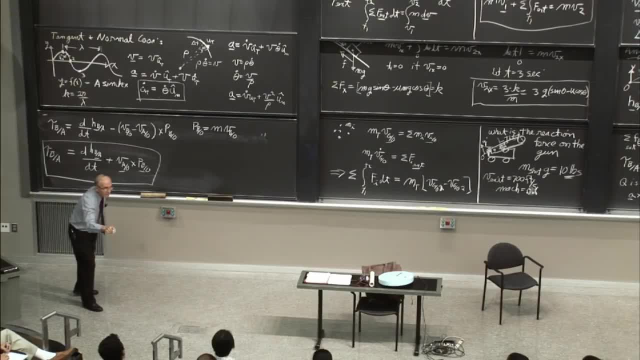 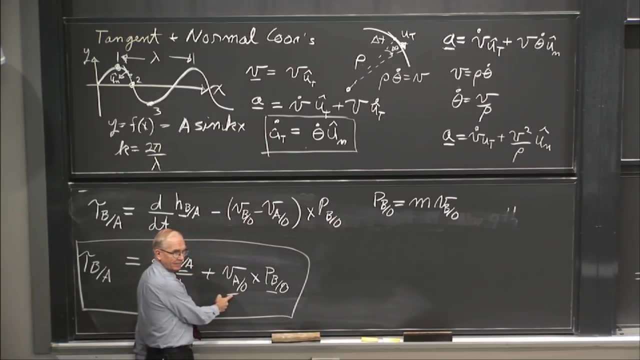 One of the terms is 0.. What did you say is 0?? One of the terms is 0.. Well, yeah, This term, presumably not This guy, If this is 0.. It's just back to our old, familiar formula. 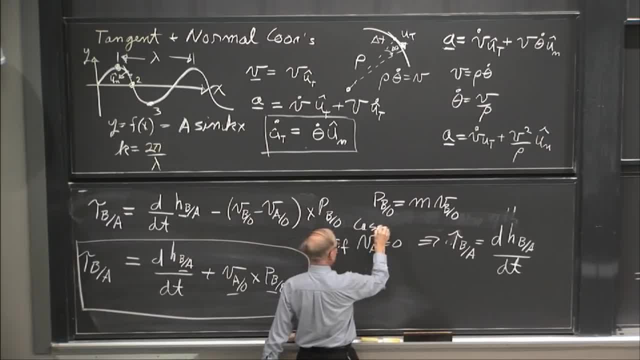 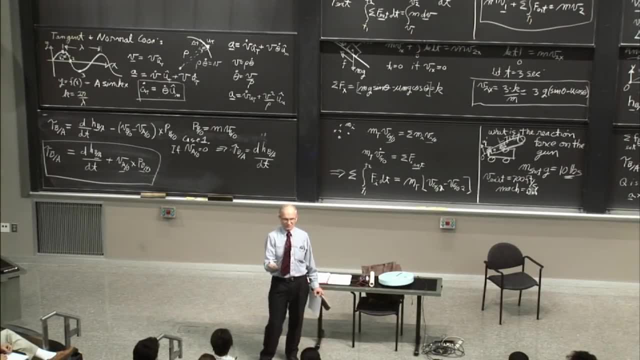 That's one case, so case one. But now, actually, this is a really important result, Because a can be anywhere As long as it's not moving, And so this allows you to do things. talk about rotations, about fixed axes, that. 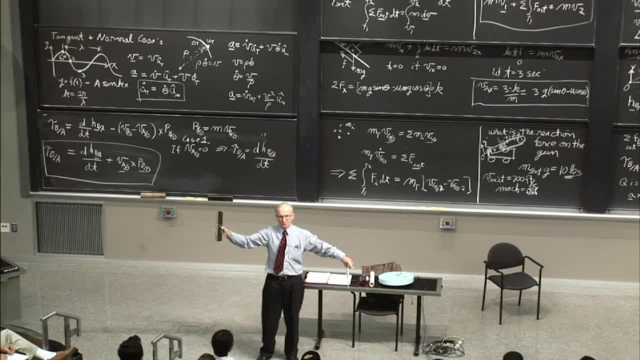 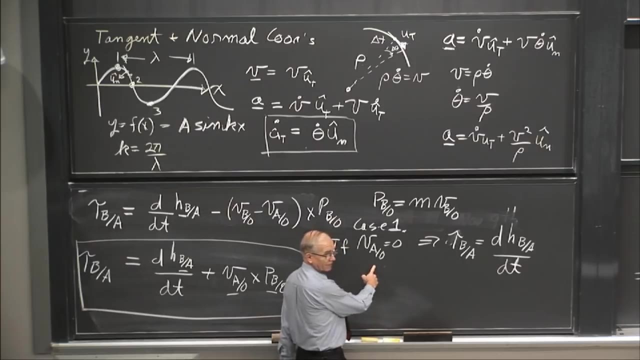 aren't at the center of mass Right. So if you have a fixed axis of rotation and something going around it, that's what this allows you to do. That's one case. So this will soon get to rigid bodies- Rigid bodies. 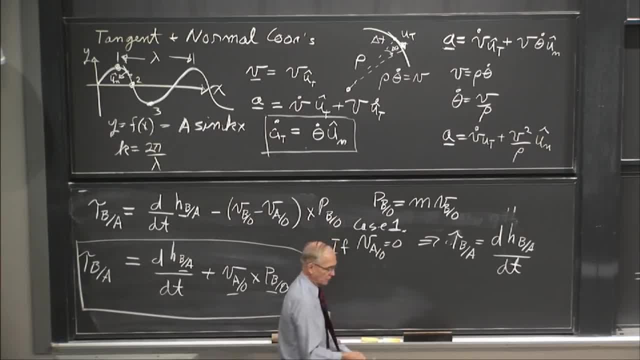 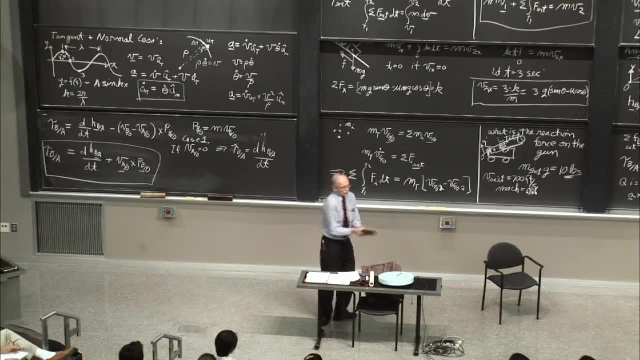 Rigid bodies would be exactly the same formulas. And you can have a rigid body now that is not rotating about its center, but rotating maybe about its end. like this, That formula applies if the velocity of that axis about which it's rotating, about which you're computing this, 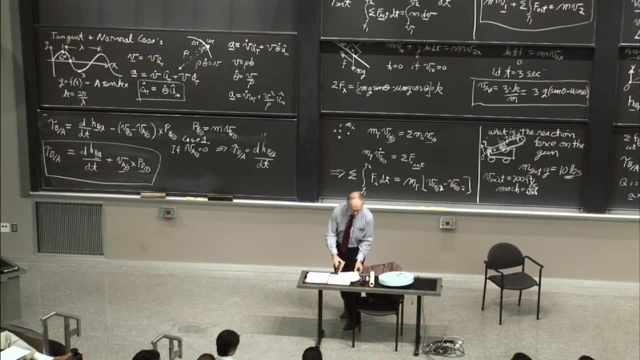 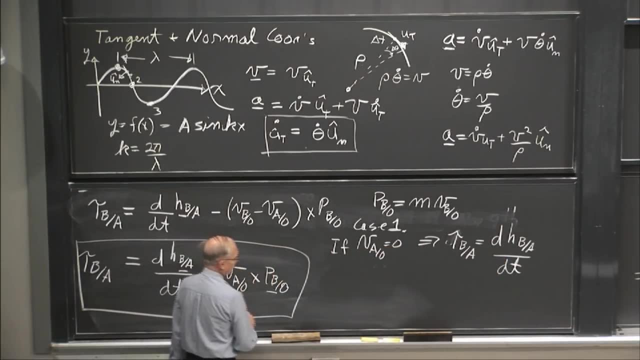 is not moving, then you don't have to deal with that messy term. So this is one case in which this term goes away. The other case This is if this velocity is parallel to the direction of the momentum, And there's a really useful time that that happens. 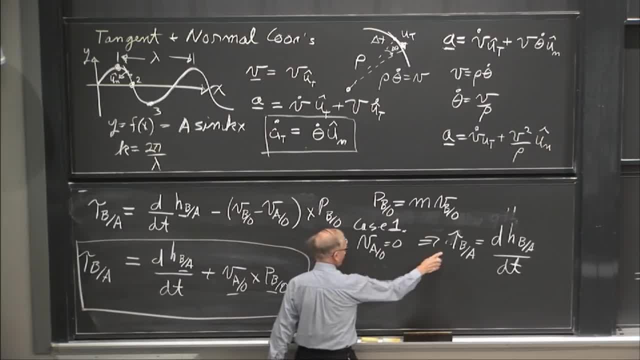 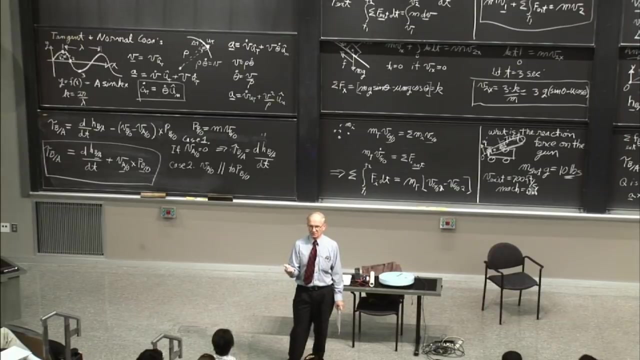 So also this formula is true. Case two is when VAO is parallel to PBO, the direction They're going in the same direction. Now that happens when A is guaranteed to be true, if A is at the center of mass. 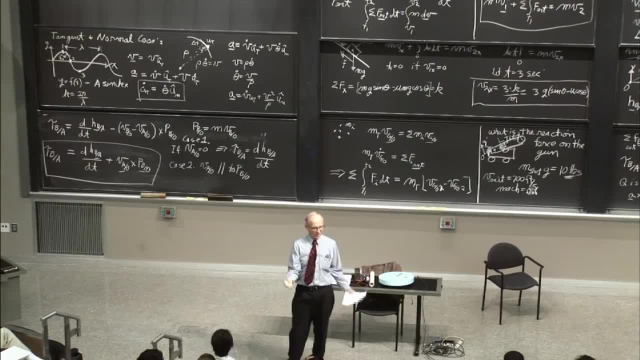 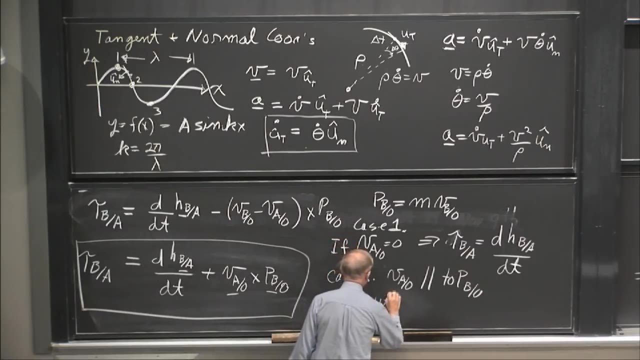 Because a momentum is defined as the mass of the object times the velocity of its center of mass, even for rigid bodies. So this is true when A is at the center of mass. So the momentum is defined as PBO, And so this is true when A is at the center of mass. 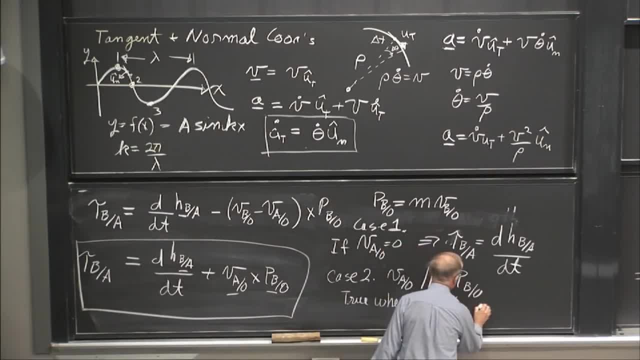 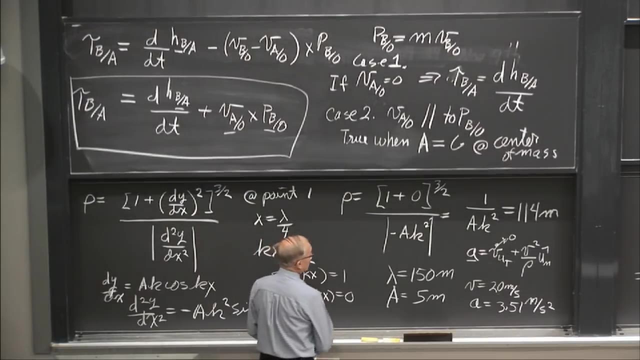 even for rigid bodies. So that's the answer. OK, Thank you so much for your time. Bye, Bye, Bye, Bye, Bye, and I'll call it g at the center of mass. So this gives us another really important generalization. 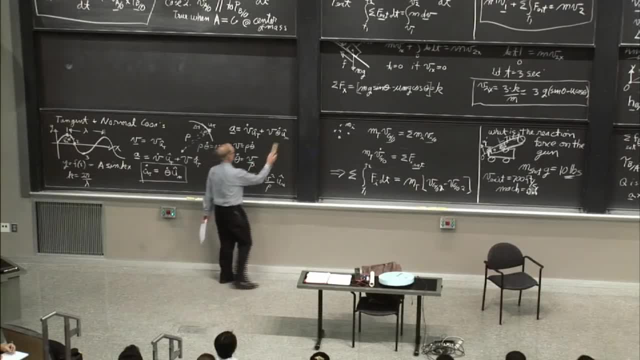 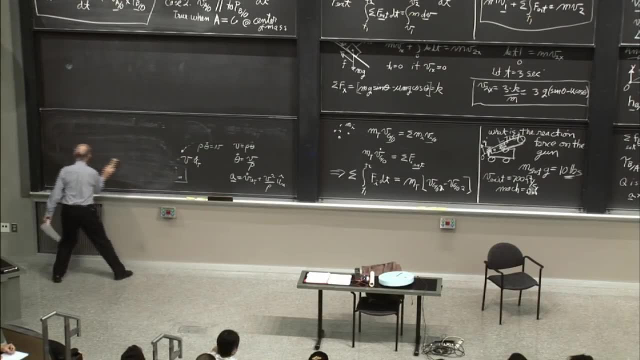 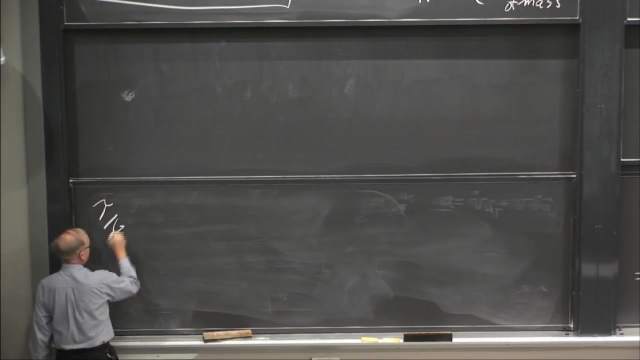 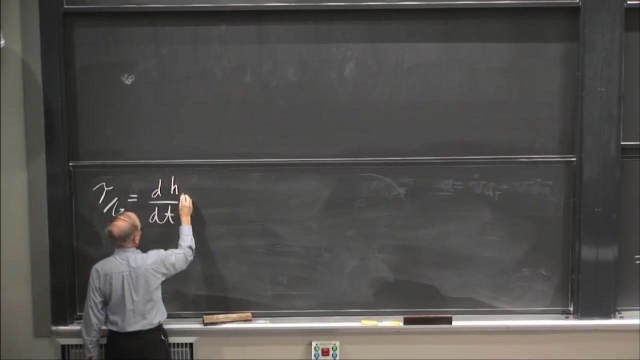 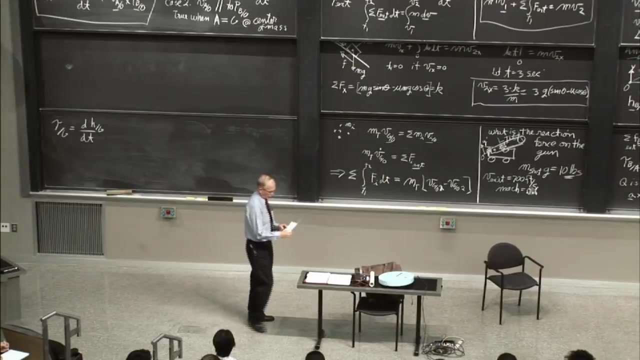 that we make great use of in dynamics And that says that the torque with respect to the center of mass is time rate of change of h with respect to g. Now I'm not going to go. I did the proof, went through this. 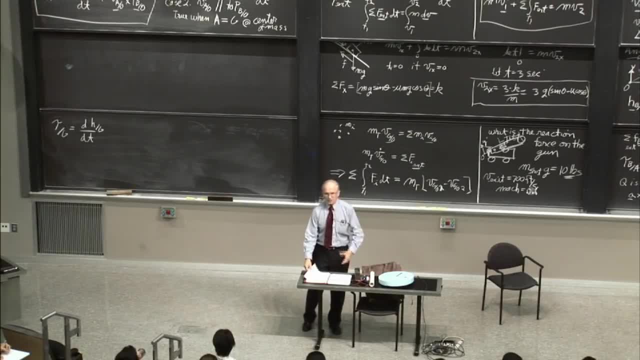 I did this little proof just for a particle, But by summing a bunch of particles and kind of going through all the summations as we did to prove the center of mass formula you can show. this allows you to very quickly show that this formulation is also true for rigid bodies. 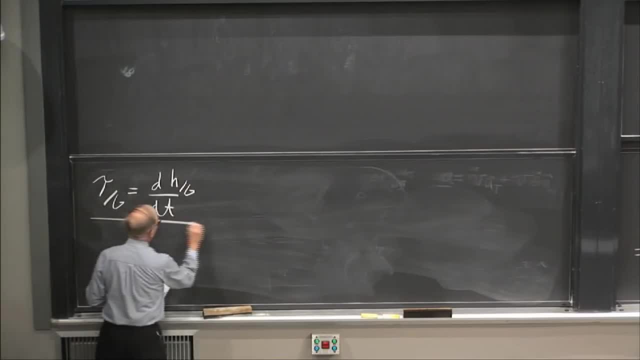 So the way you say it for rigid bodies is that the sum of the torques about with respect to some point for a rigid body is H dot with respect to A, plus the velocity of A with respect to O cross p. And now I'm going to say: 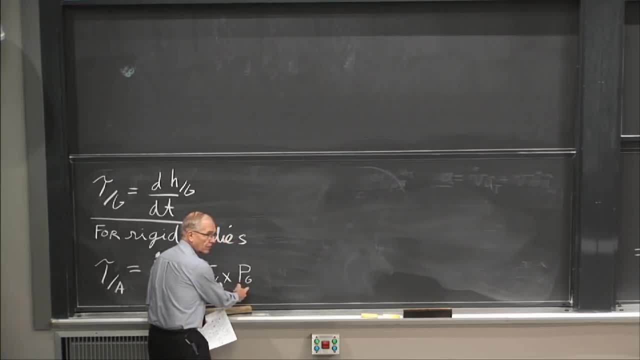 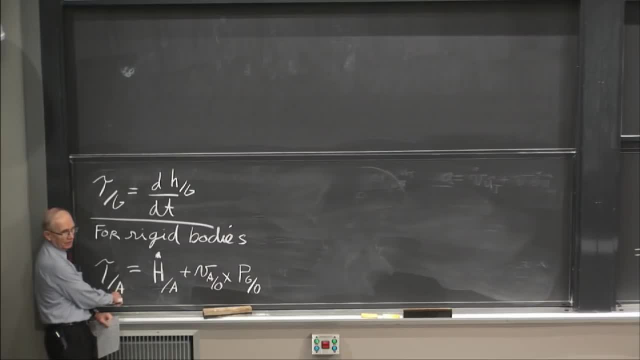 which can be moving now, even accelerating, is the time rate of change of the angular momentum with respect to a of that rigid body, plus vao, cross, pgo. And again, when would this messy second term go to 0?? When the velocity of a is 0, fixed axis rotation. 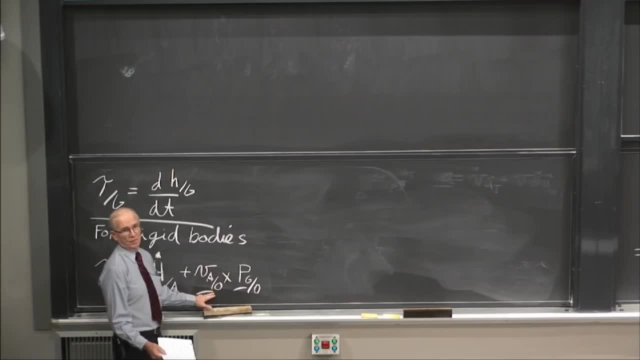 Or when this is parallel to that which is true for the center of mass. always. So the same two special cases apply for rigid bodies: when velocity of a with respect to o equals 0. Or when When the velocity of a with respect to o. 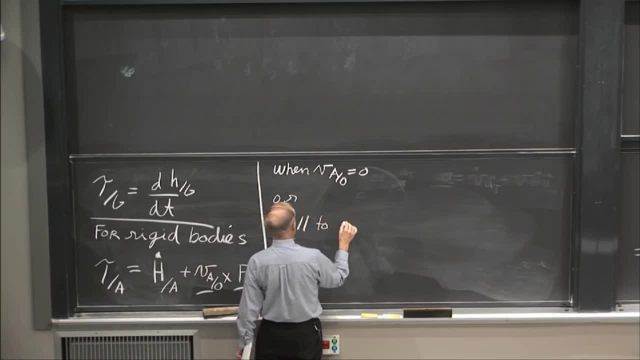 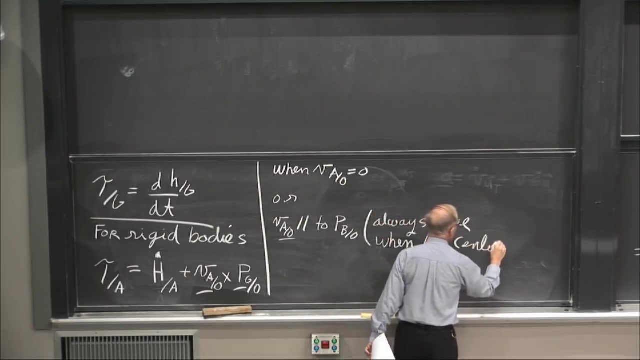 is parallel to the p and the most important case of that is always true, That's always the case, And in these one you can say this: then the torque, with respect to a, is dh. with respect to adt, No second terms. 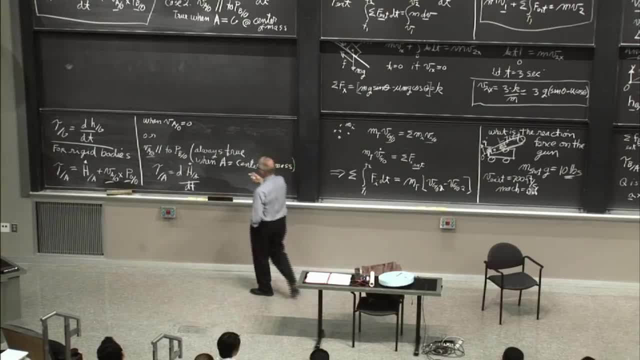 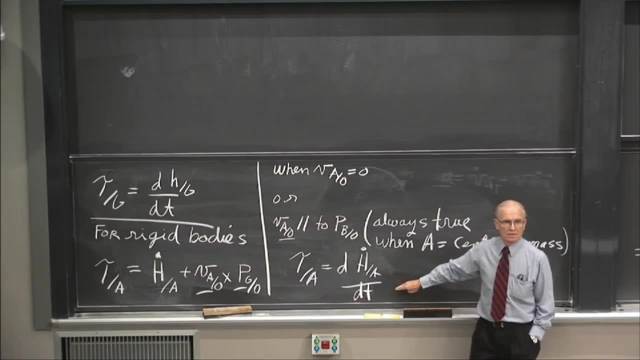 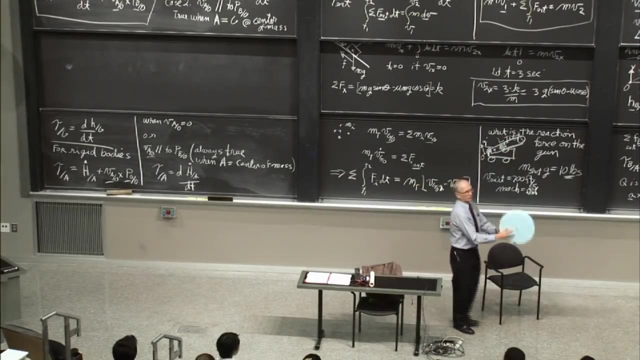 And it's those kinds of you've applied generally in your physics, like in 801, you've used formulas like this a lot. You've done problems either with respect to the center of mass, So objects doing things like that. You'll do the torque formulas with respect. 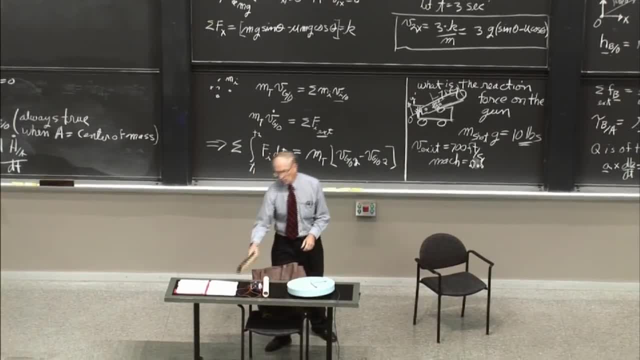 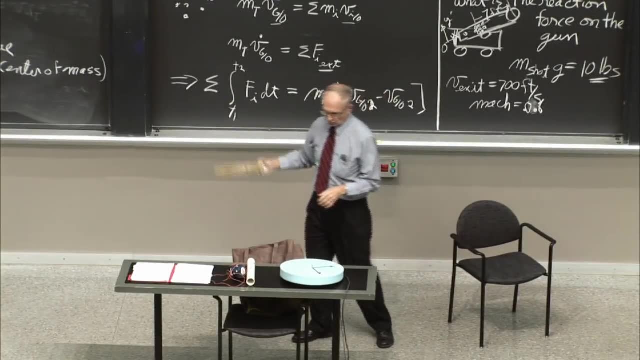 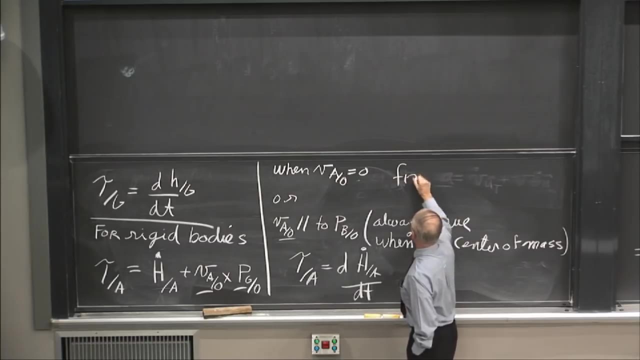 to the center of mass, Or when you have things that are pinned to points and rotate about fixed axes, then you use the other formulation where it's with respect to a non-moving Point. So this is fixed axis rotation. OK, All right. 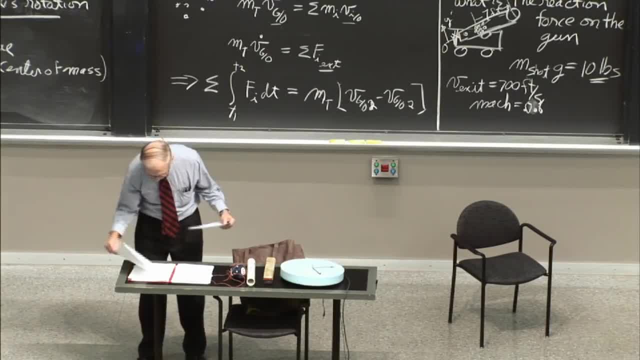 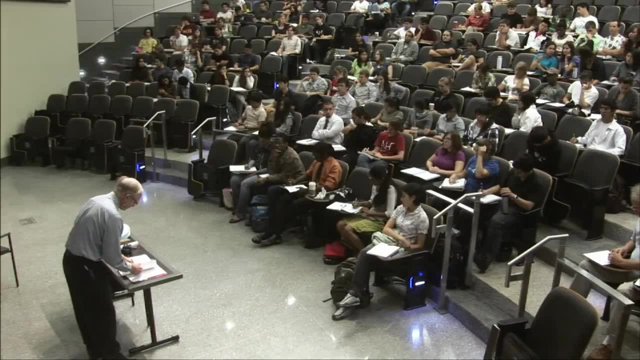 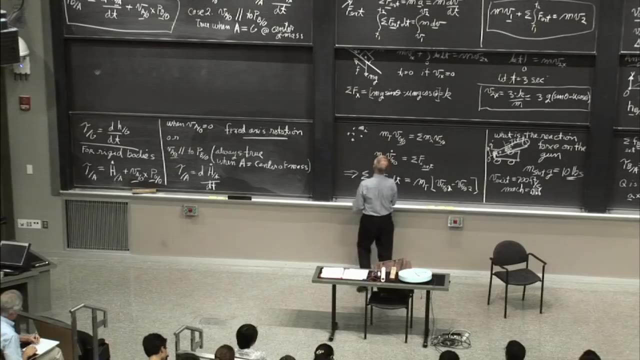 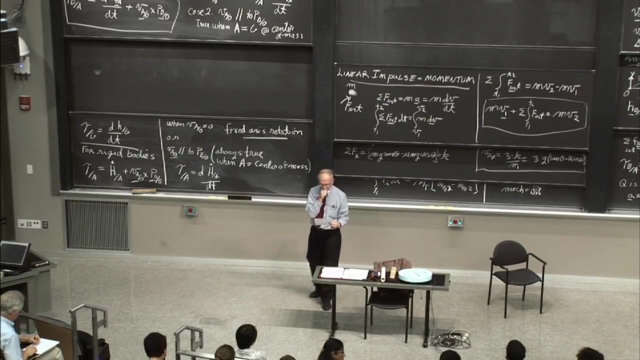 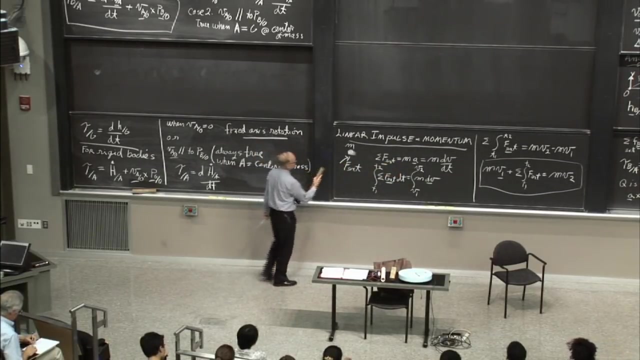 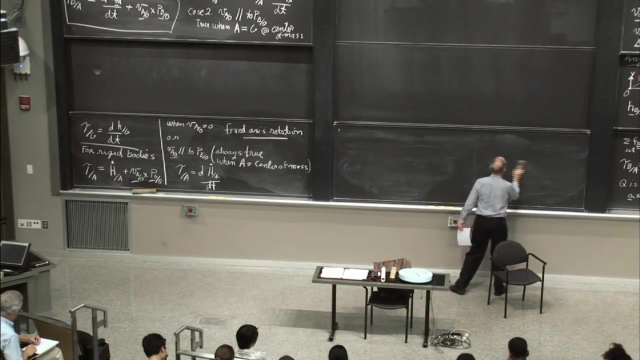 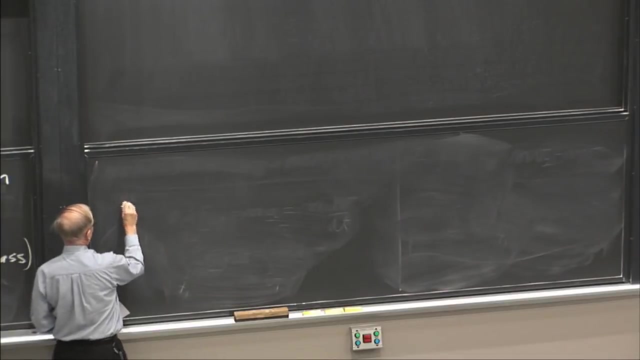 So that's kind of the dry derivation part of it. I'm going to see if I can find an example here. OK, This is quite a bit like a number of the homework problems. So I've got a carnival ride, Got a bar. 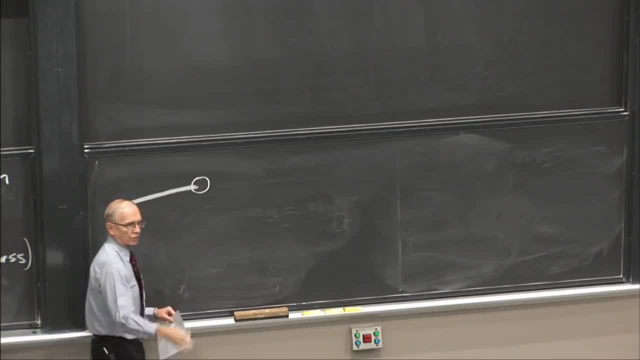 And it's got a seat out here. You're riding in it, All right. So you're taking this ride. It's rotating. This is some fixed axis here And you have a fixed coordinate system: your O, x, y, z. 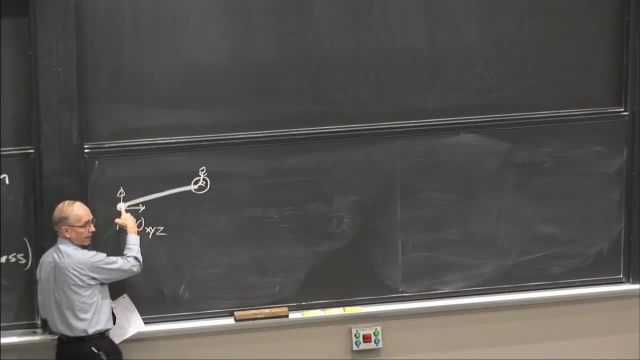 And then you'd probably have some rotating coordinate system with the point A fixed here at the axis of rotation. And what's unusual about this ride? not only can it go up, but it can go down. It can go up, It can go down. 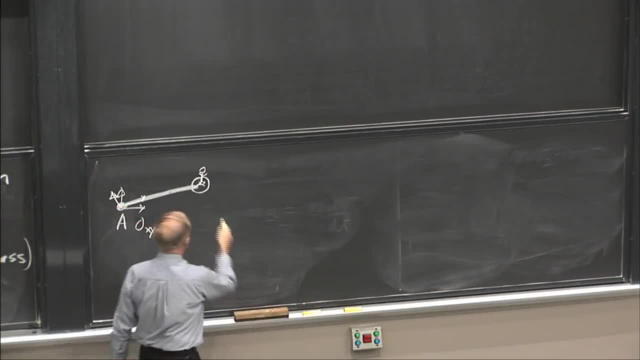 Not only can it go around and around, but the arm can go in and out, So it might take a path inwards. Like if you pull the arm in as you're going around, what are the forces that you feel in the ride? 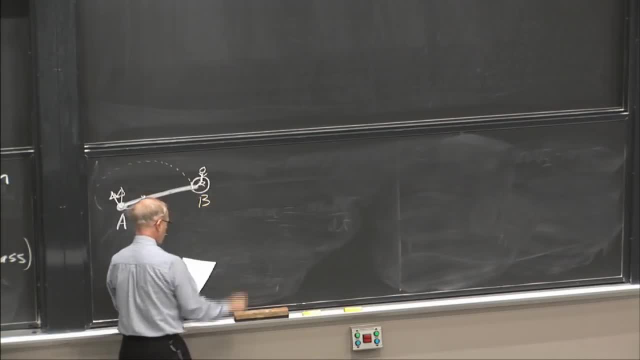 So this is my point B out here. It's where the person's at Have some mass m And let's let this go. OK, All right, Let's let for now. first case: theta dot. Let that be constant. 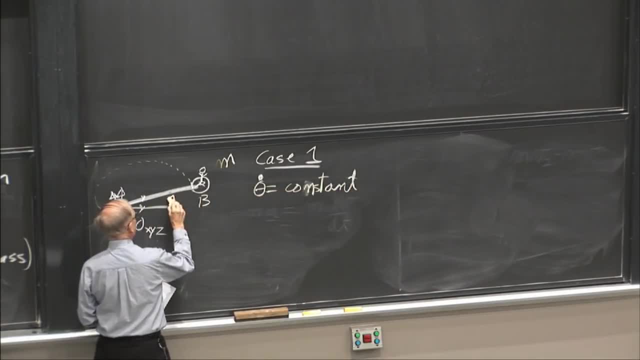 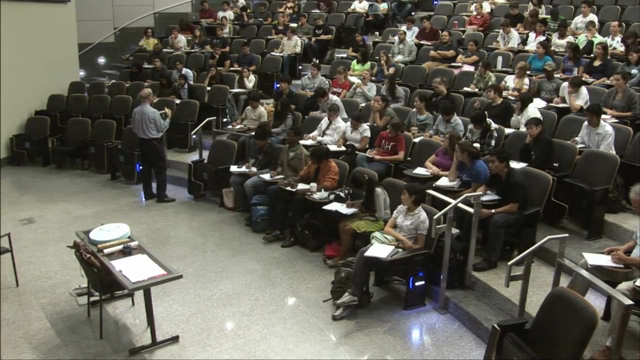 Constant angular rate here. Here's theta And r dot. All right Now you already know quite a bit about things like this. What forces, if you're riding in that bucket, what forces do you think you would feel? Or I should say it more carefully there: 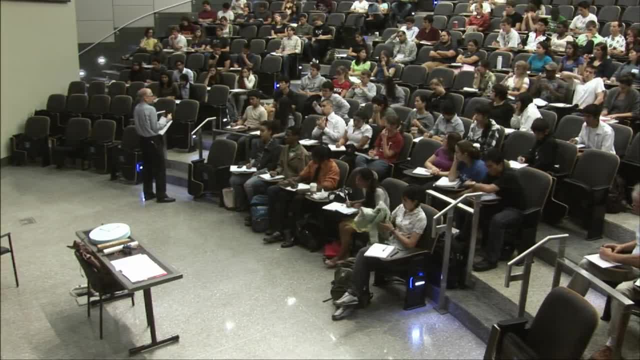 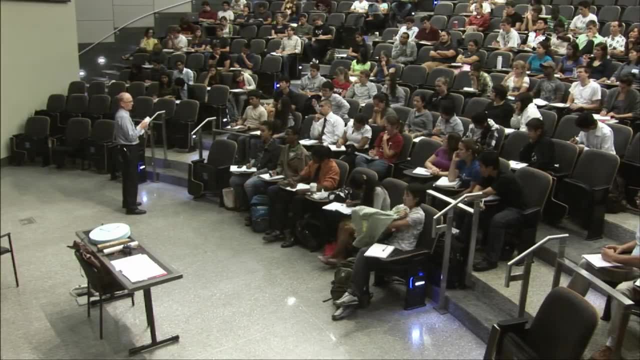 will be accelerations that you feel in that bucket. You'll feel like forces on you. But what are the accelerations that you will feel you expect to be if you're riding in it? I hear one here: Centripetal acceleration. 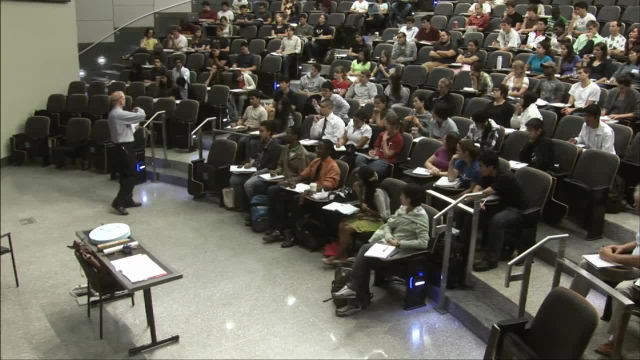 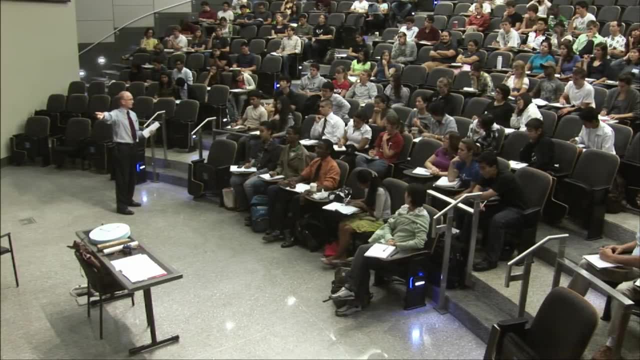 So there'll be centripetal acceleration, right, Everybody agree with that. Anything else, Coriolis acceleration. There's going to be some coriolis, because r dot is not 0,. right, It's changing in position, But when the length of the arm of something rotating, 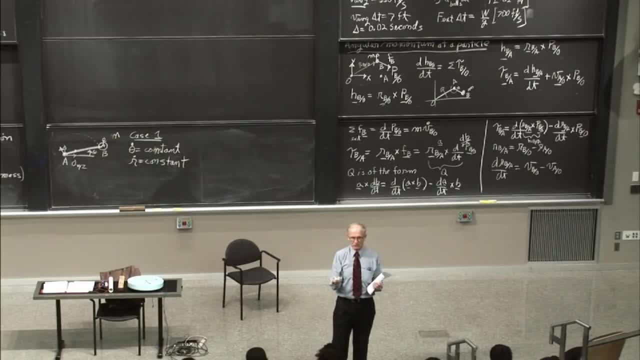 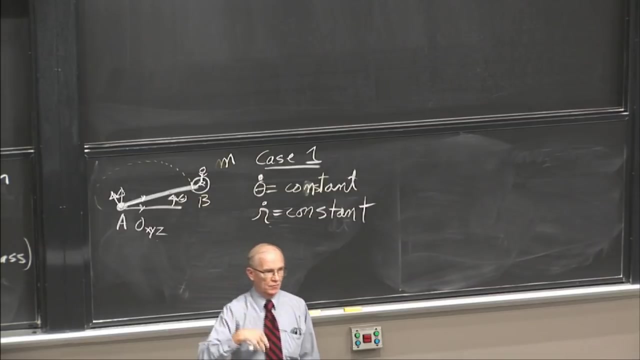 at constant speed changes. what momentum changes? Angular, for sure. How about linear momentum? Yeah, it's changing too, because r cross p is angular momentum. So both linear and angular momentum are changing as this radius gets longer or shorter. And if that angular momentum changes, 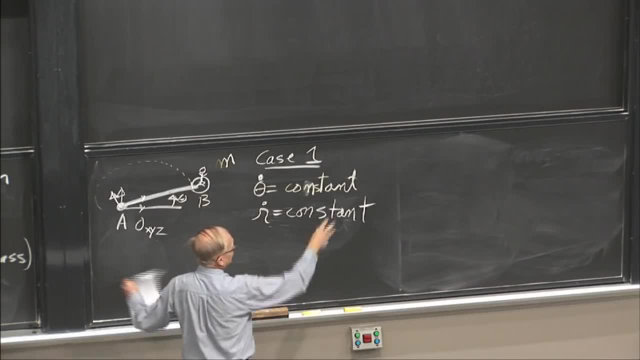 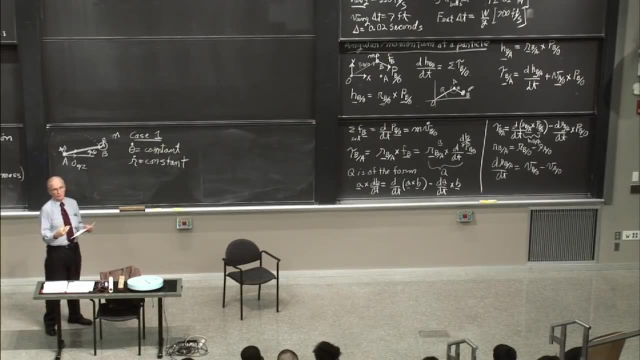 it takes torque to drive it, And so we ought to be able to use the formulas that we've just derived to calculate something about the torques required to make this happen and the forces on the rider. OK, So we'll treat this one as a particle. 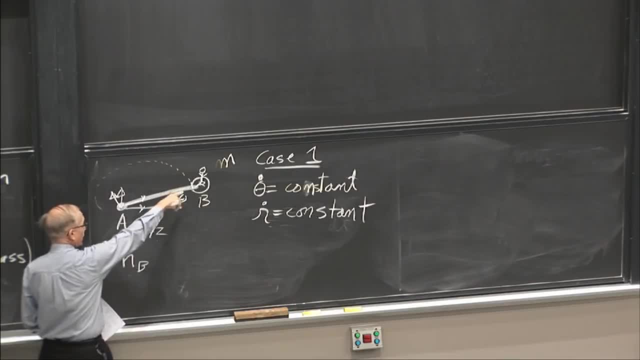 So h. the angular momentum of the rider out here at b with respect to o is going to be rvo cross p, And in this problem I'll use p Polar coordinates. pretty easy, This is a planar motion problem. 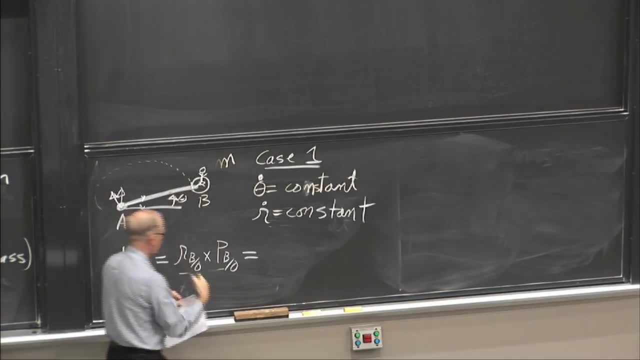 It's confined to the xy plane and rotation in z, So polar coordinates are pretty convenient. So this should look like radius r r hat cross And the linear momentum of this is the mass times r dot r hat. That's the extension rate. 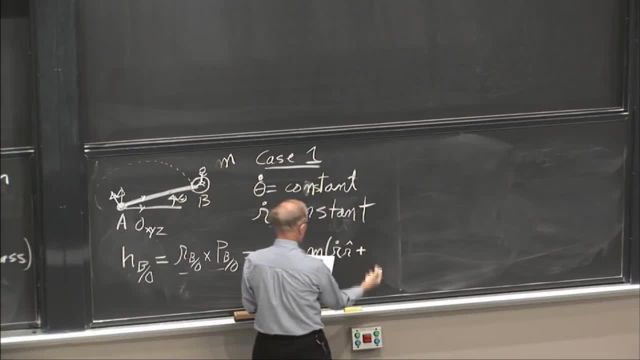 But it also has velocity in the theta hat direction: r theta hat. So this is p with respect to o mv And this is the r crossed into it. Now, r hat cross, r hat gives you 0.. So you only get a single term out of this. 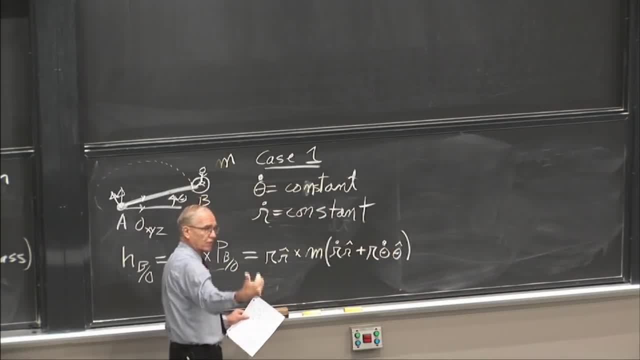 And you get an r hat cross theta hat, A positive k. So this looks like: plus m r squared theta dot k hat. That's my hbo. Now, that's my first piece that I wanted to get. That's the a part. 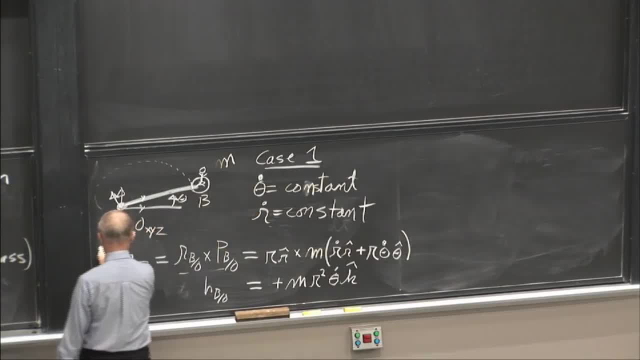 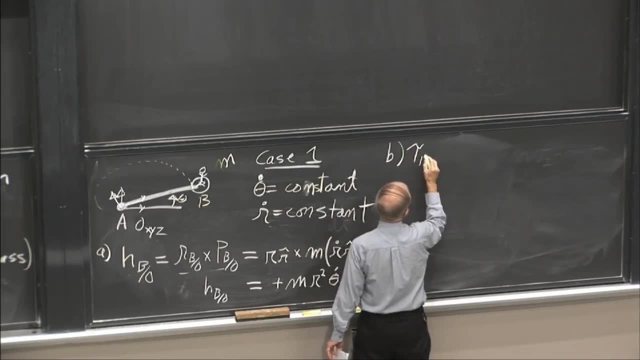 That's find the angular momentum. So this is a, b. I want to know the torque. Well, which formula can we use? Are we allowed to use? do we have to account for that second term? No, why? Yeah, the velocity of the point about which. 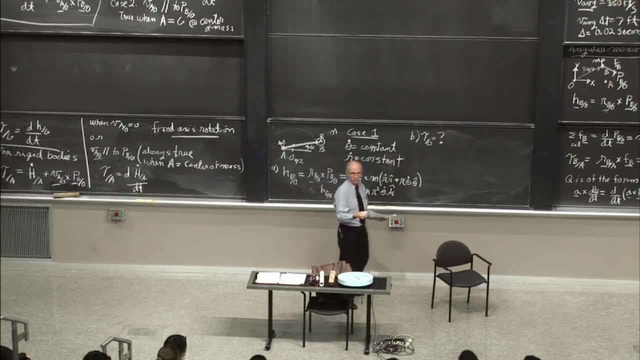 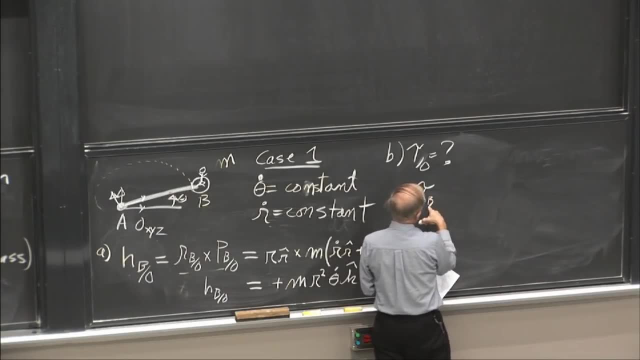 we're computing the angular momentum And therefore the torque is not moving. So you only have to deal with the first term. So the torque required to move that particle at b with respect to o is just the time rated. change d by dt of h. 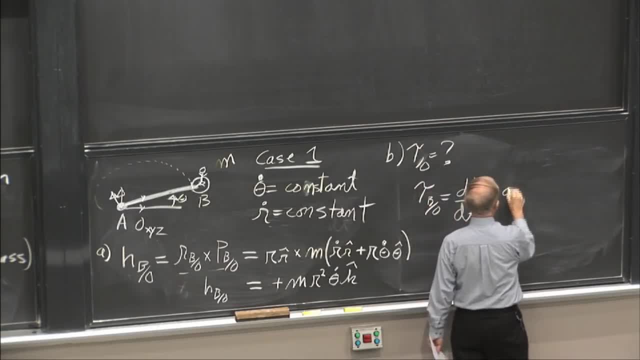 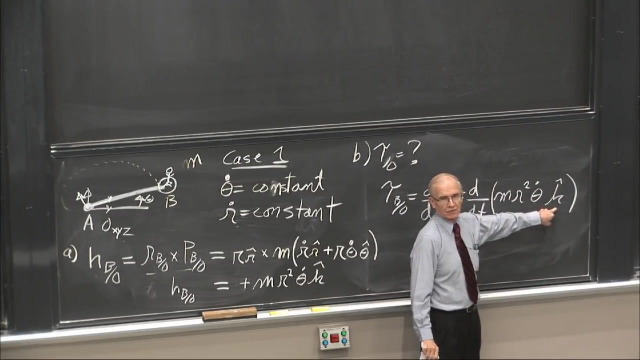 B with respect to o And that's d by dt of mr squared. Yeah, theta dot k hat. So what are the constants in this expression? so we don't have to worry about their derivatives? Does k hat change length? No, 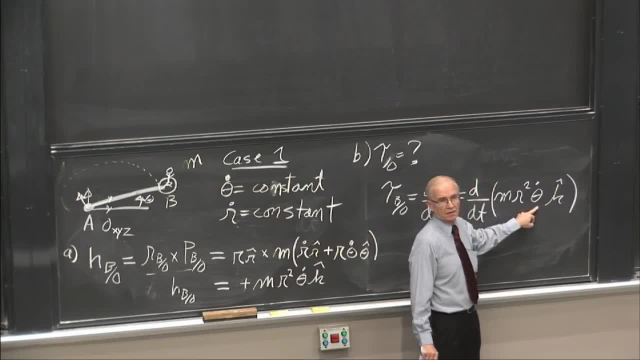 Change direction? No, Theta dot does it change in this problem? No, we fixed it. We said it arbitrarily, started off saying that we'll just let theta dot be constant. r, though, is changing, So the time derivative of this particular one. 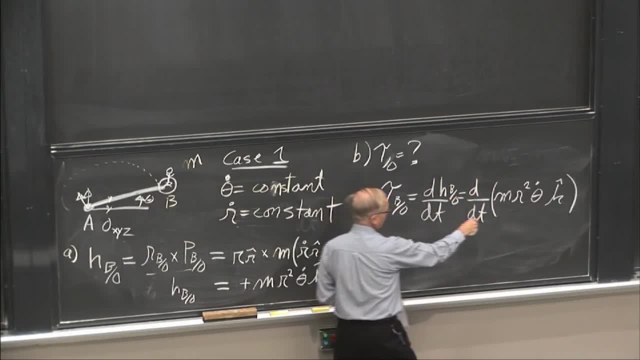 we only have to deal with the r. Actually, I'll forget that for a second. So I want to get both terms and then we'll let it be a 0. So this time derivative. then when you work it out, The derivative of the r term gives you 2mr r dot, theta dot. 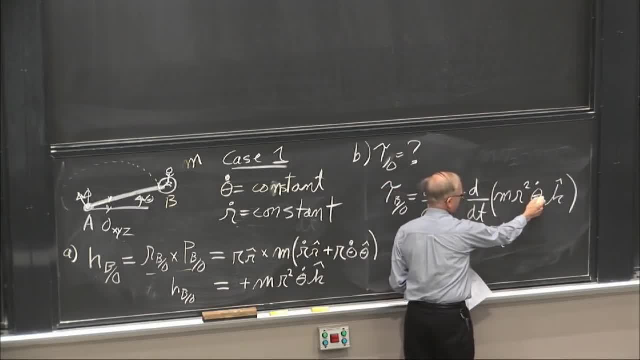 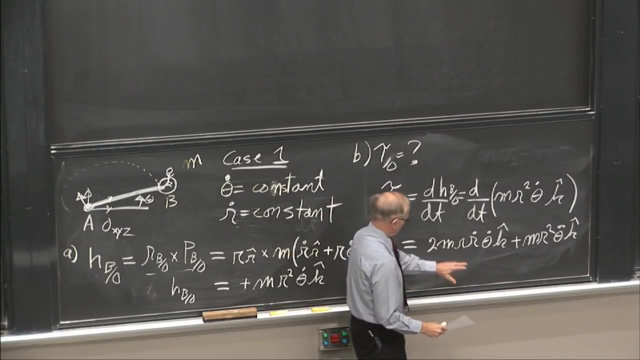 k hat, And I'll just go ahead and forget for a minute that I said that's constant. Let's get the other term that might be there. That term gives us m r squared theta double dot k hat. This term comes from what we'll find is the Coriolis one. 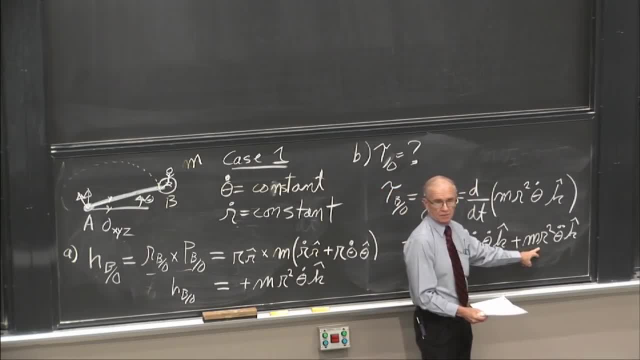 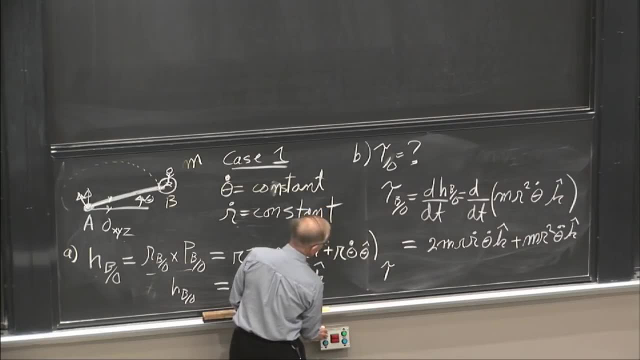 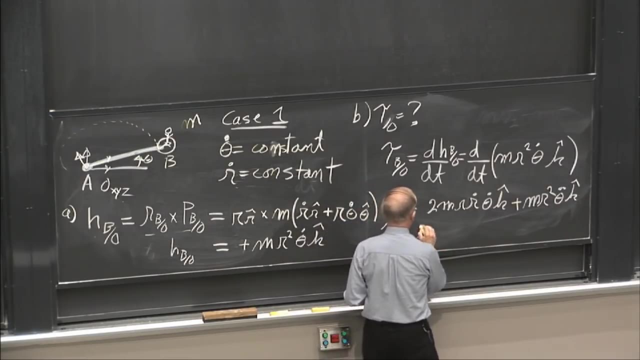 And this is from what we'd call the Eulerian acceleration. This torque must the torque. let me get this up a little higher. We should be able to write as some r cross f Right, And so the r cross f terms. this will be from the Coriolis. 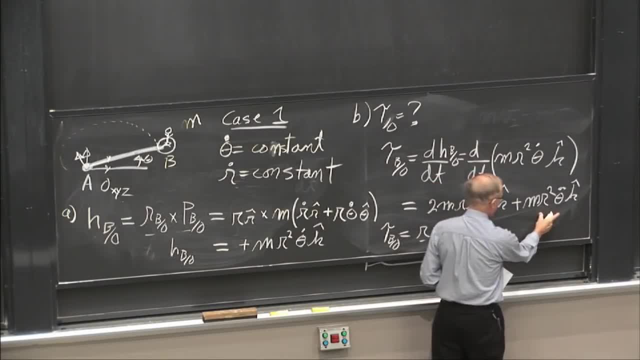 force and this would be from that Eulerian force, So this will look like r r hat cross. OK, OK, OK, OK, OK, I'm just factoring this back out into its cross products: r r hat cross, 2m r dot. theta dot in the theta hat direction. 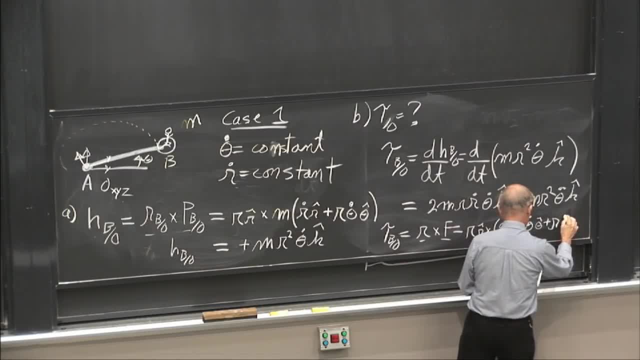 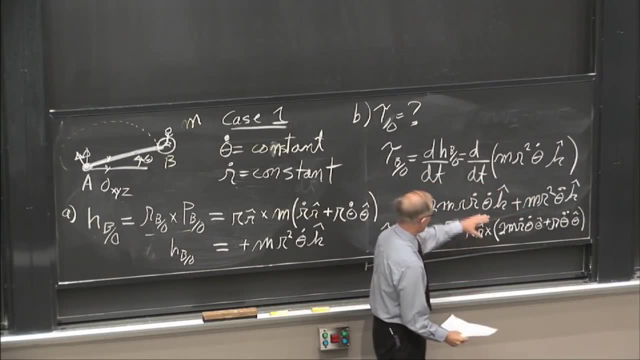 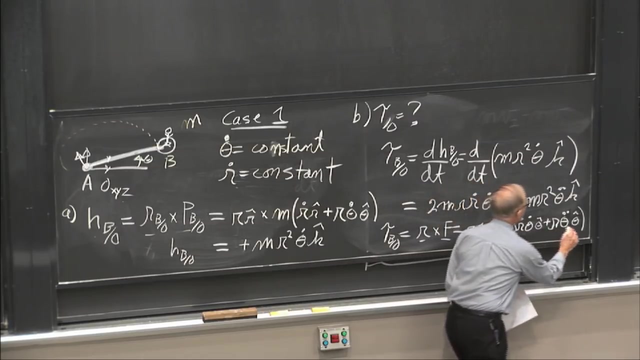 plus r theta, double dot in the theta hat direction. So there's two terms in this torque expression. They come from r cross two force terms. The first force term is what we know to be the Coriolis force And the second force term- I'm missing an m here. 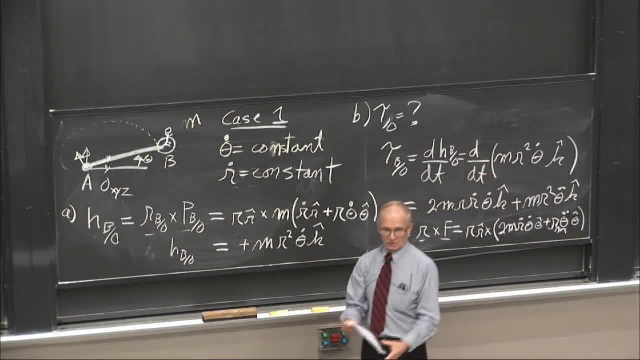 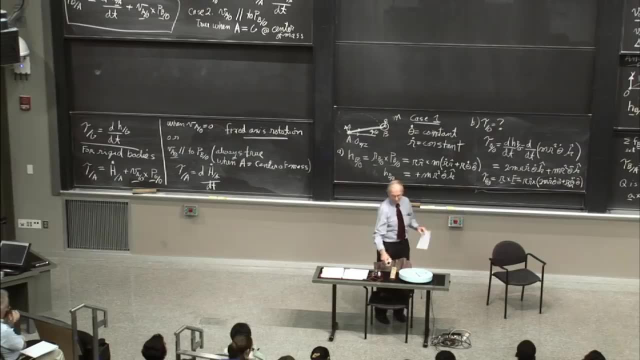 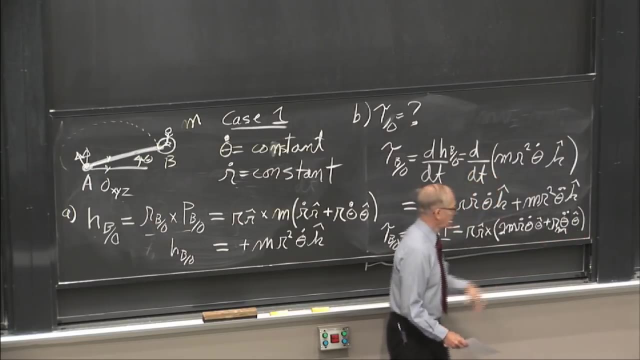 rm theta double dot theta hat. That's the force that it takes to. if the thing we're accelerating, just to accelerate that ball, theta double dot takes a force, You do these cross products. r cross theta hat gives you k. r cross theta hat gives you k. 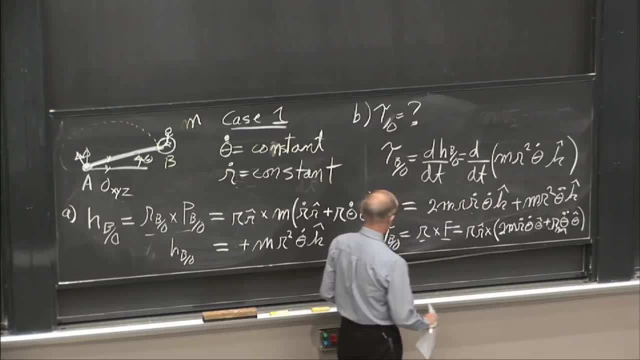 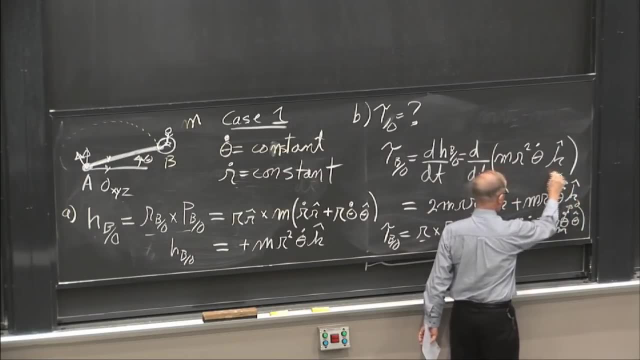 It all comes out in the right directions. And now to do the problem we had. we said, oh yeah, but this one's 0. So we'll let this term go to 0. We're left with a single term. 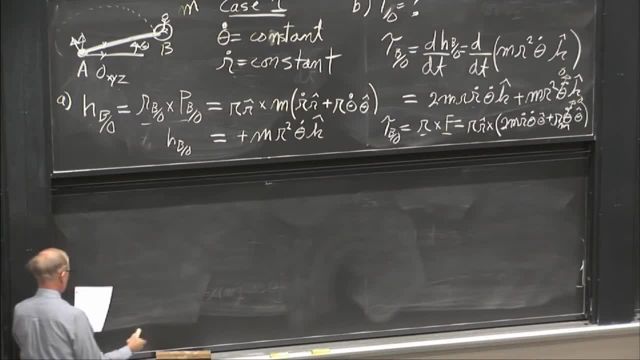 And it represents a derivative of 17 minutes. But we don't know what the value of 0 is. So you see, this is some new work. You see what is left now. This is a double: the 0 and 1.. 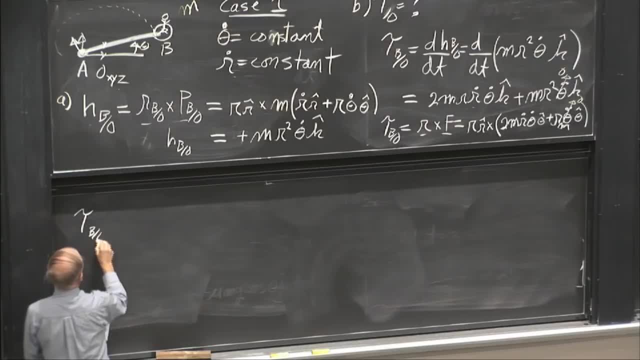 It looks like it's a lower number than the自, along which we said 한� theirs. But now, if it was 0 or 0, we'd be using beta these two, the two there, and we'd be choosing our. 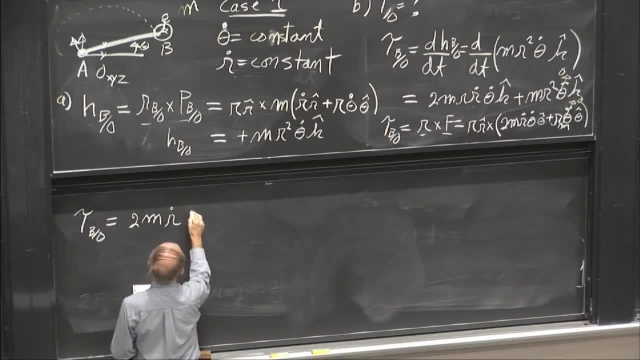 So, as we humans have tried to determine the value, this is the value that I get. So here's the difference: 0.7xxx.2xx.1. discovers that 06, Netherlands walks through these terms: 1,2,, 15,, 1,6,, 6, when we scored 116.1,. you see, this is 0,, 5 times zero, 7, ?35.2,4,2,3 e. 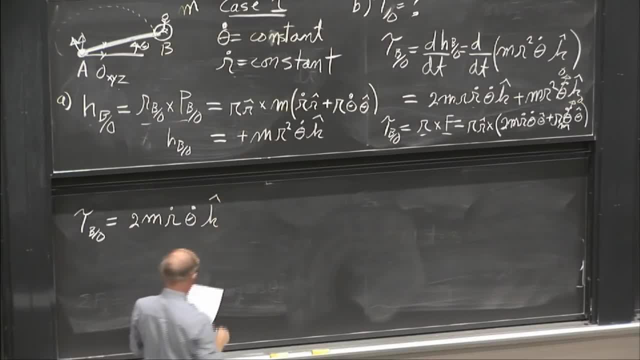 And if we plugged in some numbers, let's just see how this works out. And this we know is just r cross the Coriolis. Well, let's let m be 100 kilograms And r be 5 meters and r dot 0.4 meters per second. 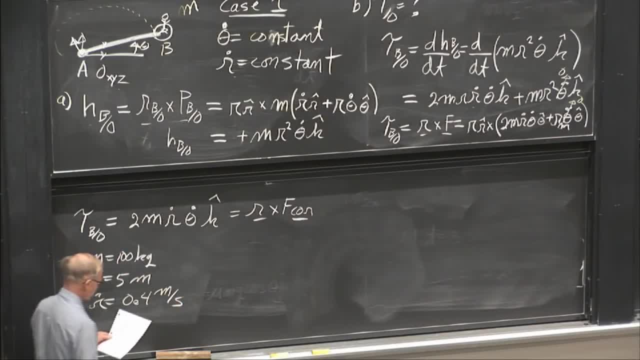 All kind of perfectly reasonable dimensions. And theta dot equals 3 radians per second, So 2 pi radians per second means it goes around once a second Right A little less than half a rev per second. Yeah, Is there supposed to be another r there? 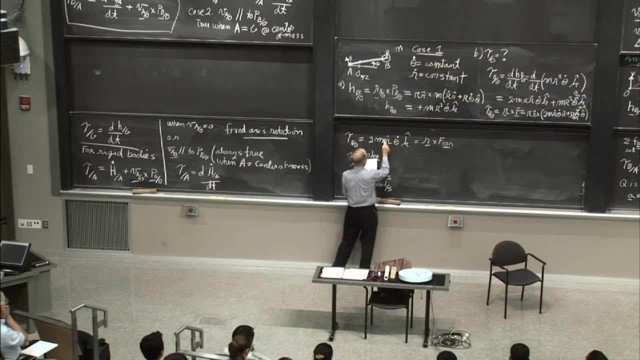 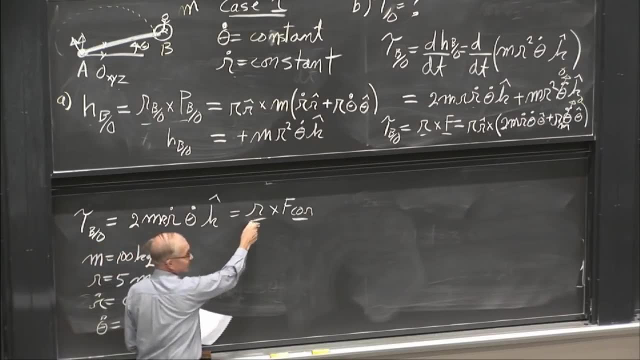 Probably. Yeah, Good catch, Got to have an r in it, because that r comes from here, right. So I had the Coriolis force written down, but not the r. you have to multiply it by. So now, if you plug in all of these numbers, 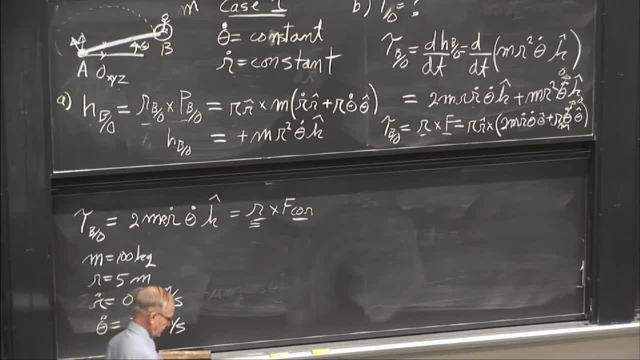 let's see if it's a ride you could survive. I actually computed the Coriolis force first. I think it's just interesting to get a physical feeling for whether or not you can feel these forces. So the Coriolis force is just everything but the r. 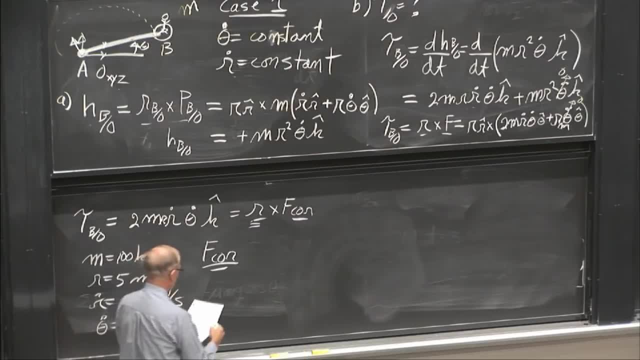 2m r dot, theta dot. So if you calculate that you get 240 newtons And r times that the torque, 5 times that, about 1,200 newton-meters, And the acceleration, how do we get acceleration? 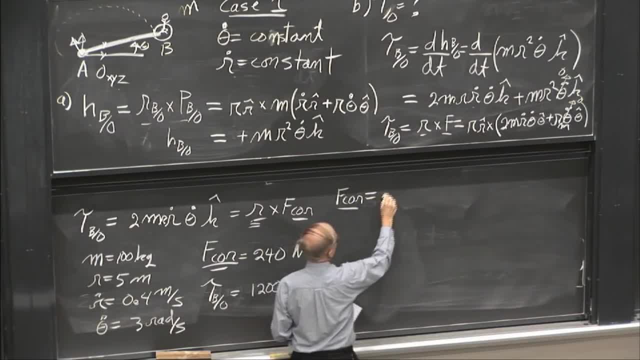 Well, F core Coriolis force is some mass times an acceleration. So we can solve from that 240 newtons the acceleration right Now. this is an acceleration of B with respect to O: 240 newtons divided by 100 kilograms. 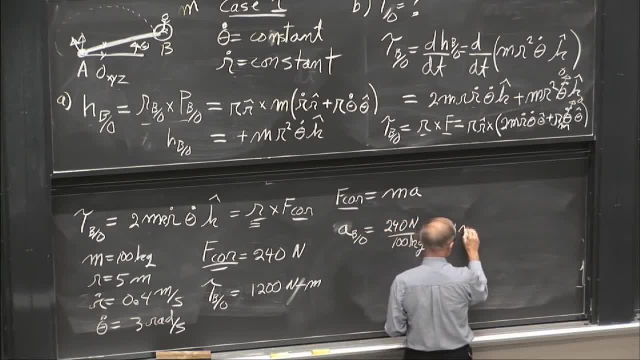 2.4 meters per second squared. And what's that in g's? About 1 quarter, Yeah, about a quarter of a g. And again, would you feel that? So now you're riding in the bucket, right? Let's say it's just spinning around. 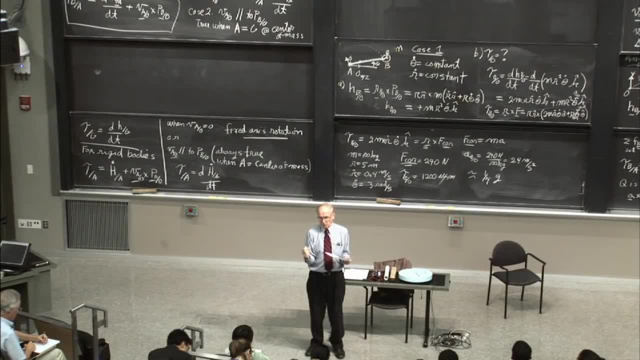 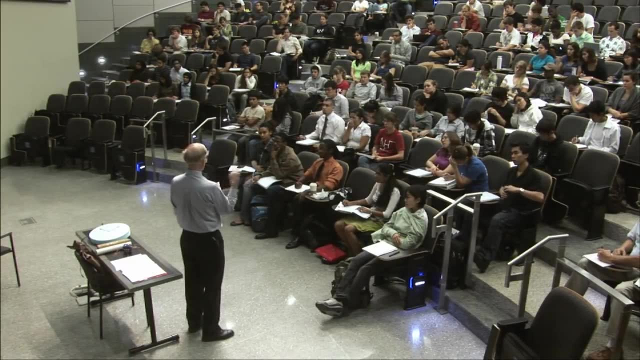 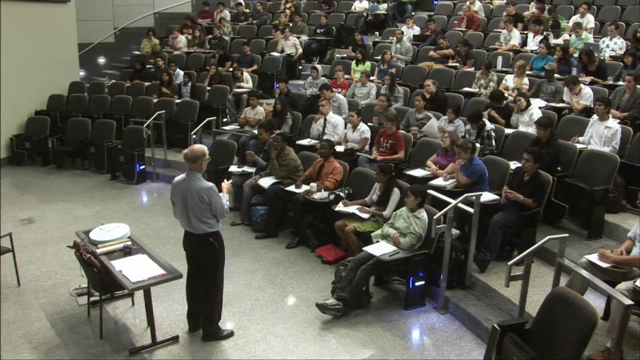 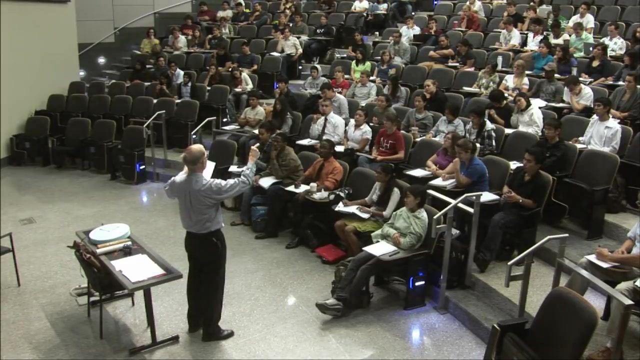 The arm's not going in and out at all, So you're riding in it. What force would you feel? Would you feel any forces pushing you into your seat? Constant speed: r dot 0.. Somebody out there? Would you feel any force if you're going around and around? 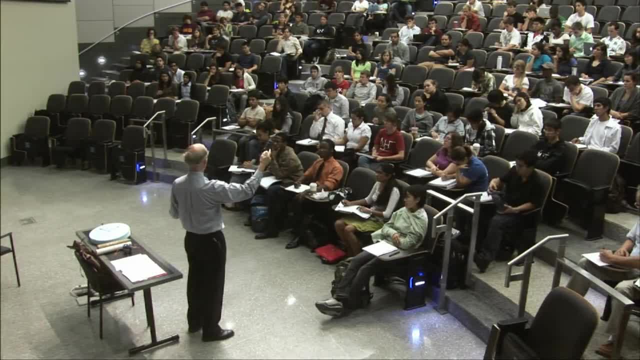 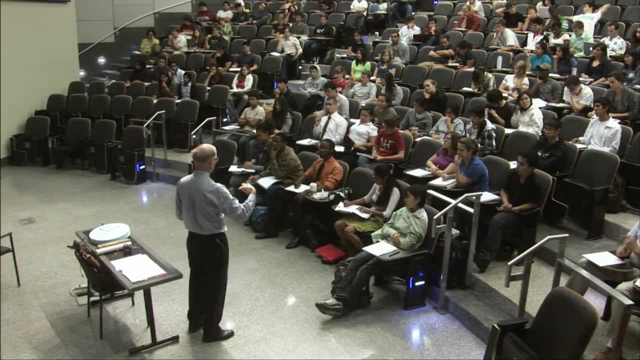 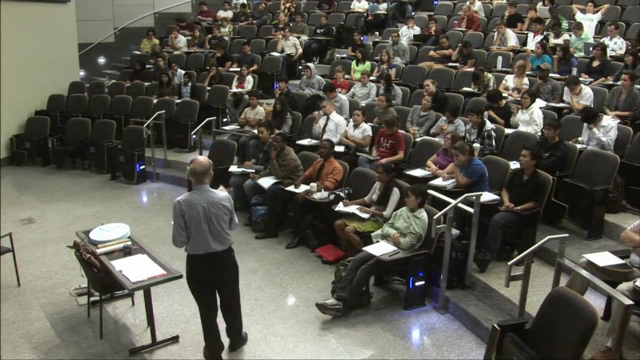 in this thing sitting in the seat. OK, what's it come from? Centripetal acceleration, right, All right. So, and that is in what direction? Acceleration is inward. What would you actually feel? You'd feel if this seat could swing out? so you're facing in. 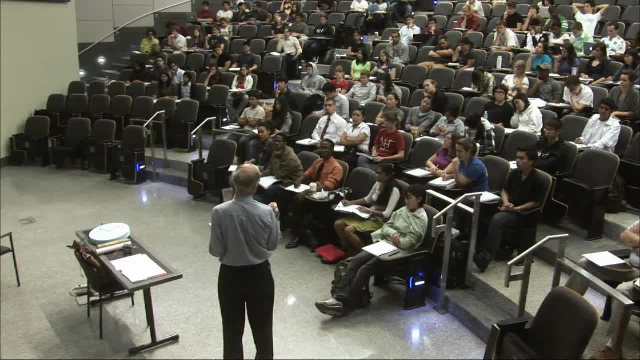 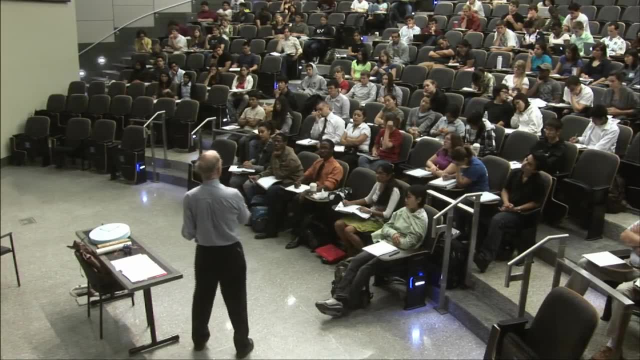 you'd feel like you're being thrown out in your seat, right Yeah, Because you have to have a force on you to make that acceleration happen. The acceleration is inward. The force had better be pushing you inward, So it's pushing on your back if you're looking in. 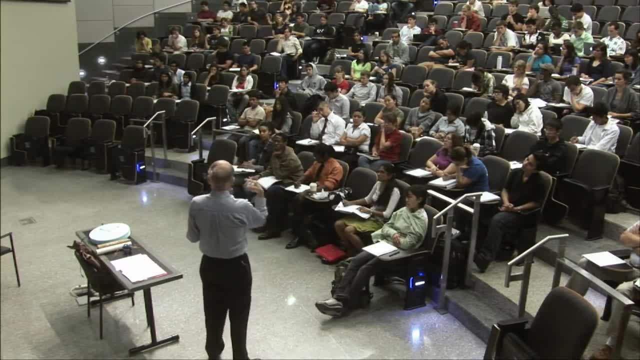 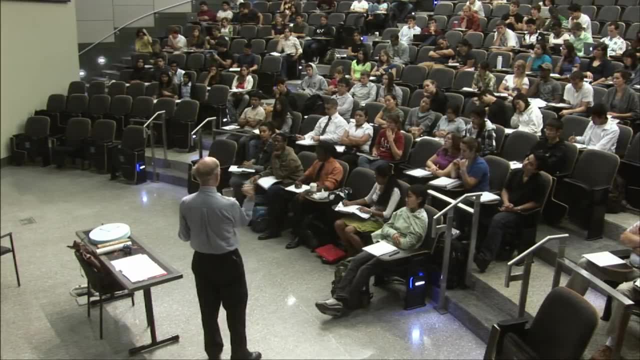 going around. So that's the, you know the. I've forgotten the term for them, But you know they put the astronauts in a centrifuge right, Spin them around to see if they can take high g's. OK, that's the g, the inward high g acceleration. 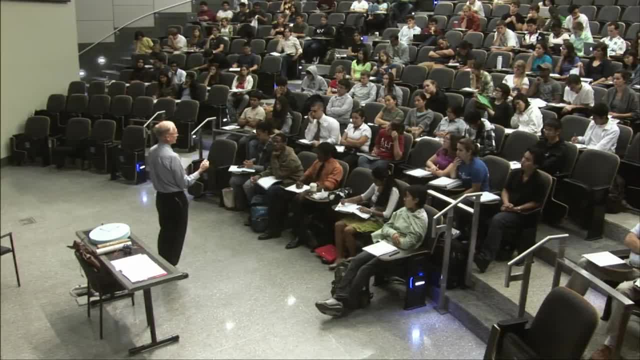 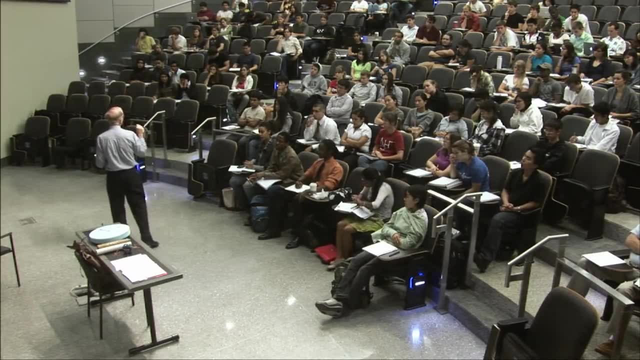 That's the acceleration due to the centripetal acceleration, making you going in a circle. But now, not only are you going to feel that, but now you start changing the length of the arm And if you change r dot and make it positive, 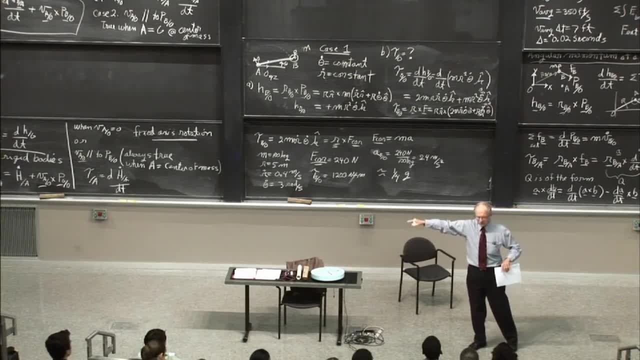 so the arm is getting longer And we made this 0.4 meters per second. So it's moving out. you know about like that. It's not real fast, But it's going to create a quarter of a g acceleration on you. 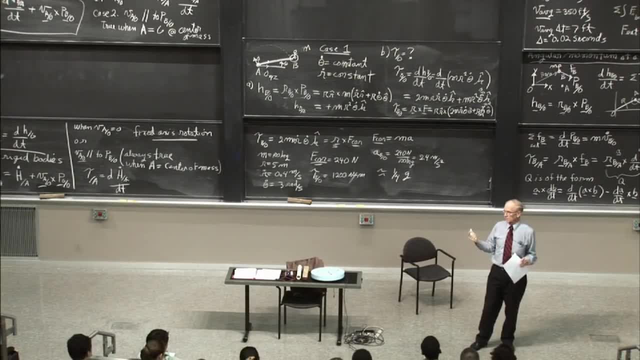 And if r dot's positive, which direction is that acceleration? I was careful when we walked all the way through this. The acceleration is positive, but in what direction? For Coriolis, Theta hat, Positive theta hat. So it's in the direction of increasing theta. 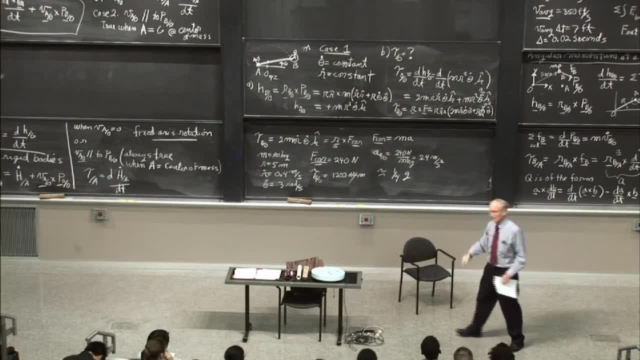 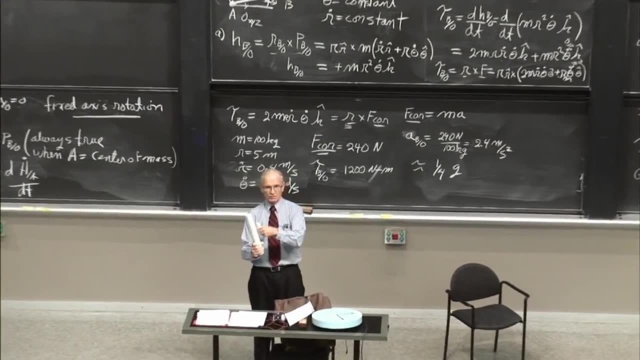 So this one is perpendicular to the arm right And this is the, you know, one of my ping pong ball in here. The force that actually causes it to speed up is partly Coriolis and partly Euler, And if I could make this go at constant.